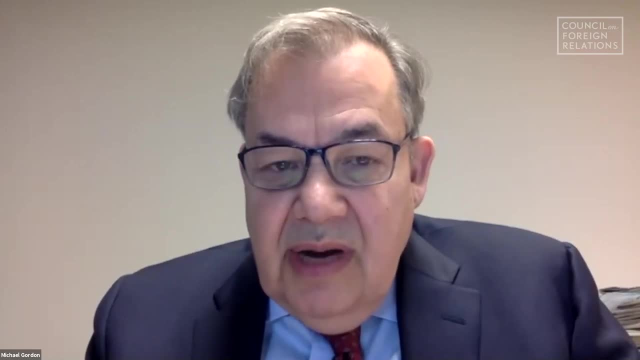 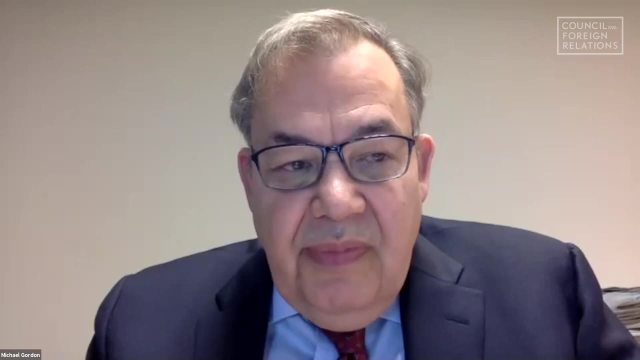 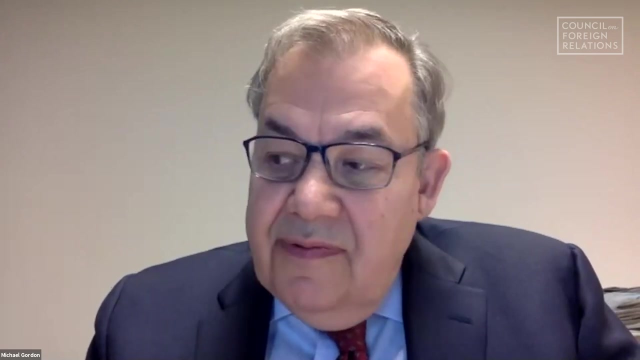 in the last half for a Q&A and there's a procedure for raising your hands and asking questions. As you know from the materials in front of you, the people who are going to be speaking today, it's a strong panel of Robert Einhorn, who's a senior fellow at the Working's Institution. 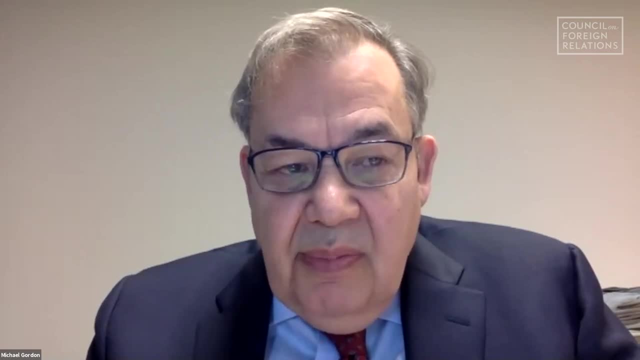 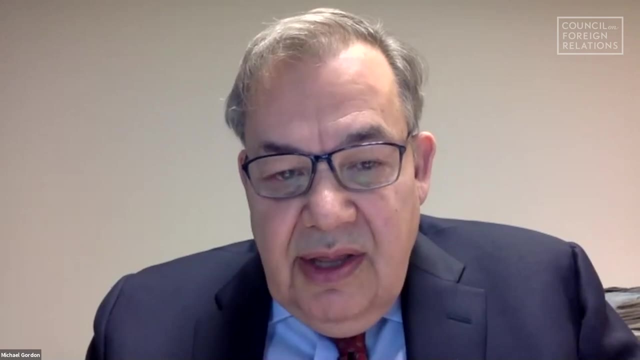 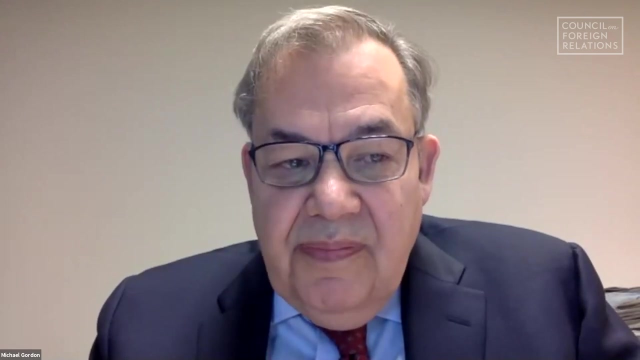 who's a senior official at the State Department on nonproliferation issues, a very experienced person in these areas with a lot of, I think, nuanced and original views. Lisa Gordon-Haggerty, a former administrator of the National Nuclear Security Administration. Laura Holgate, who. 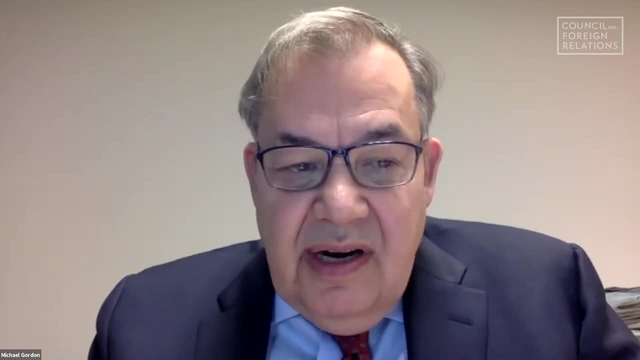 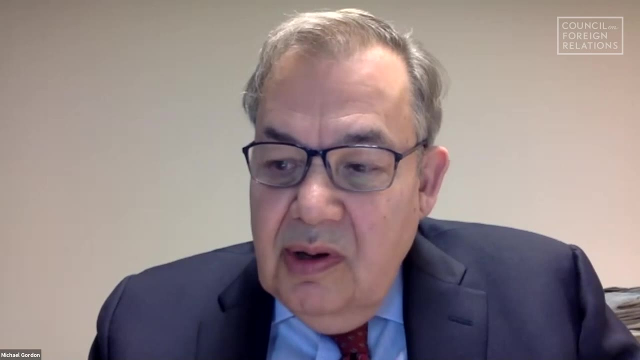 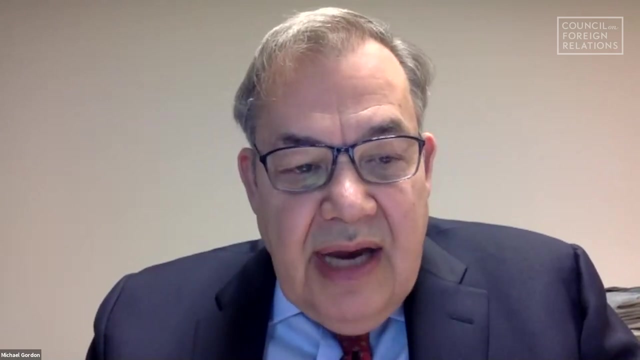 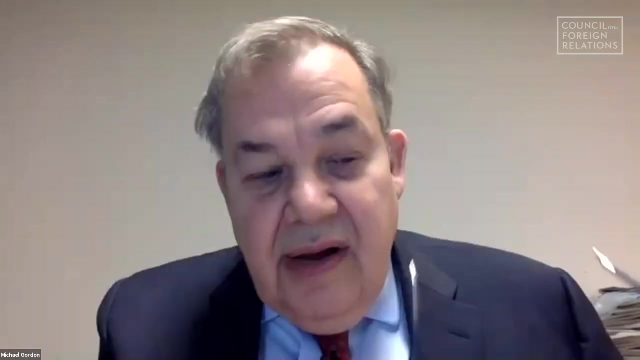 was at the Nuclear Threat Initiative and was a representative to the IAEA. And Fred Kaplan, who's an author and journalist. His latest book is called The Bomb, And Fred and I were colleagues in Moscow just a little while ago. So with that, all of this is on the record. I'm going to start it off by asking a question. really, 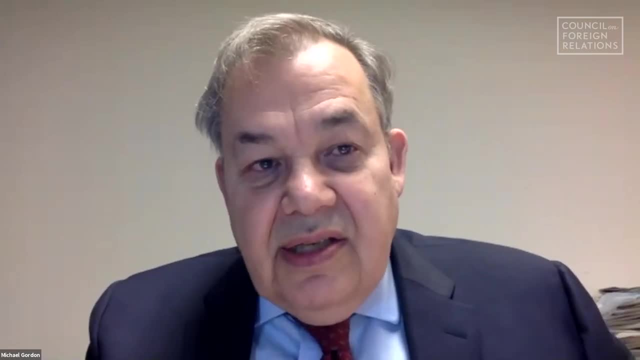 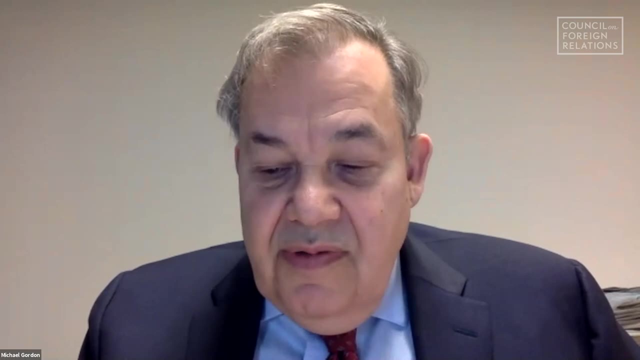 to each of the panelists, And then I'm going to ask a separate question to each and a follow-up, And then, after about 20 minutes or so of this, we're going to open it up to the members who are participating in this. 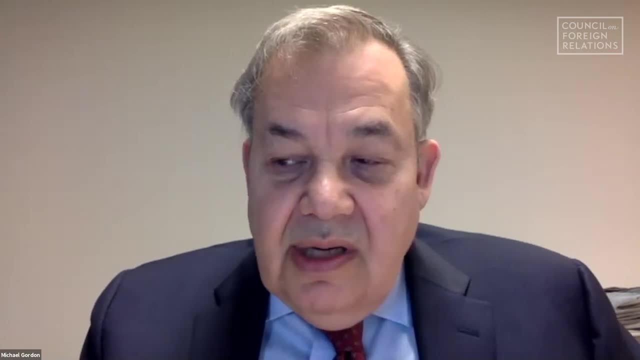 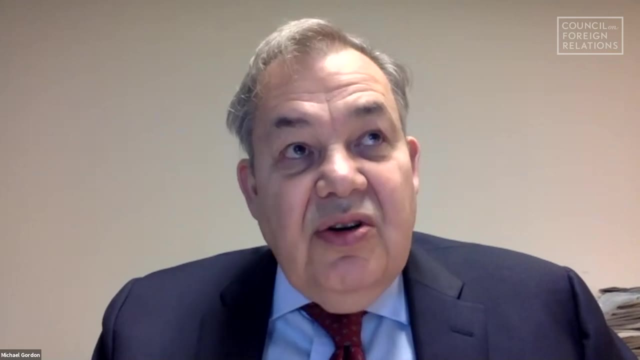 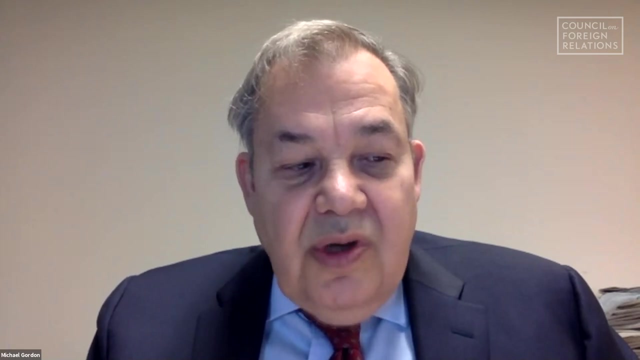 So for Bob Einhorn, I thought maybe you could start us off by giving us an overview of you know set the stage of what's happened since the NPT entered into force. How successful or unsuccessful has it been in your view? You know what's gone right, What's not gone so well. 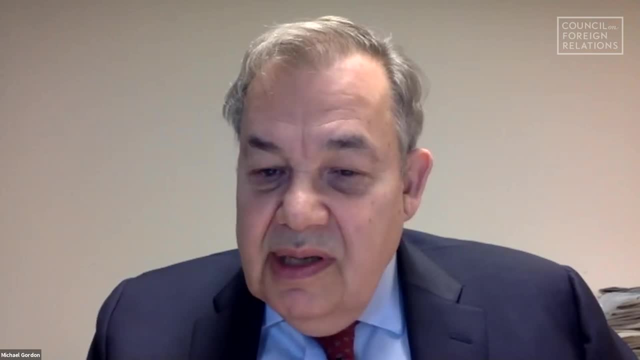 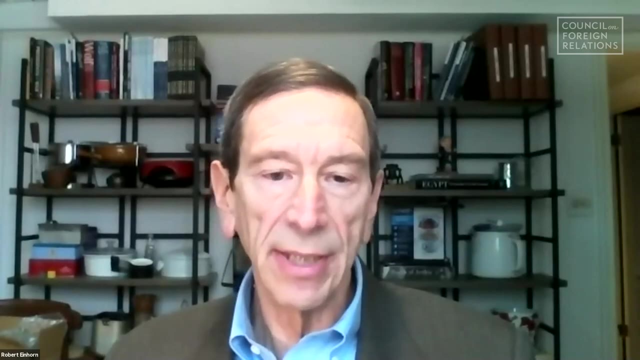 And just give us an overview, And then I want to ask you a follow-up, please, Michael. thank you very much, And for me it's a special honor to participate in the Council's Paul Warnke lecture. I worked closely with Ambassador 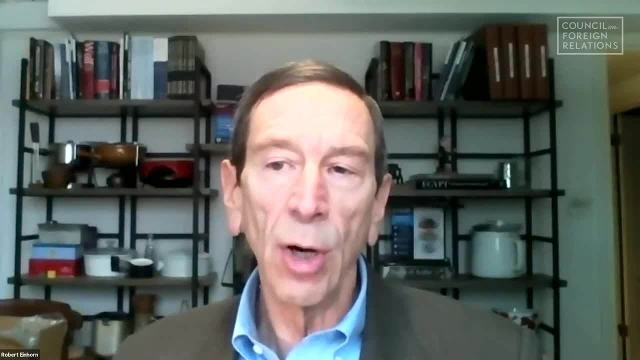 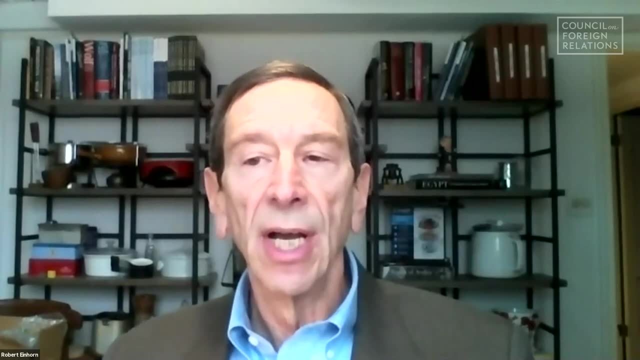 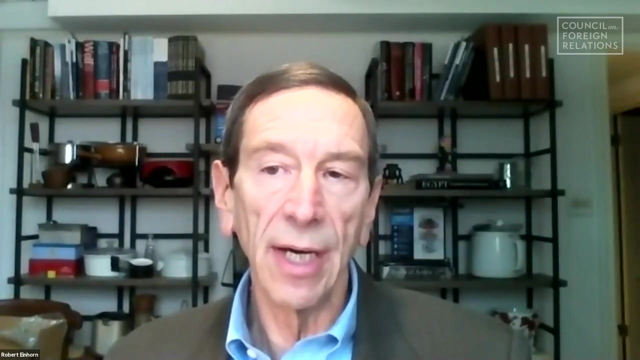 Warnke when I was a member of a US arms control delegation that he was leading in the late 1970s. Paul was a very powerful advocate of arms control measures that strengthened US national security And he was the most effective negotiator I've ever seen. So I'm 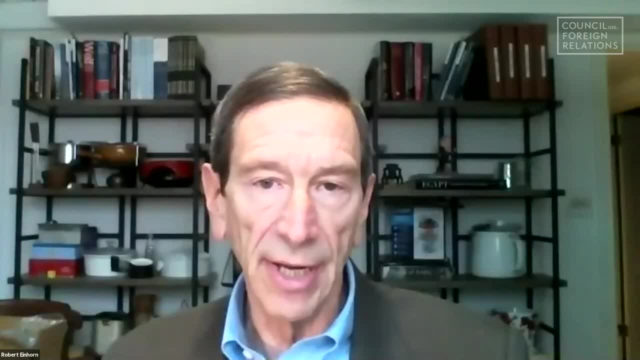 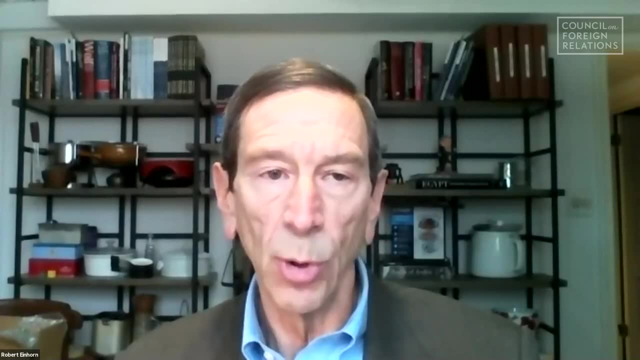 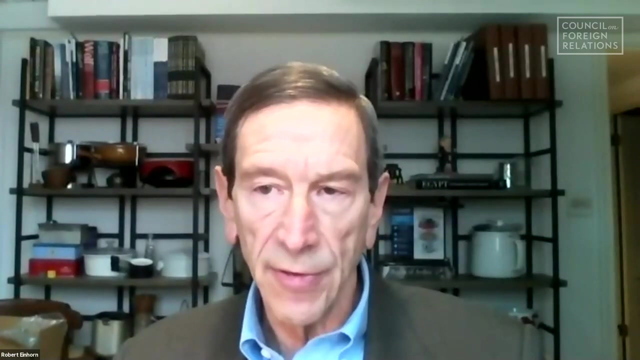 very pleased that the Council has this annual event. Let me turn to your question, Michael The. in my view, the NPT and the broader nonproliferation regime that the NPT is the foundation of has been remarkably successful. There are now 190 states party. to the NPT only five that aren't India, Pakistan, Israel, South Sudan and North Korea, which was a party and withdrew. Many states with the technical capability to acquire nuclear weapons chose not to do so, including many US allies who, of course, had security guarantees. from the United States. Several states pursued nuclear weapons but voluntarily abandoned their programs. That includes Egypt, Argentina, Brazil, South Korea actually built a small nuclear arsenal, but decided to eliminate them with the transition from two-black majority rule. Belarus, Kazakhstan, Ukraine inherited nuclear weapons, but they were not able to acquire nuclear weapons. You know they had nuclear weapons on their territory with the collapse of the Soviet Union, but they decided to give them up and join the NPT as non-nuclear weapons states. Iraq, Libya, Syria sought nuclear weapons but were pressured to halt their programs. in some cases by the use of military force, And Iran's nuclear ambitions have been blocked by the Iran nuclear deal, at least for the time being. So, despite all kinds of dire war about a world with many nuclear-armed states, we haven't had a single addition to the nuclear club. in the last 30 years, And this has created the conditions in which the peaceful uses of nuclear energy could be safely pursued. The NPT has also encouraged progress toward nuclear disarmament, which is another of the NPT goals, which is embodied in Article 6 of the NPT. Cold War nuclear arsenals have been dramatically reduced, especially by Russia and the United States, in the course of a succession of strategic arms agreements. But recently, with the return of great power competition, that progress has been stalled And further nuclear reductions are unlikely for quite some time. Many non-nuclear weapon states party to the NPT have charged the nuclear powers that are party to the treaty with a failure to comply with their obligation to pursue nuclear disarmament, And they have looked to other solutions to promote nuclear disarmament, such as a treaty on the prohibition of nuclear weapons. 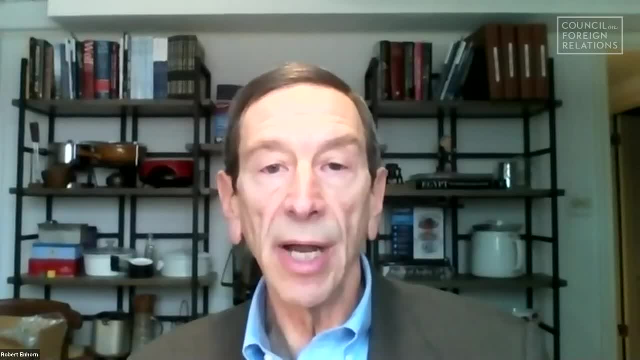 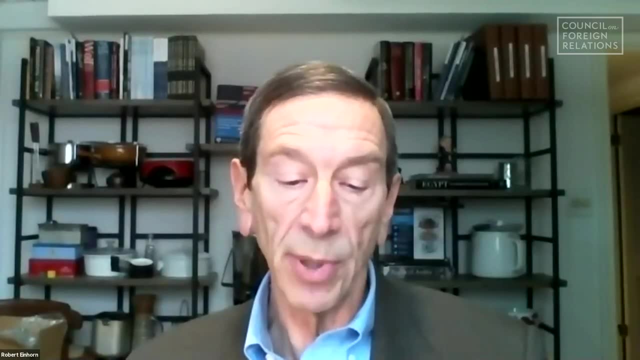 There's been a polarization among NPT parties that threatens to weaken the NPT as a barrier to nuclear proliferation. So overall, in my estimation, the non-proliferation regime, the NPT in particular, has been remarkably successful, But there are challenges for the future. 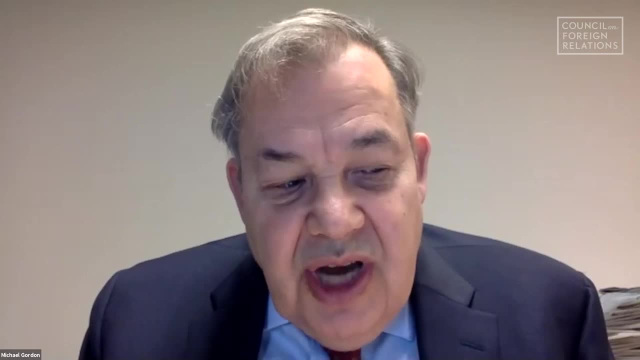 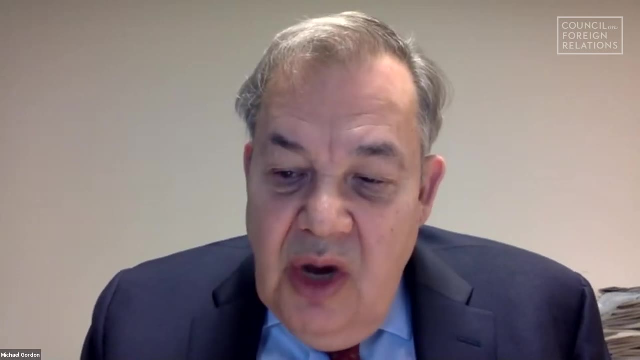 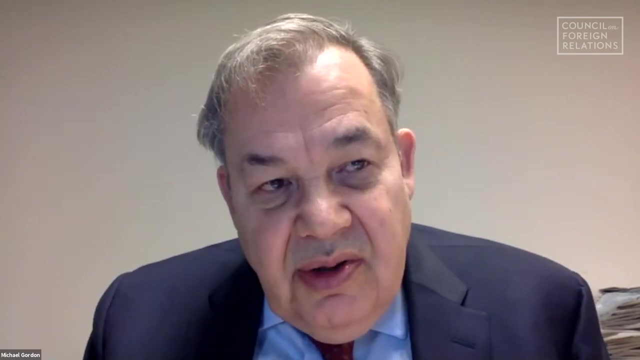 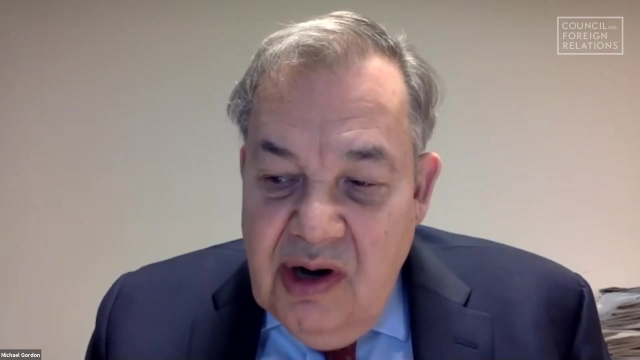 Well, let's take up some of those challenges. Maybe I'll switch to Laura Holgate and just ask you: what do you see is some of the particular challenges for the regime in coming years? Which countries specifically should we be concerned about? And also, as Bob mentioned, Article 6 of the NPT. 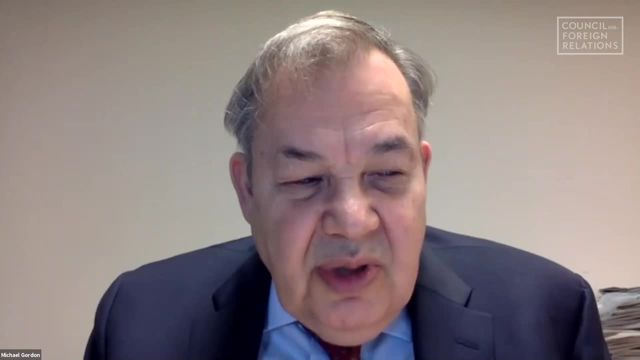 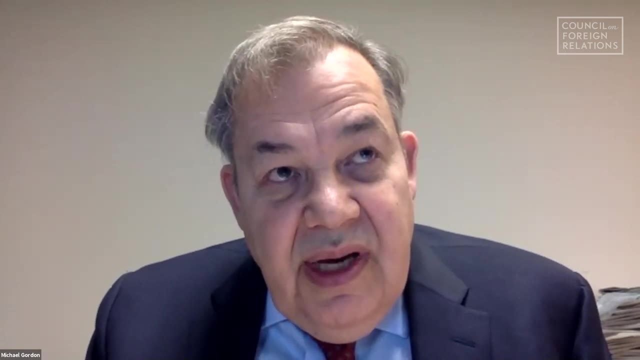 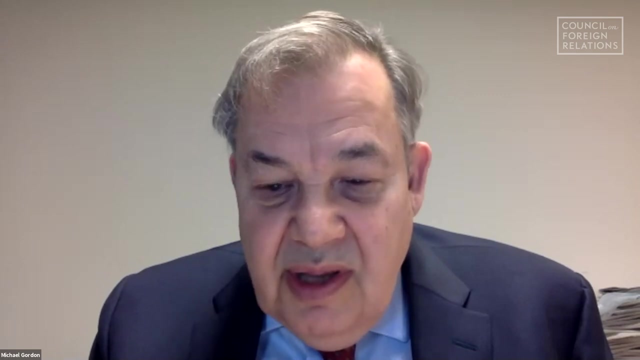 says that there is an obligation on the parties to pursue negotiations in good faith. Where does China fit in on that? Should they be pursuing nuclear negotiations not merely as an end in itself, but also as part of the program to strengthen the NPT? 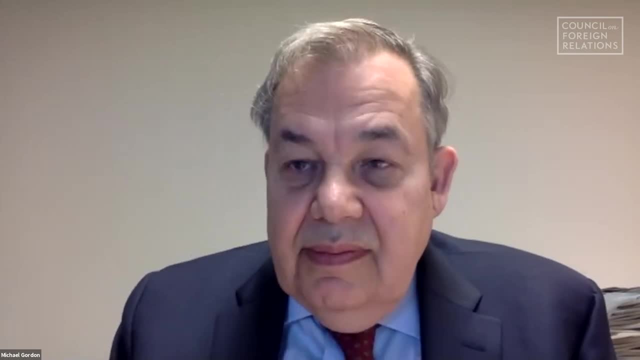 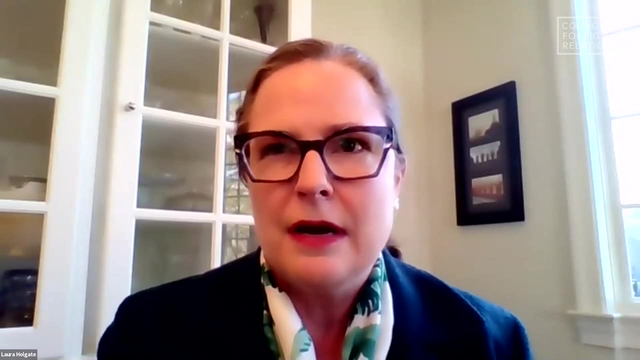 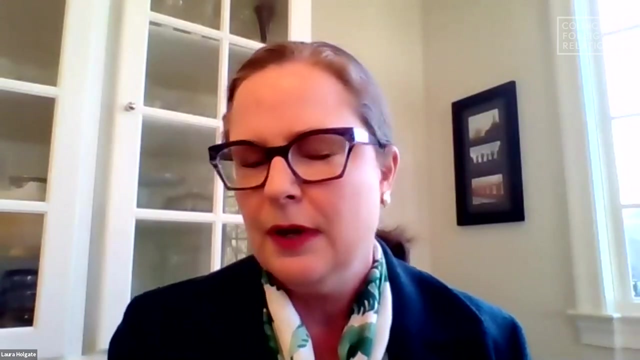 And if not, how do we deal with China? Well thanks, Michael. I think Bob obviously laid down a really important reminder that the nonproliferation treaty has been quite successful at the things it set out to do, But there's a lot of changes in the current and future environment. 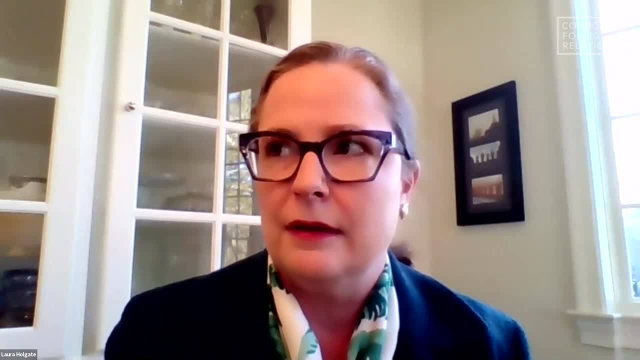 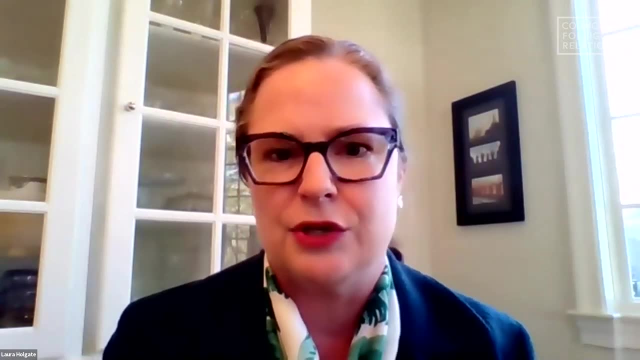 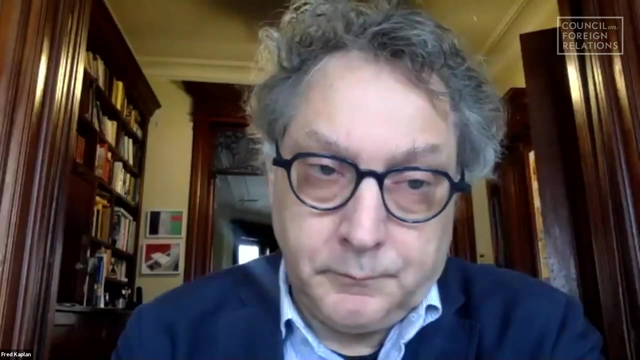 that the treaty is not well suited to and that we need to think about the treaty in the context of a broader set of the nonproliferation regime, which has a number of formal and informal components to it. One of the things that we're seeing is the rise of non-state actors. 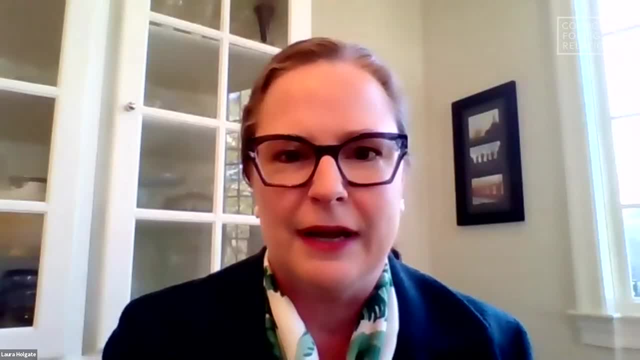 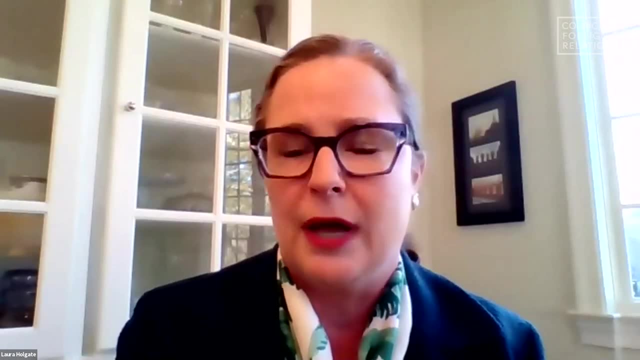 both malicious, obviously, in the form of extremists, violent extremists, but also potentially beneficial, or at least neutral, when you're looking at global companies, whether it's trading companies, whether it's nuclear energy companies, who do not play the normal role of states. 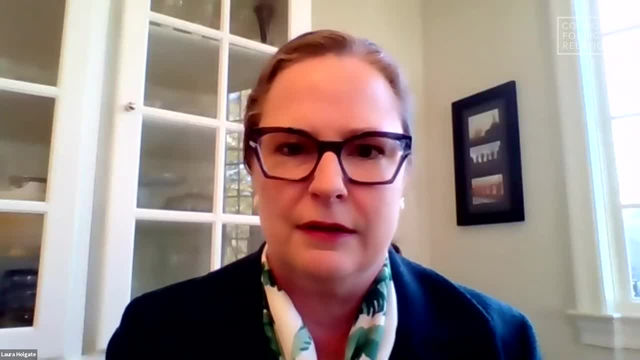 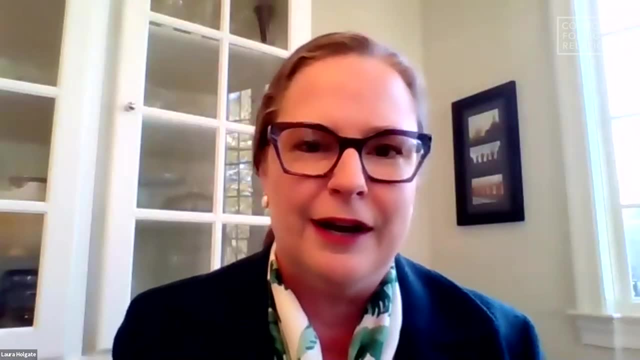 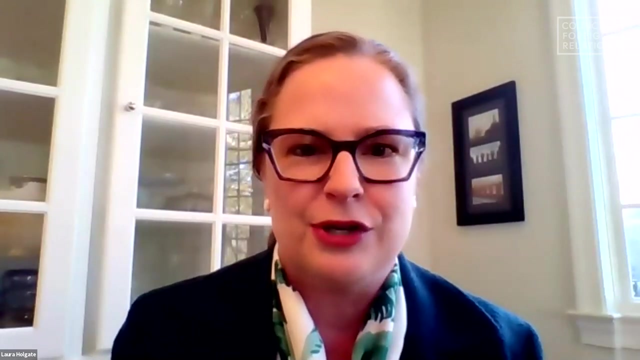 but whose decisions have an impact on the success or failure of some of these elements, And I would even include non-government organizations like the Nuclear Threat Initiative among the beneficial non-state actors. but where action is, We've been able to stimulate action that has a real-life outcome. 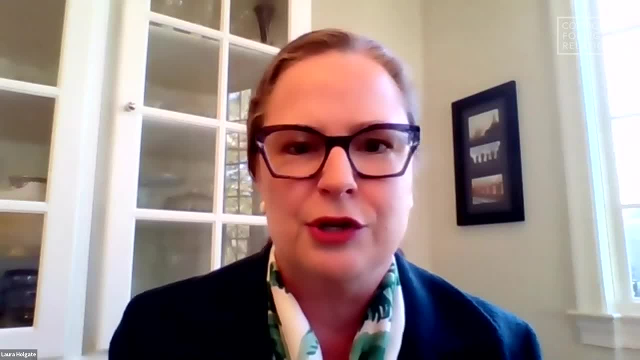 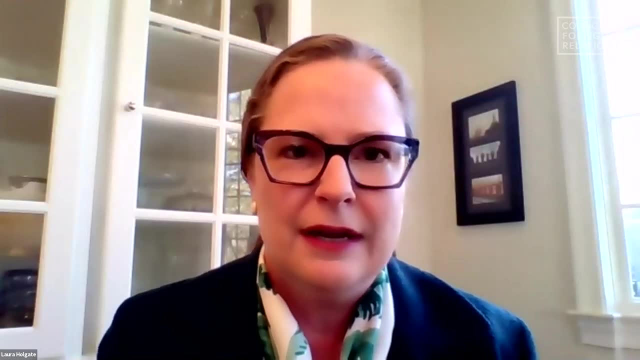 And so the system isn't really well structured to accommodate that range of non-state actors. I think we've also seen that US and Russia used to share a common perspective. They were both negotiators of the lead negotiators for the nonproliferation treaty. 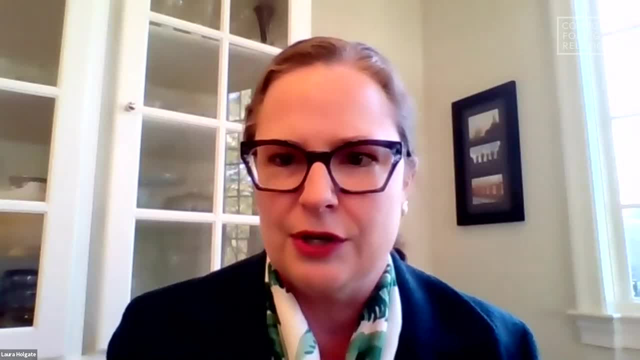 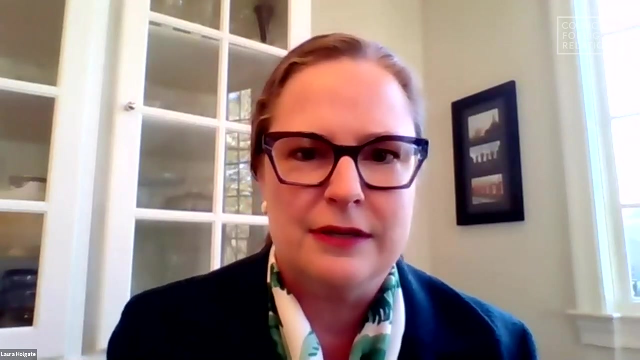 Right now we have very different views between US and Russia of what's the value of the treaty. what role do we individually have or collectively have regarding the various aspects of the treaty and how we interact around things like the safeguards component of the International Atomic Energy Agency's verification responsibilities? 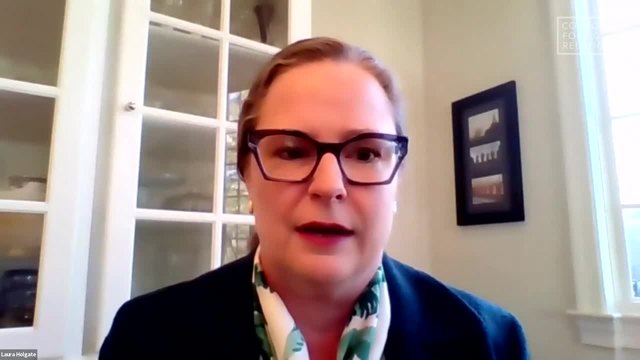 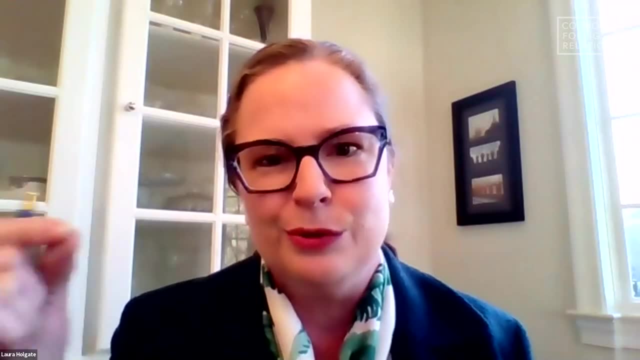 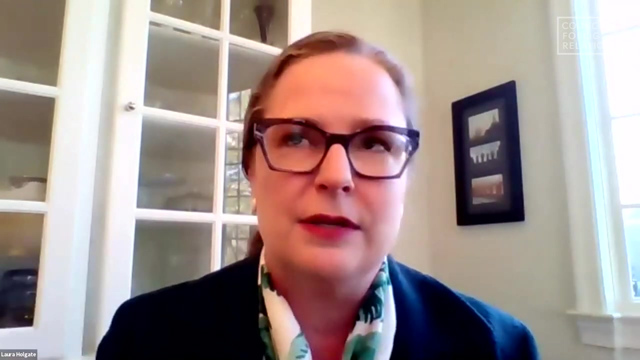 as well as nuclear security- security of nuclear materials and weapons- And US and Russia have very different perspectives there, So that lack of consensus among the two main nuclear actors, I think, makes it really challenging From a The other point about the US and Russia piece, though. also is that it's no longer that we that the biggest nuclear threat has to do with US-Russia intentional, massive, mutually assured destruction. It has more to do with accident miscalculation and so on, And there the NPT offers us almost nothing in terms of protection. Regarding China, clearly China accepted the same responsibilities in Article VI as US, Russia, France and the UK to pursue good faith nuclear nuclear disarmament. China's been successfully hiding behind the significant, significantly larger arsenals of US and Russia. My personal view is that there's one more round of US-Russia reductions. that would be important, but then the energy should shift to the P5 as the venue. I don't think it makes sense for China to be negotiating with the US and Russia on its own. 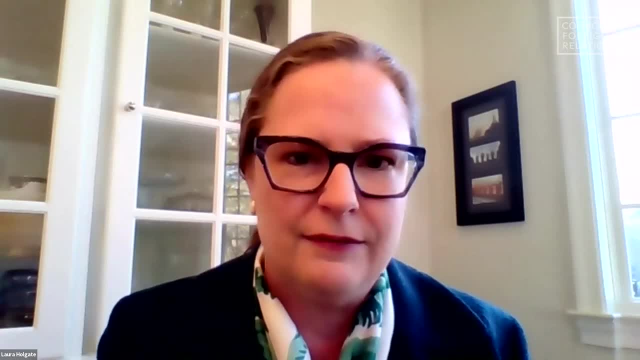 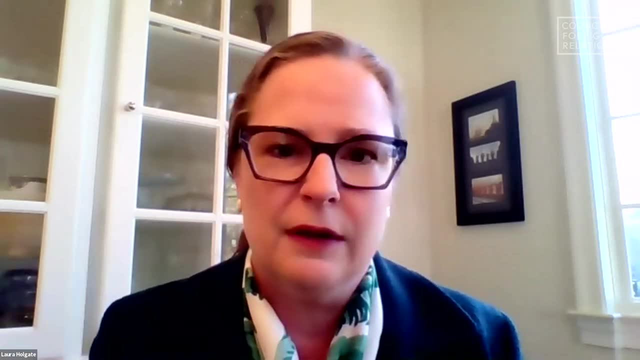 I think it's a conversation that needs to be about all of the P5, because they all have the same Article VI commitment. There's work that can be done now and was started. you know 10 years ago that Bob was involved in. 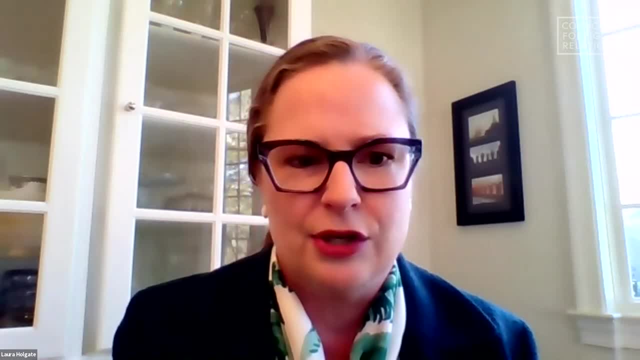 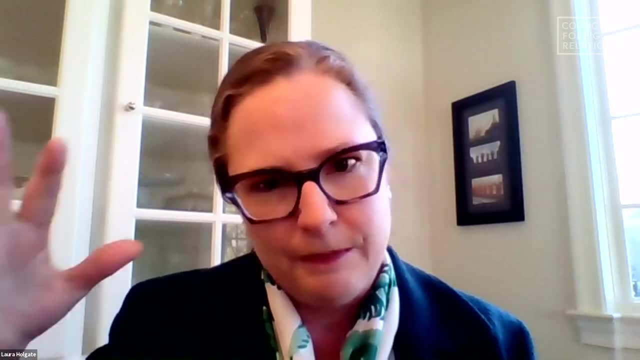 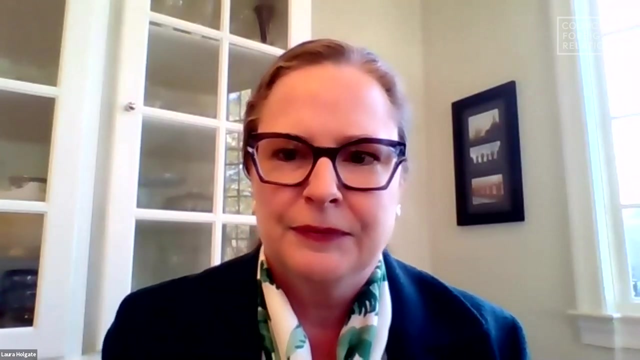 of trying to bring some of that disarmament discussion and culture into the P5 context And that can be reinvigorated, expanded as a creating a path to engage China, along with the other countries, in a future disarmament discussion. So for 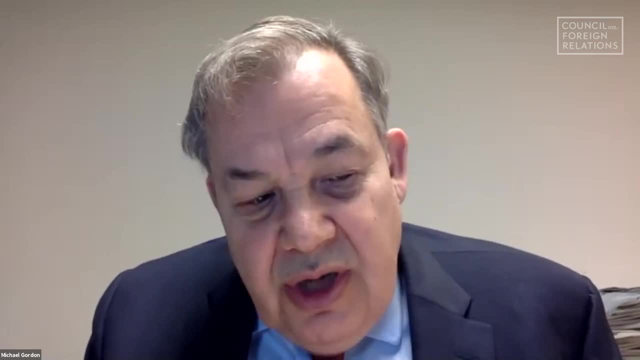 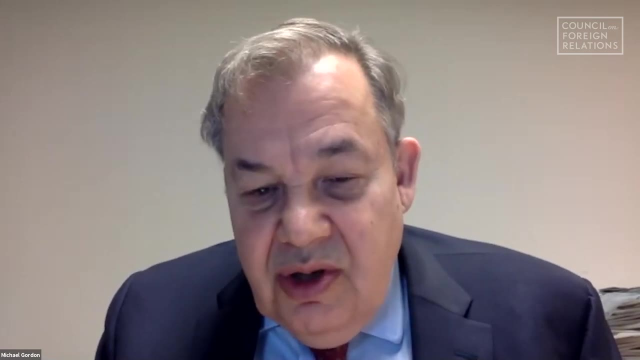 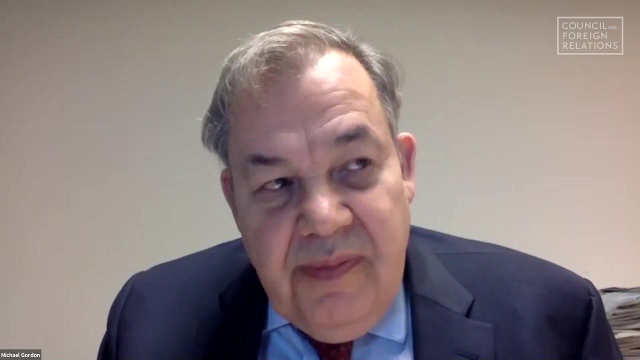 for Lisa Gordon-Agerty a question. With the renewed concern over climate change and the new administration, I was certainly going to emphasize that people see a some people see a growing role for nuclear power in the future. What are the technological challenges that? 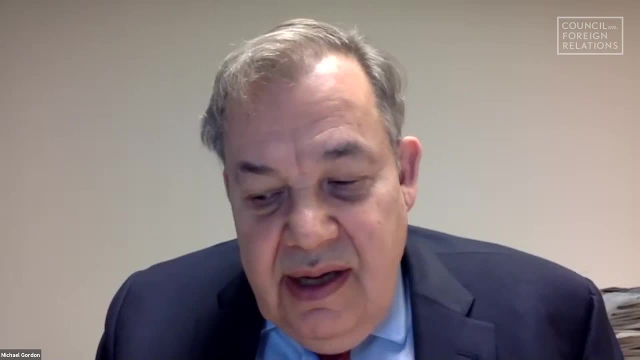 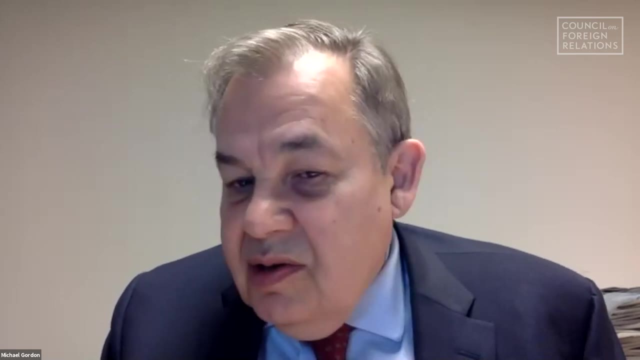 if that were to come to pass, that the further embrace of nuclear power might pose for the NPT, for counterproliferation efforts, and what are the technological solutions, if there are any? Can you address this from the sort of technology side? 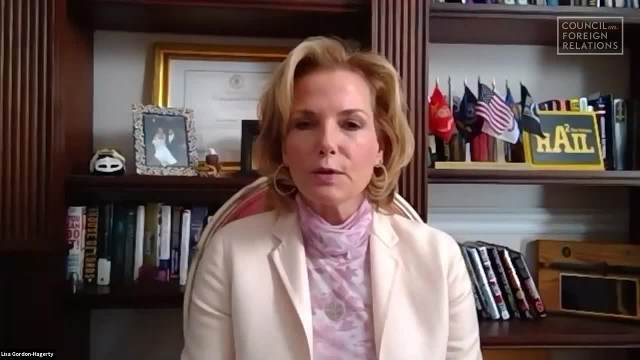 Well, thank you, Michael, for the question, And I also want to thank the Council and the Warnke family and my counterparts on the panel today, as well as those that are listening. This is a really important topic. It doesn't deserve just an hour. 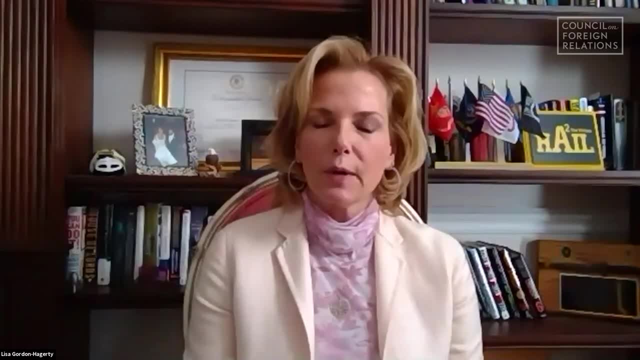 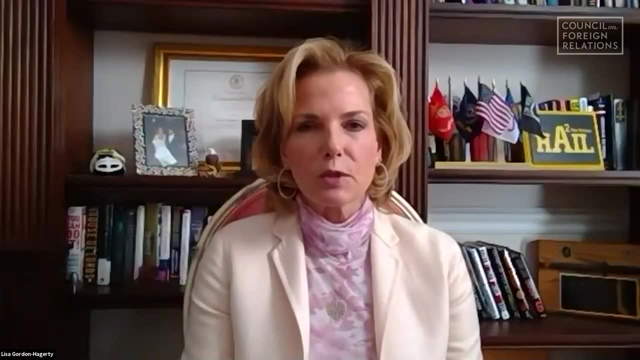 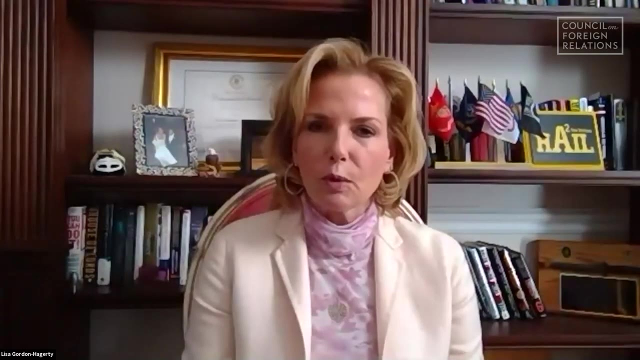 It deserves much more continued interaction, So I look forward to being hopefully part of that continued conversation through the Council. I too want to acknowledge the success of the NPT over the last 50 years. I think it's had positive contributions towards global security. 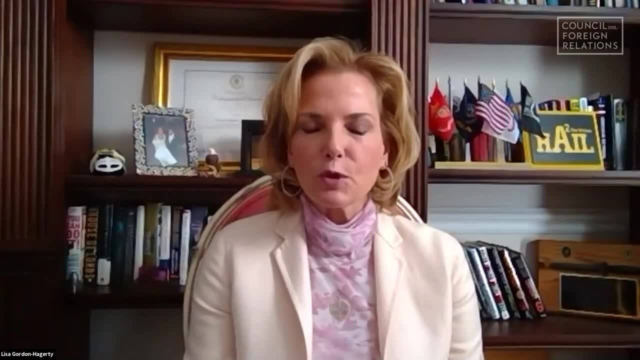 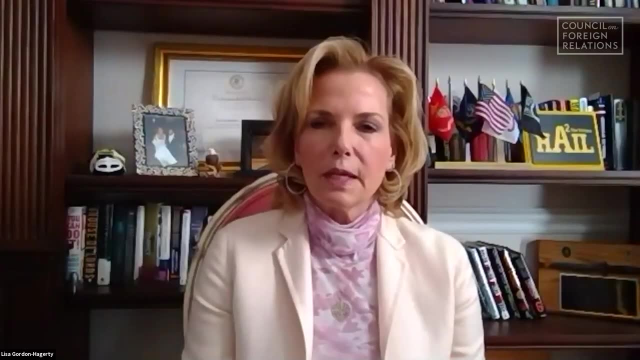 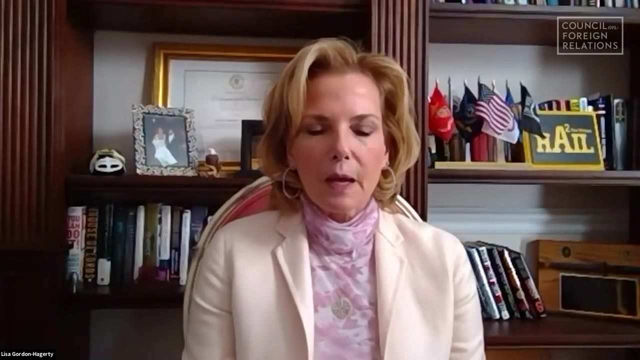 as Bob and Laura both laid out, And even in a virtual seminar like today and how we're all working basically virtually throughout the world, the NPT continues to be successful in different areas in advancing the three pillars of the NPT. With regard to the NPT, 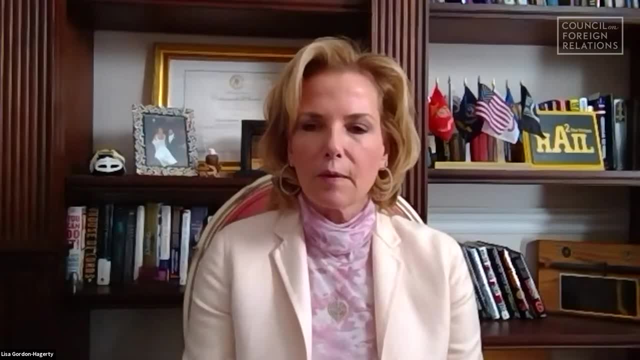 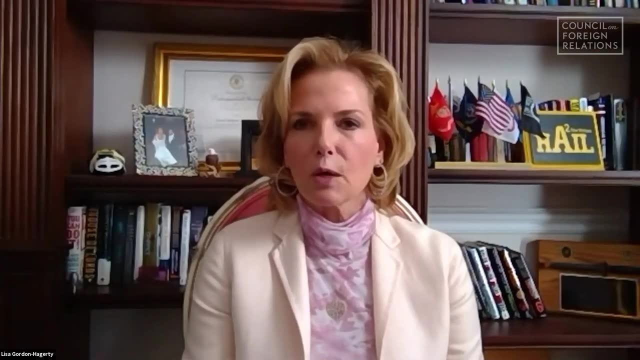 with regard to your question on proliferation and on the capacity of potential, the peaceful uses and how, of course, we're all working towards a carbon-free climate and where we're looking at emerging technologies, whether it's small modular reactors or other technologies. 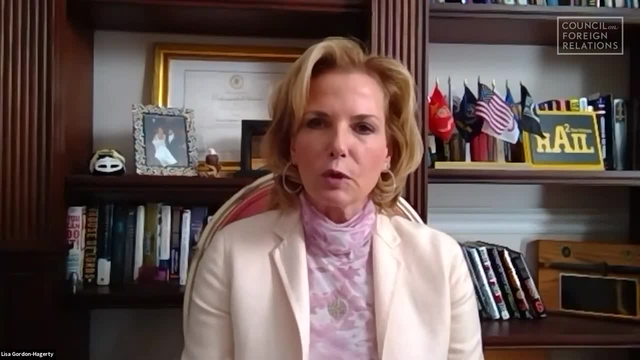 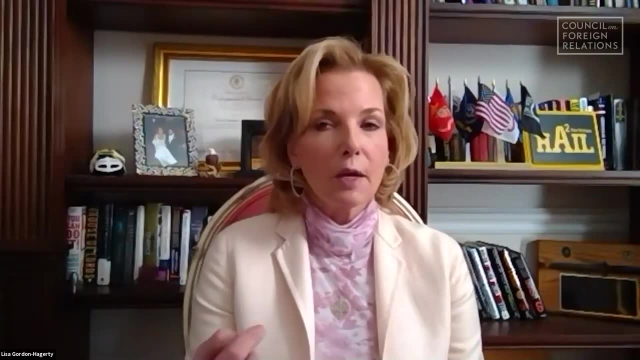 I think we have the benefit of being able to look back on the last 50 years of the NPT, making progress, learning about the finding, the lessons learned, the shortfalls as well as the successes that we've all encountered in the NPT. 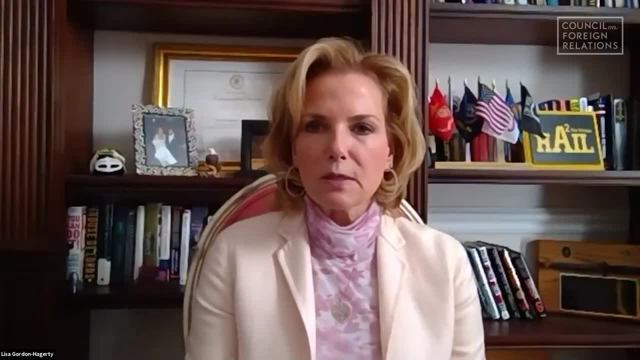 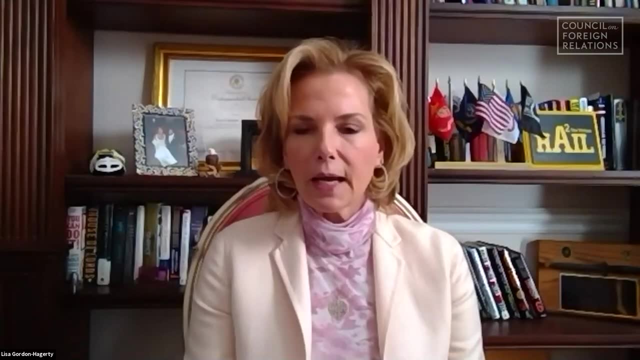 Learning from that through the robustness of the United States government, through the technical expertise present at NNSA and at other agencies. But again, prevention is where you know that to me is a strong suit. So from a carbon-free future, 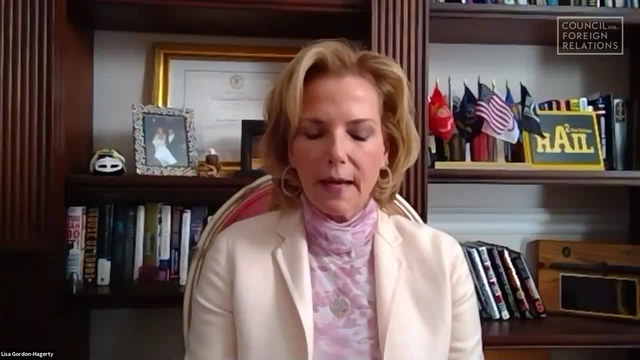 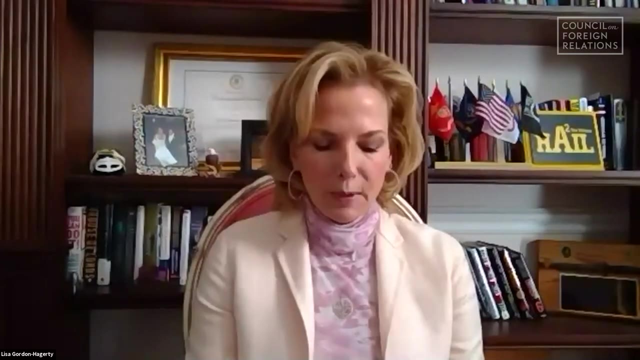 IAEA plays a critical role in that in peaceful uses. There are mature nuclear energy technologies out there, capabilities in countries that administer them, and it's in all of our best interest to make sure that we are all working towards the progress of peaceful uses. 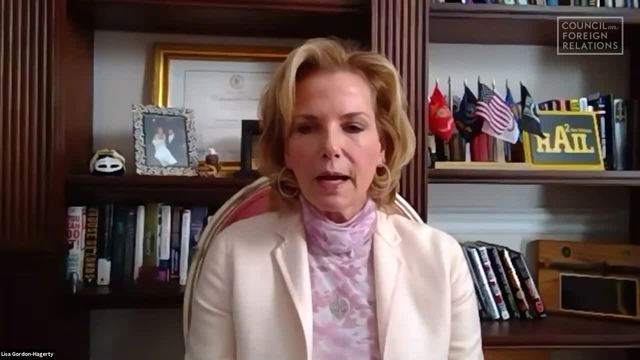 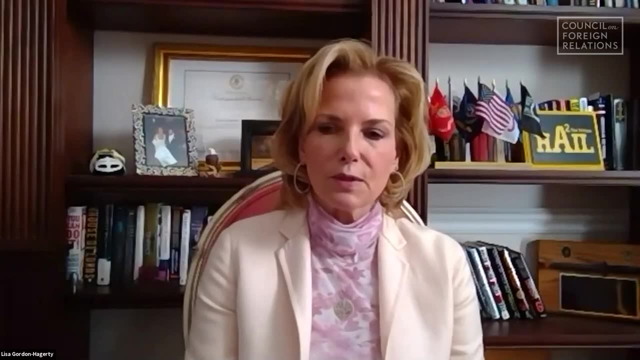 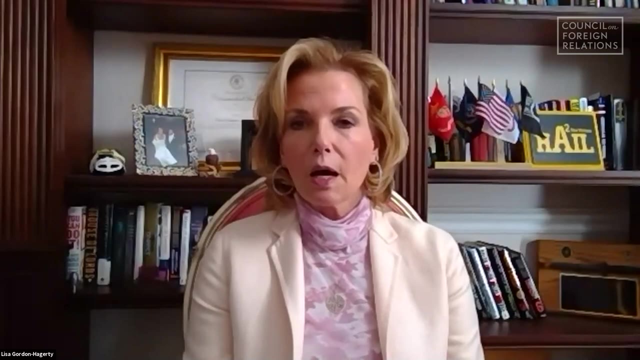 My concern is that, while we have emerging technologies that have certainly been for the benefit of health and safety, increased health and safety and security and safeguards, there are some emerging technology of which I'm very concerned, including AI and additive manufacturing. We need to get ahead of these capabilities rather. 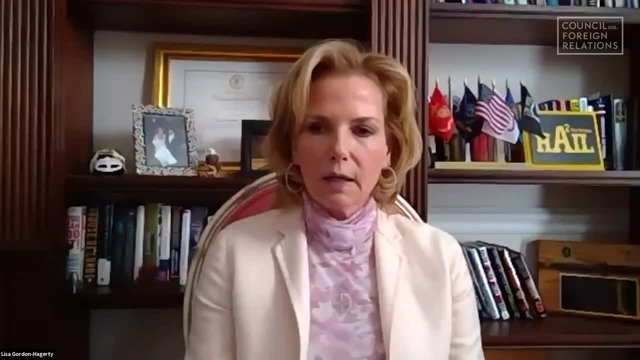 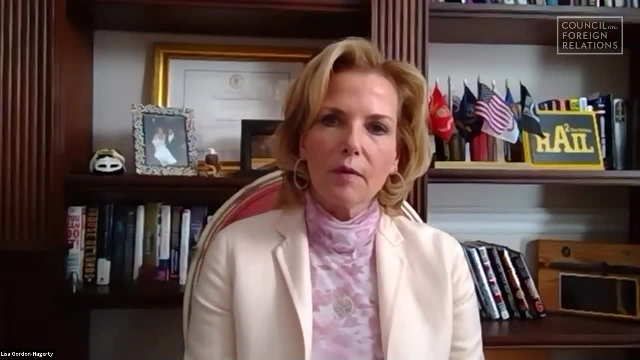 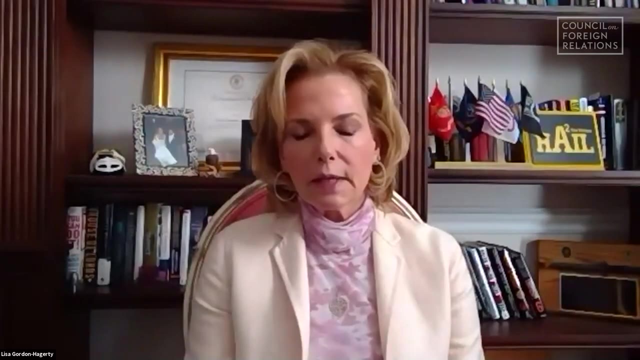 than seeing them being exploited in malicious ways. There are technologies and capabilities resident in the United States government and other places that can address these issues before they are used for malicious intent. There's no doubt, like I said, that the technologies of today have served great use for improving the health. 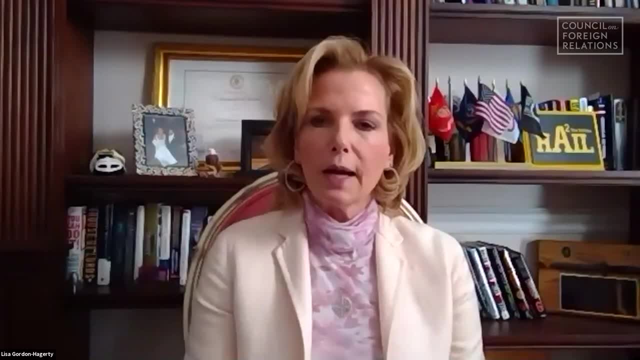 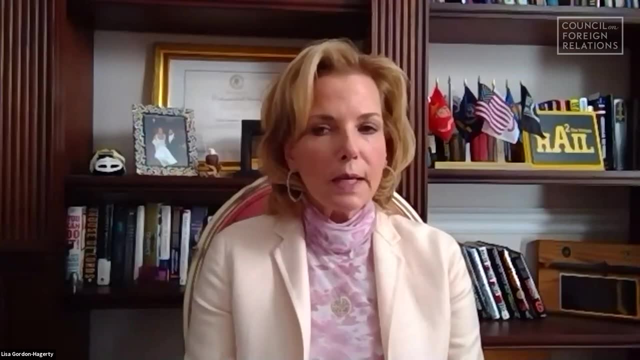 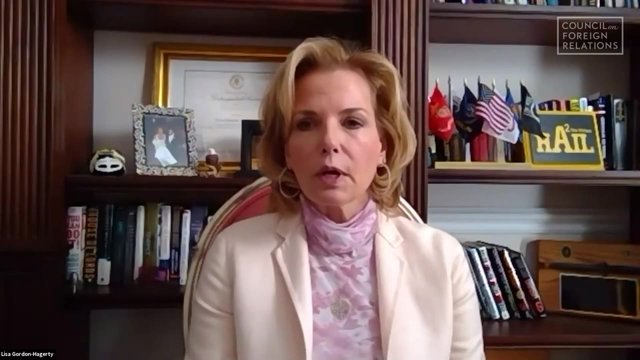 and safety of the globe. However, we do have some other emerging things, unlike anything we have seen in the traditional nuclear energy sphere. So we need to get ahead of that And, I think, through the robustness of the interagency, the US government and other partners- the UK, France- 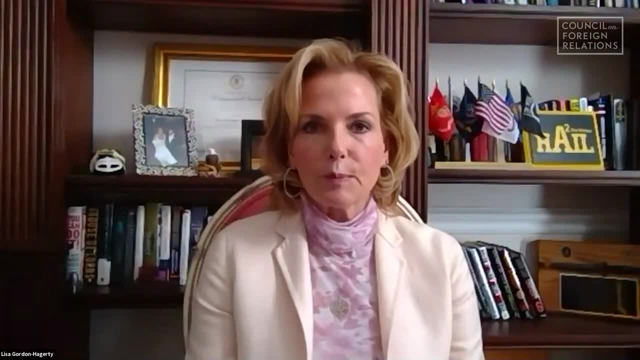 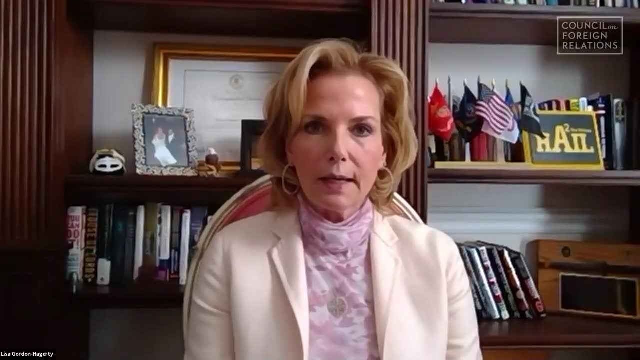 and others, and perhaps even using the P5 generally. I think there are ways of getting ahead of this now, because it's only going to get worse. We've seen what AI has done, We've seen what additive manufacturing can do, And it's unlike anything we've ever seen before. 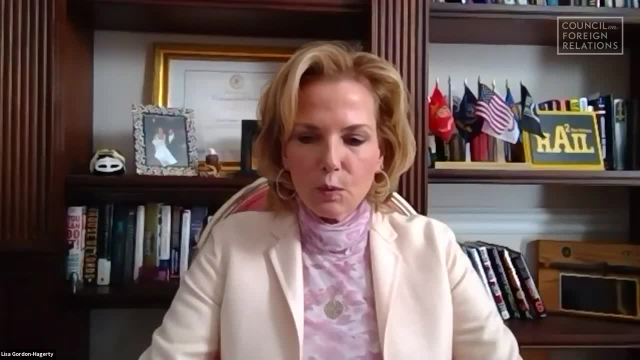 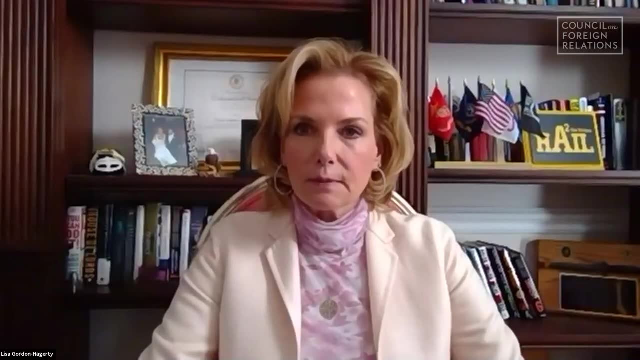 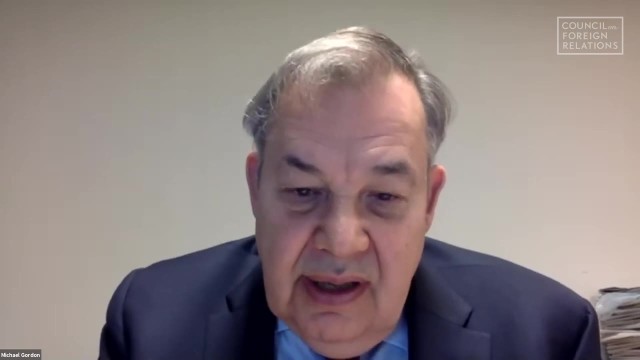 So those are a couple of things I'd like to ensure, without getting too wonkish in the technical aspects. I think there are a lot of people on this call that will appreciate the importance of emerging technologies. So thank you. So, Fred, when you wrote your latest book, The Bomb, 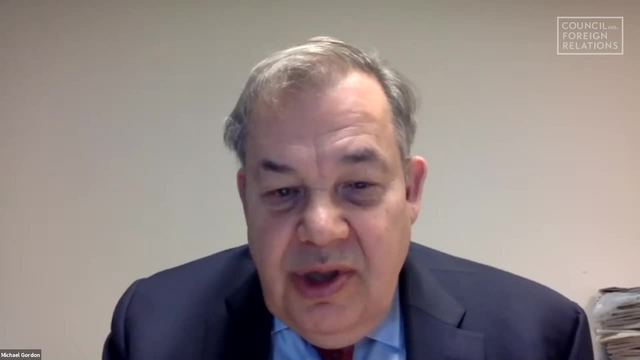 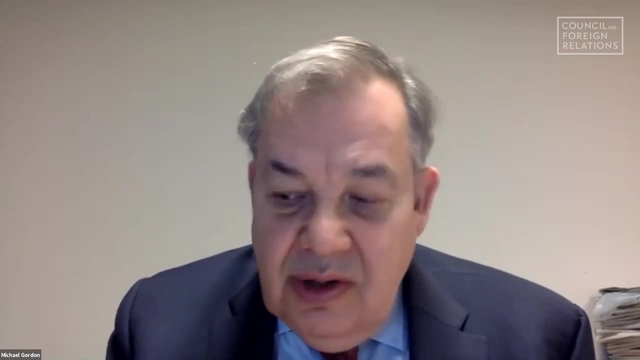 you did some research into the origins and kind of prehistory of the NPT. Maybe you could share a little bit of that with this group and also what the implications or lessons are for the future of the NPT. Well, thank you, Michael. 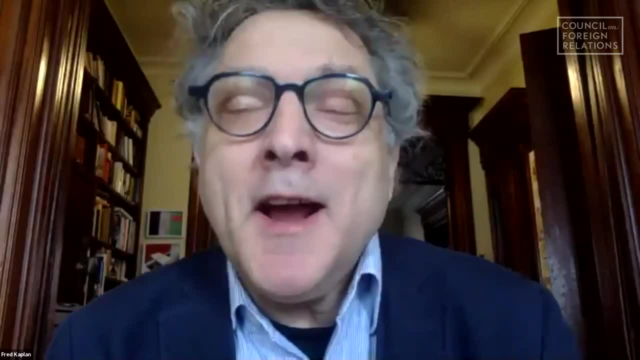 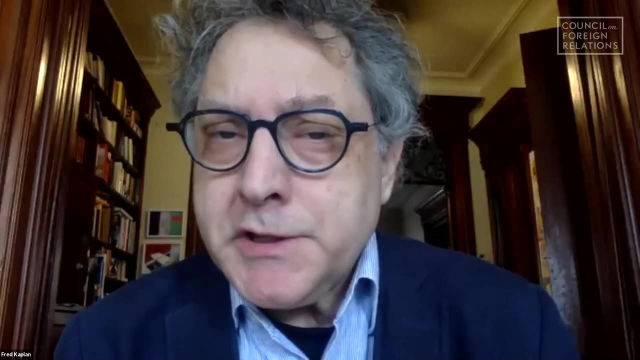 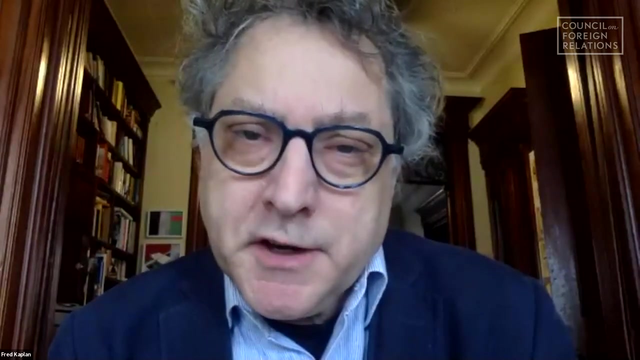 And thanks the Council. Good to see you all again. Yes, there's a whole history to this that really I wasn't familiar with until doing the archival research. So the impulse toward negotiating an NPT started in 1964 when China tested a nuclear bomb. 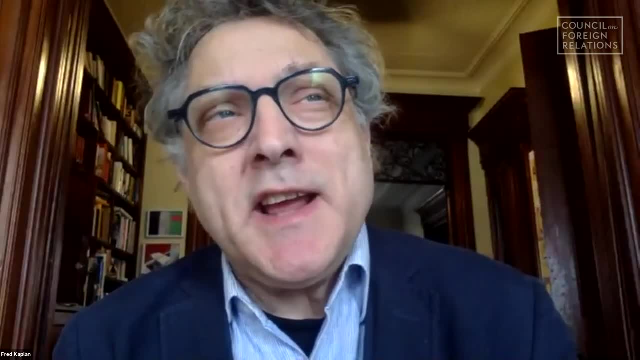 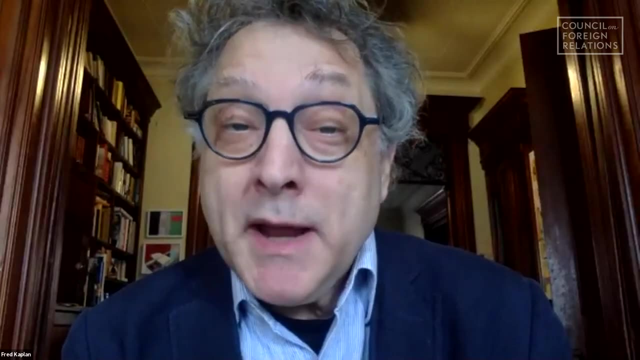 Secretary of Defense at the time, Robert McNamara, didn't see this as an imminent threat, but realized that there were about six other countries that also had the capability to do this and thought that might destabilize the world. So he wondered if there might be an international treaty. 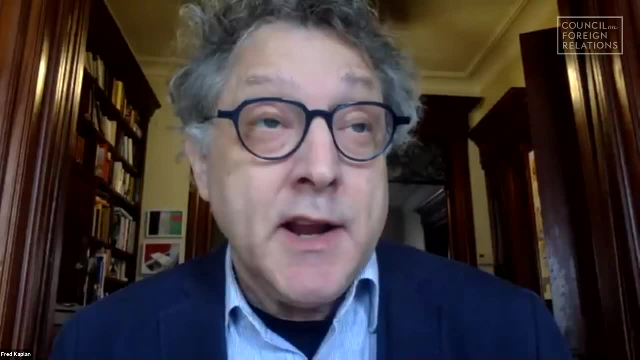 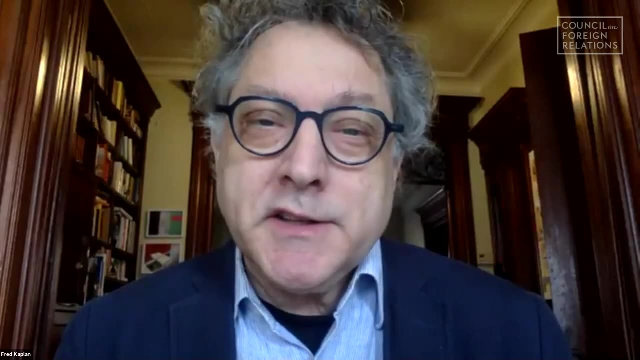 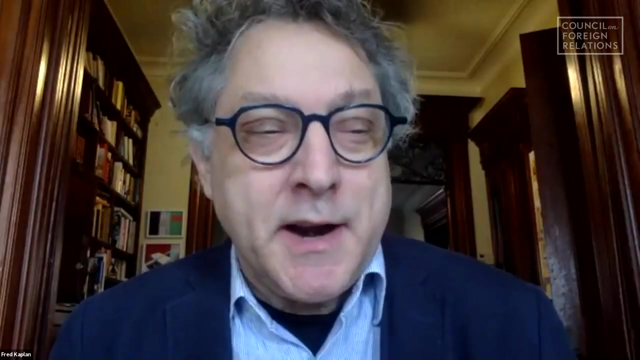 to just ban the development of nuclear weapons. Remember, keep in mind, that this was before there were any meaningful US-Soviet arms control treaties. This was, you know, Khrushchev had just been deposed and Brezhnev had set up stuff. 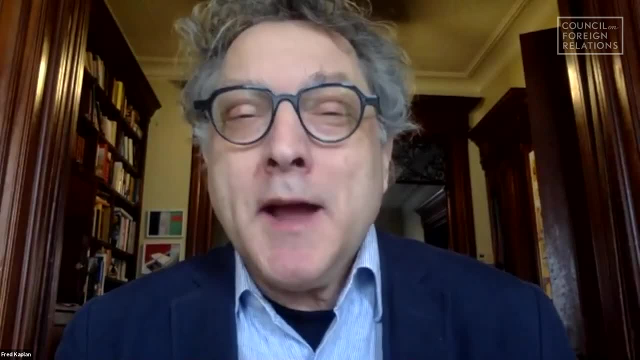 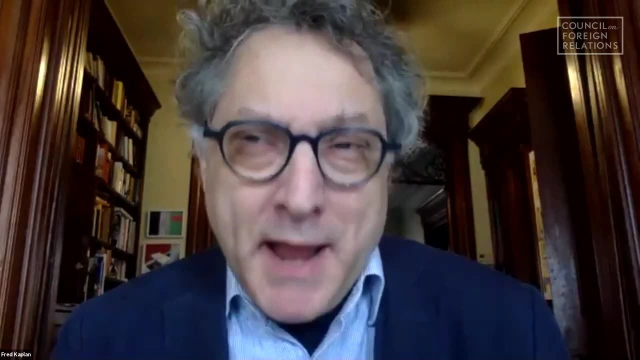 It was a very – this was Cold War times. yet he had this ambition. So he and McGeorge Bundy, the national security advisor, set up very secretly a panel of ten people headed by Roswell Gilpatrick, who had recently been Deputy Secretary of Defense. 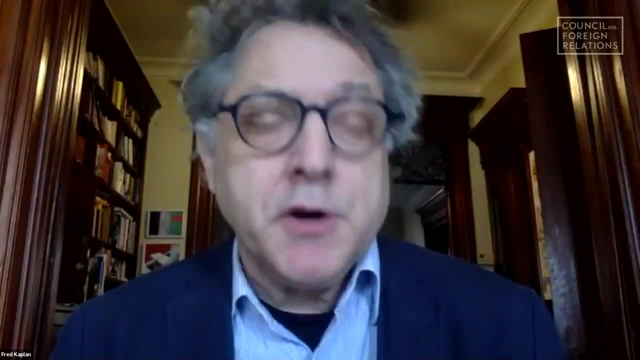 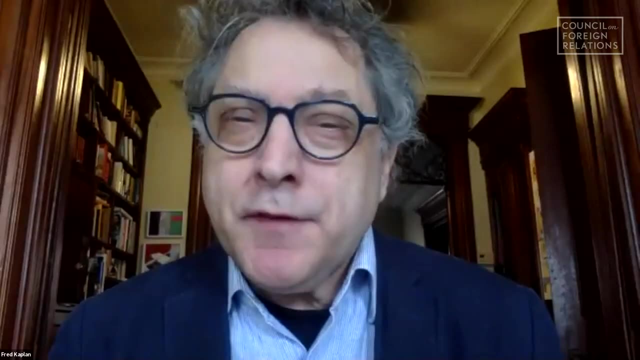 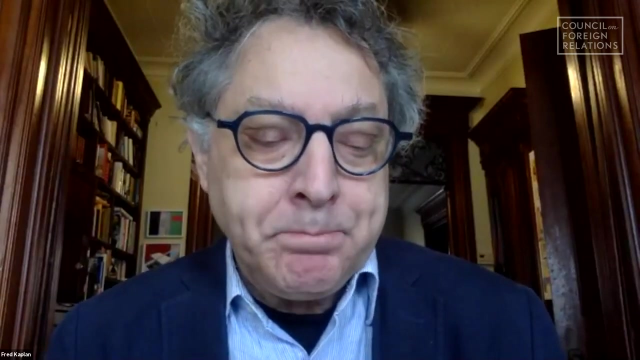 staff director of Spurgeon-Kinney, major arms control advocate- I'm sure many of the people watching remember him- And they had five very, very classified meetings in the executive office building to discuss this at the end of 64, beginning of 65.. 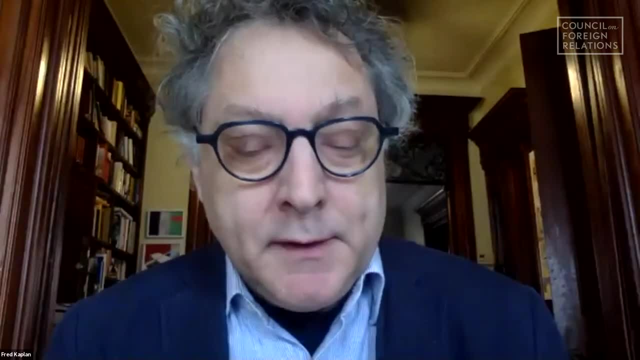 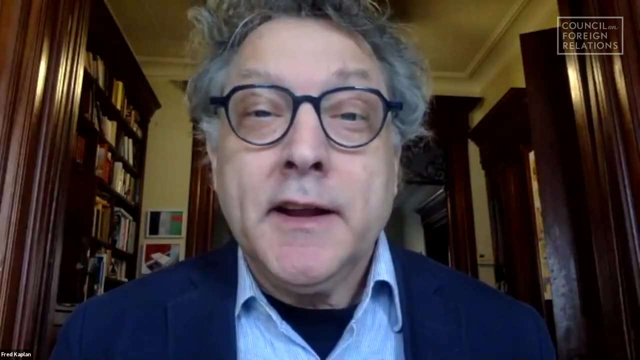 And you know there were some people on the panel arguing: well, maybe nonproliferation is a bad idea. For example, it might be a good idea to help India get the bomb to deter China. I mean, these were discussions that nobody had ever had before. It was starting from ground zero. They came up with the idea that, no, actually on balance it's better that the countries that don't have nuclear weapons still don't, for reasons that are now kind of commonly discussed. but it was quite unusual. 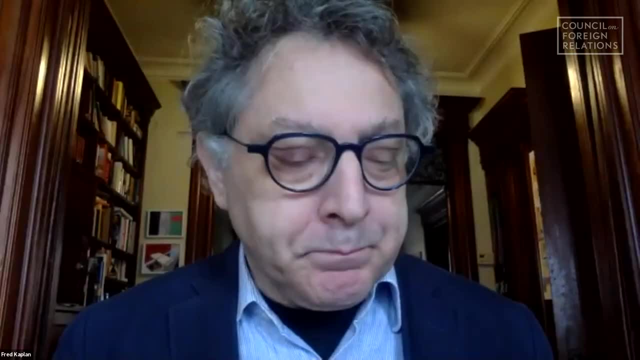 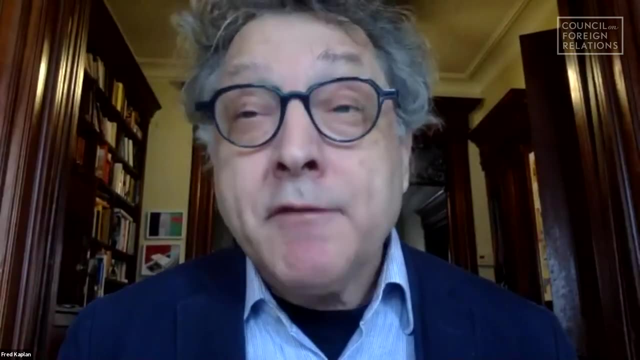 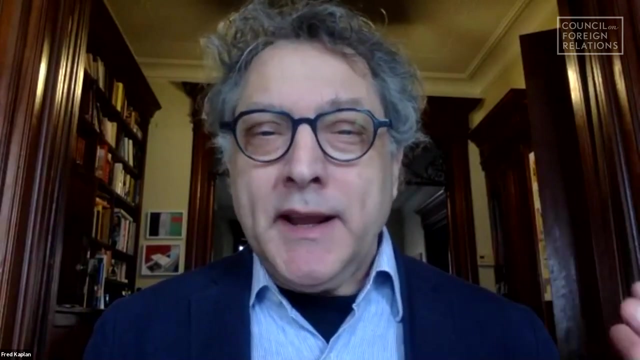 And then came a very interesting proposal. It was thought: okay, the rest of the world is going to forgo nukes, The countries that have them really ought to reduce them. And an idea was floated that there should be a ban on developing any new ICBMs for 12 to 18 months. 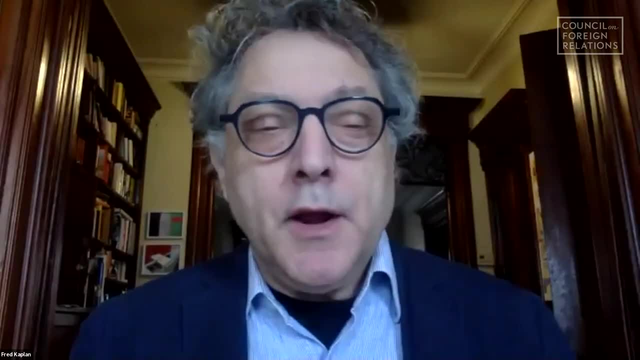 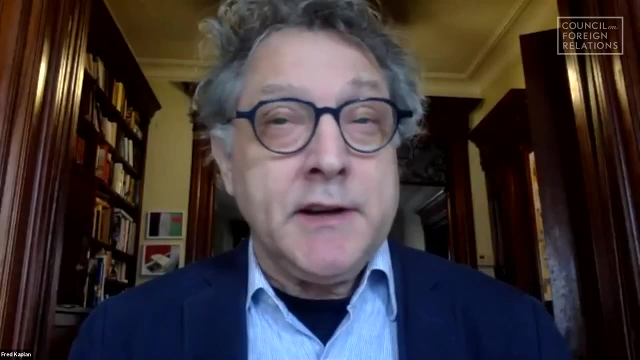 and that the existing nuclear power should reduce their arsenals of warheads and bombs by 30%. The chairman of the Joint Chiefs of Staff didn't like this idea at all, But even Spurgeon Keeney, who was a very ardent disarmament advocate. 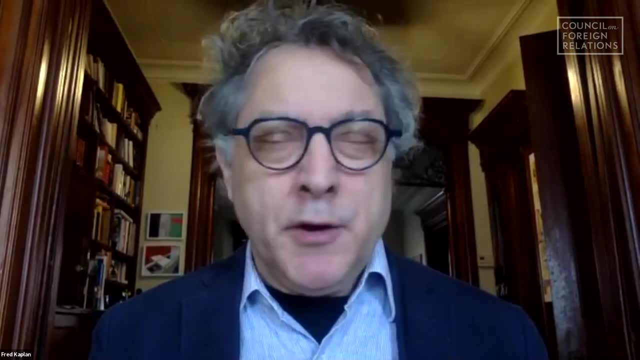 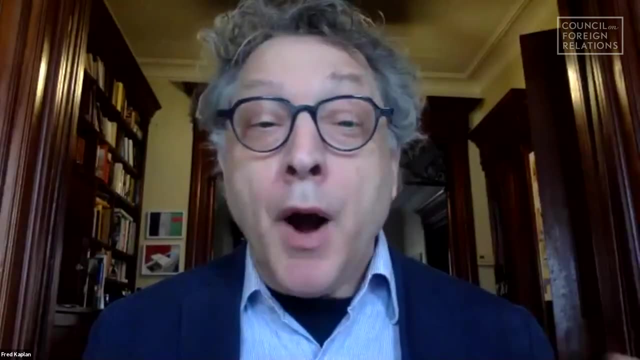 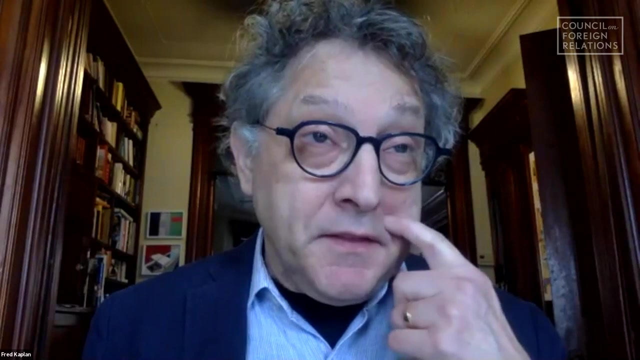 thought this might not be a good idea. A moratorium of 12 to 18 months. we might get locked in And this might hurt our bargaining position in any subsequent arms control talks with the Soviet Union. Now this could have been a crucial turning point. 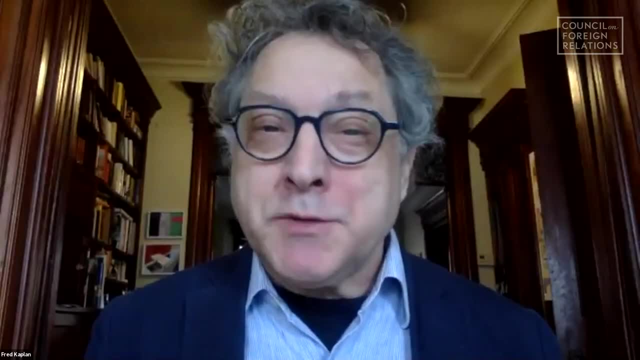 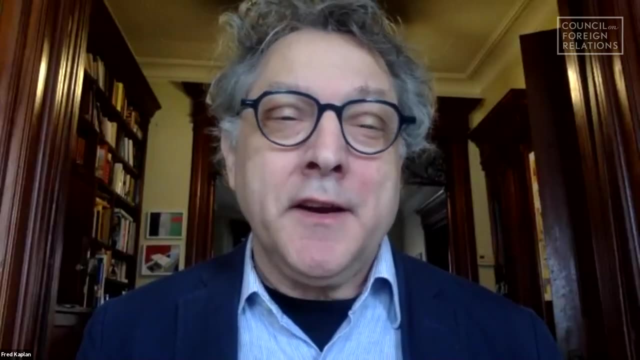 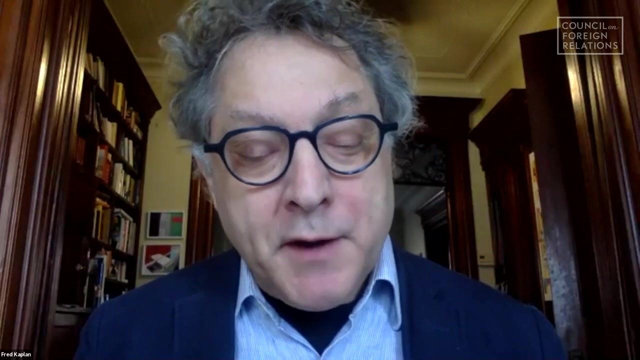 Remember, this is 1965, five years before we developed MIRVs. If this had happened, then the subsequent course of the arms race might have been much less frightening. But then what happened? kind of an encouraging thing. we presented this idea to the Soviet Union. And the NPT as it was presented to the United Nations ultimately was pretty much a joint US-Soviet draft. There were two separate drafts, but they were pretty much identical And again, this was at what might be not quite the height of the Cold War. 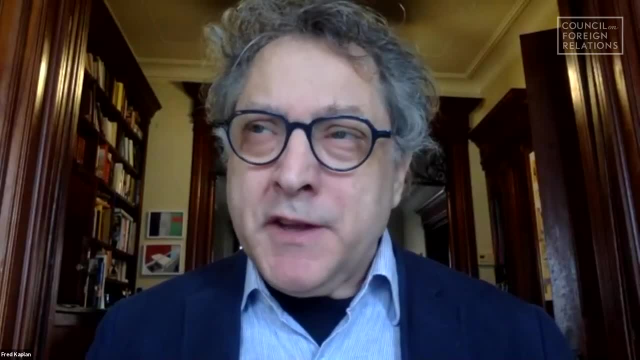 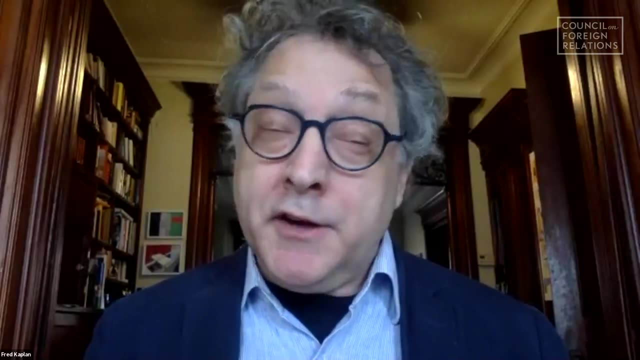 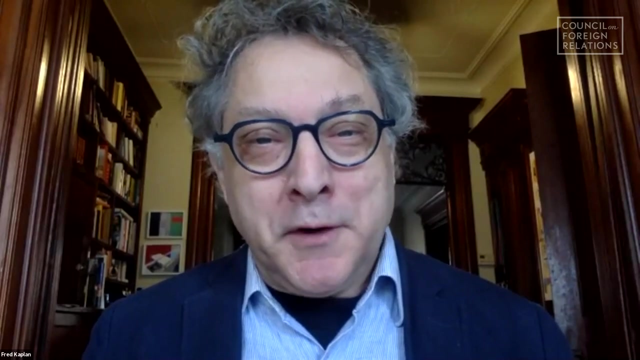 but very close to it. And yet you know, the Soviet Union has actually had even more of an impulse toward nonproliferation than we do. They've never provided nuclear materials to their so-called allies, because they feared their allies almost as much as they feared their enemies. 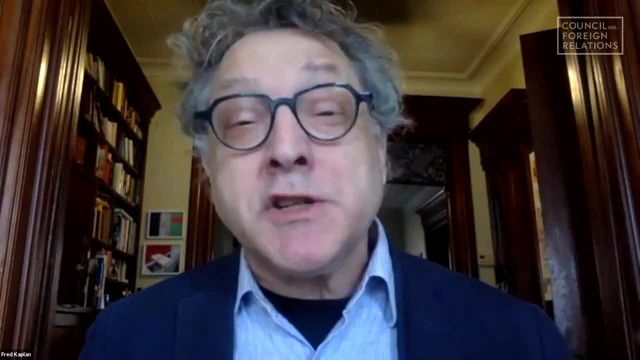 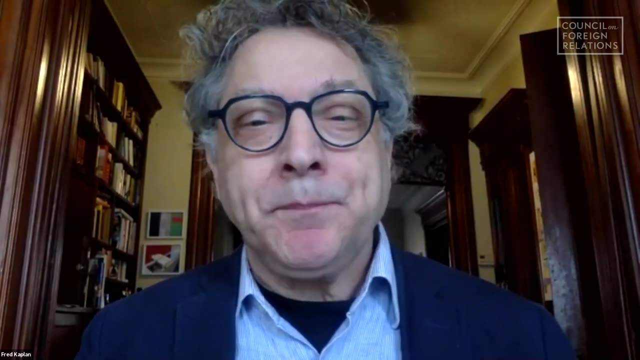 So there was a common, there was converging and even a common interest that the two of us had, And I think you know this holds some lessons for what we might do. now Things are quite hostile between the US and Russia. 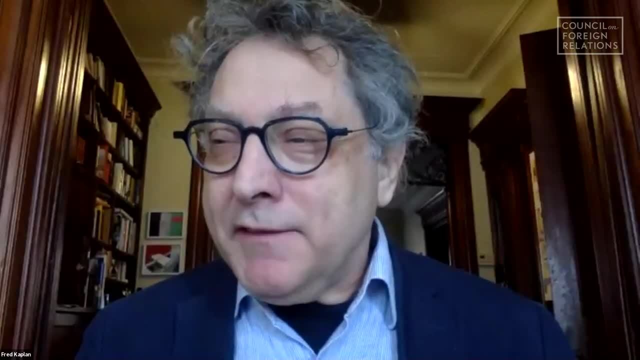 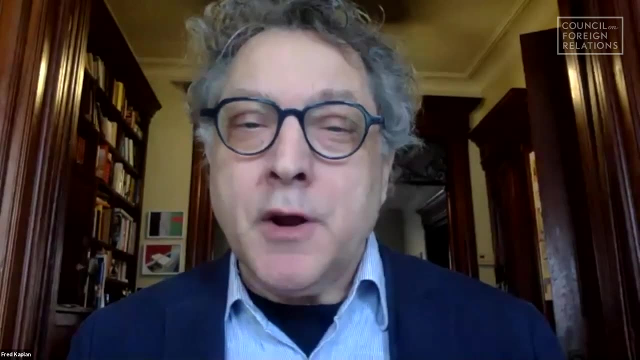 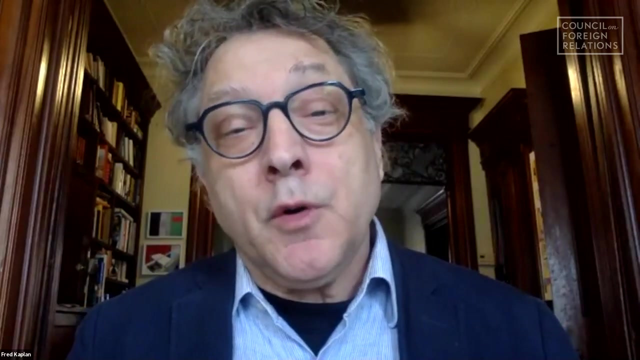 Russia, US and China, And yet even something quite as dramatic as a nonproliferation treaty was able to be negotiated at that time. And you know, one might wonder what less ambitious but still quite important accords might be developed now. 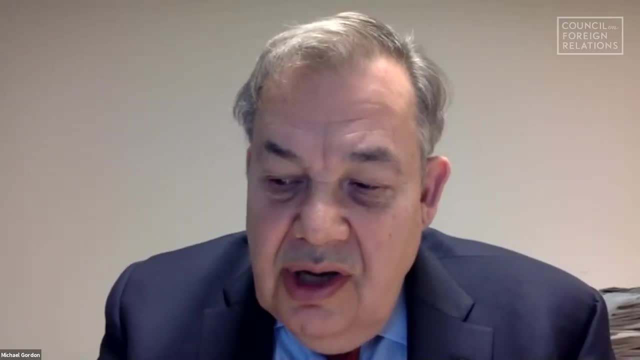 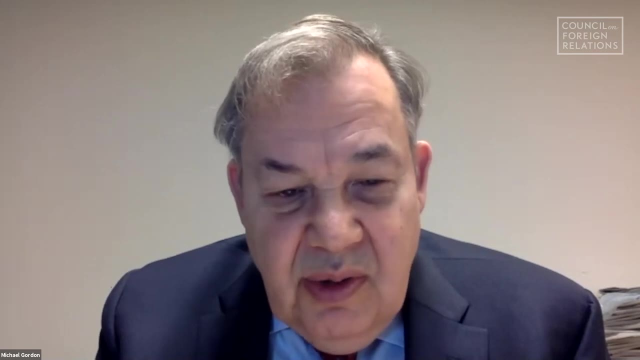 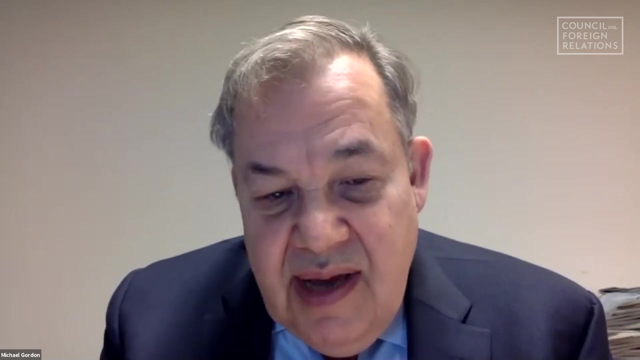 So, Bob, let me come back to you, Looking to the future. there's a review conference coming up at some point- Postponed, but still will occur. But what specific things do you think can be done to strengthen the NPT and the nonproliferation regime generally? 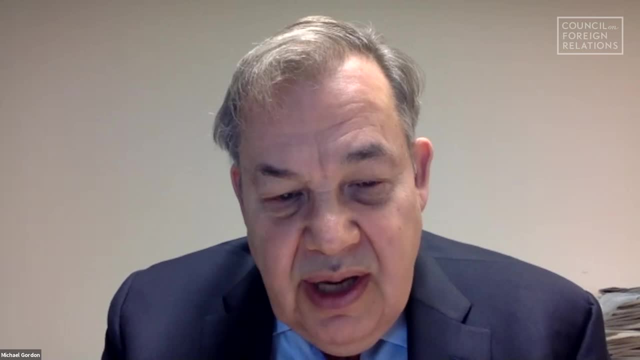 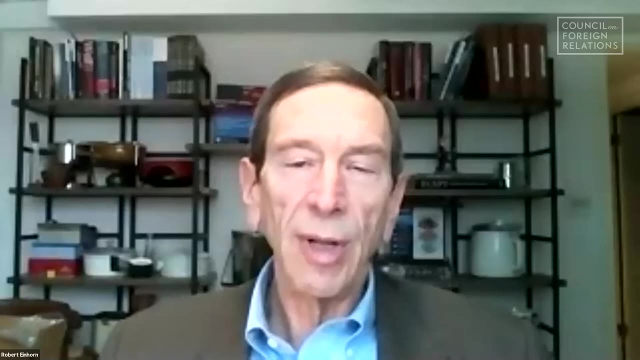 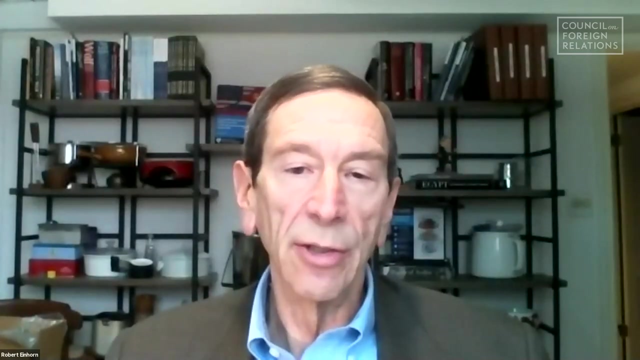 What are the things that you think might weaken it, And where does the review conference fit into this? Well, Michael, Iran is obviously a big challenge. If there is a tenth nuclear-armed state, many people fear it's going to be Iran. 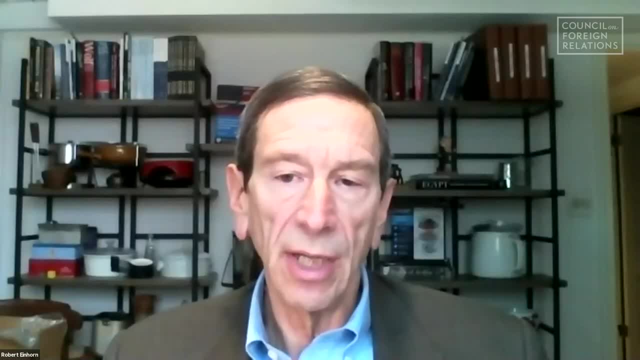 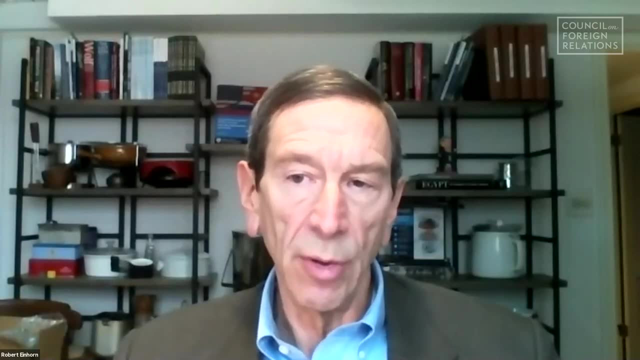 With the erosion of the Iran nuclear deal, Iran is building up its nuclear capacities again. So the Biden administration is going to have to address that problem and pursue a follow-on negotiation to try to extend some of the expiration dates in the JCPOA. 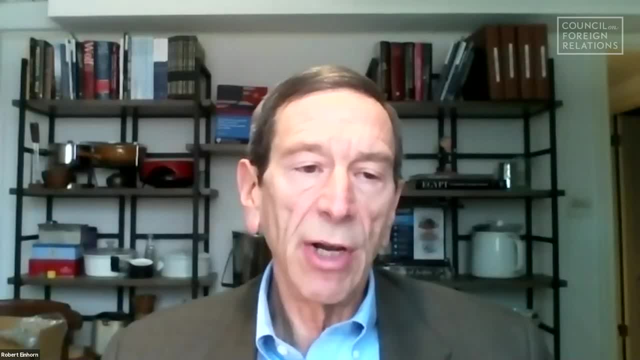 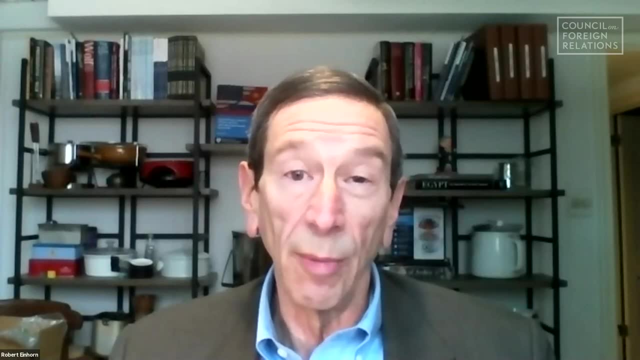 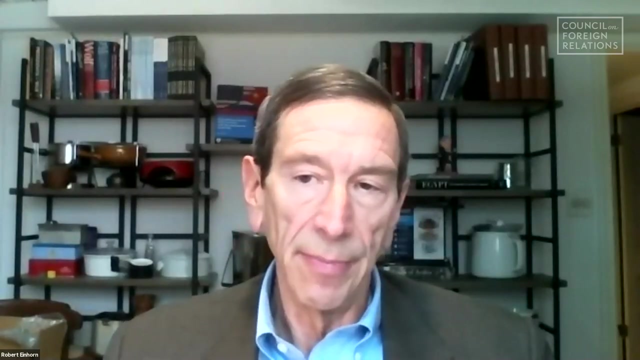 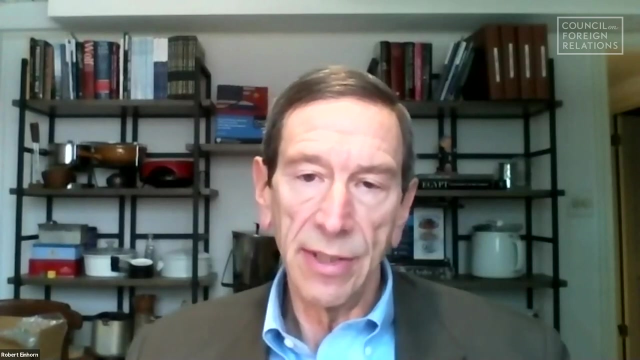 You know, Saudi Arabia, The Saudi crown prince, has said that if Iran gets nuclear weapons, his country will match them And others in the region could eventually follow suit. Turkey is a question here. So I think, dealing with the Iran problem and preventing Saudi Arabia from acquiring the technologies, 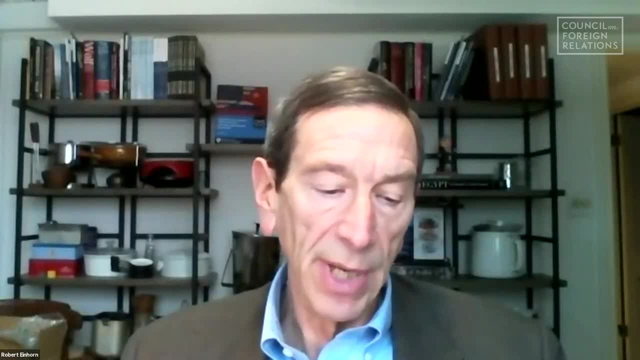 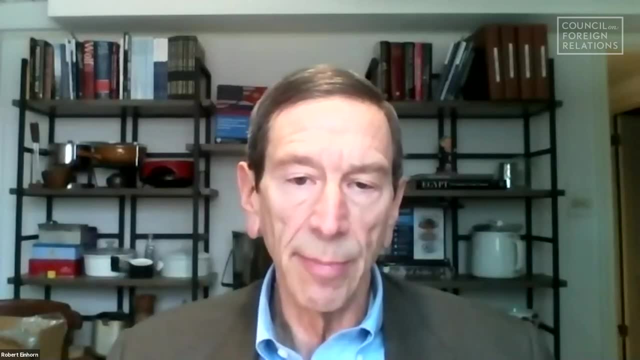 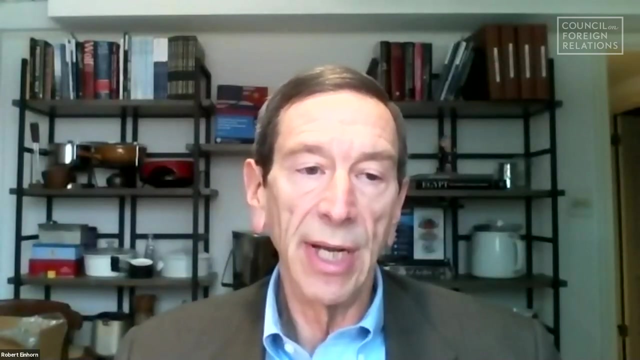 to pursue nuclear weapons. especially enrichment, should be a high priority. And then in Northeast Asia you have growing North Korean nuclear and ballistic missile capabilities. You have China's regional assertiveness, And they may be prompting South Korea and Japan to reconsider their decision to forego nuclear weapons in the past. 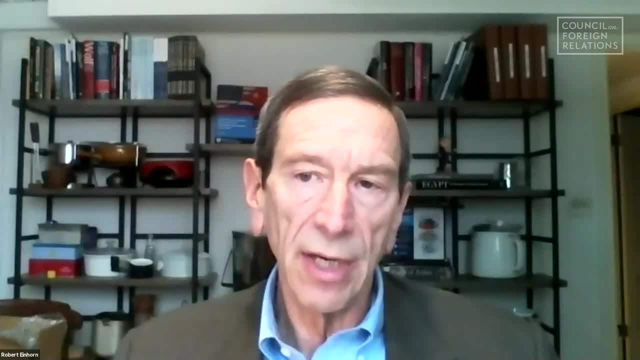 And I think in this connection, the credibility of US security assurances is very important And I think President Trump's transactional approach to alliance commitments has raised concerns on the part of America's allies about US security assurances. So a key element of nonproliferation actually. 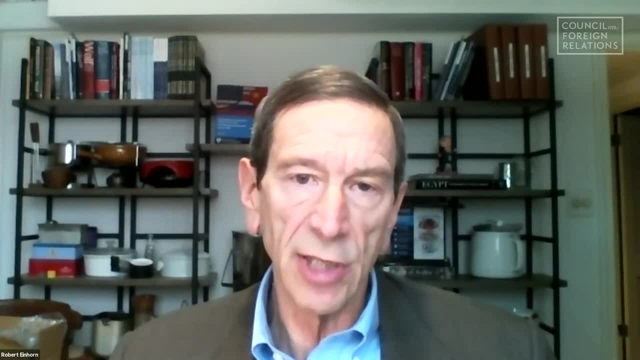 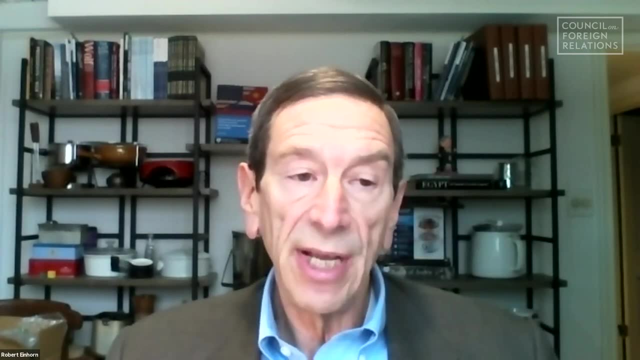 is to reinforce US commitments, especially the US extended nuclear deterrent. You know, I think, strengthening the IAEA safeguard system- this is something that Lisa and Laura know a lot about- and making the additional protocol of the IAEA universal standard. for NPT verification will be critical- Working together with Russia and China- Laura mentioned this. we used to be partners with China in dealing with North Korea, partners with Russia in dealing with Iran. That's more difficult now. That has to be restored. 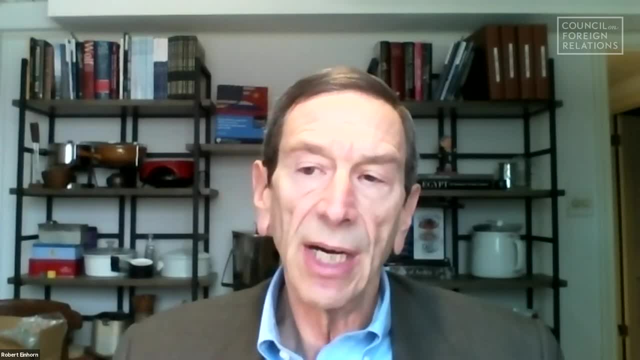 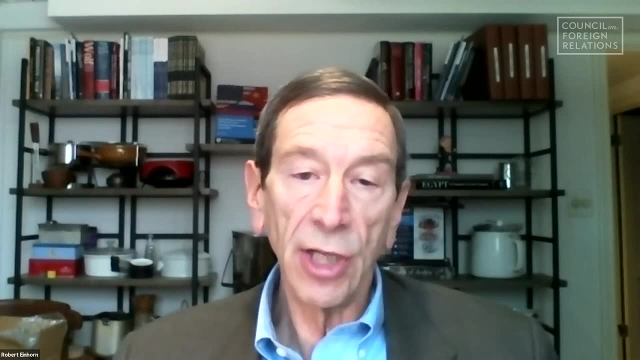 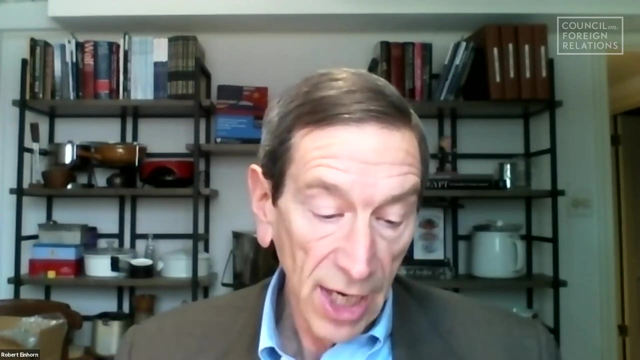 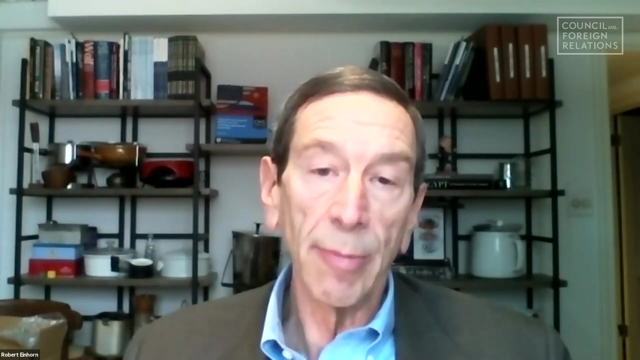 The illicit procurement networks have become much more sophisticated. We need to strengthen national and international interdiction capabilities to prevent these technologies from going to countries that want to have a nuclear capability. And, of course, we have to try to rejuvenate arms control. 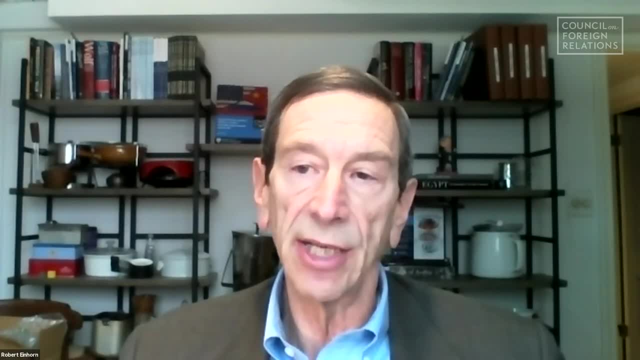 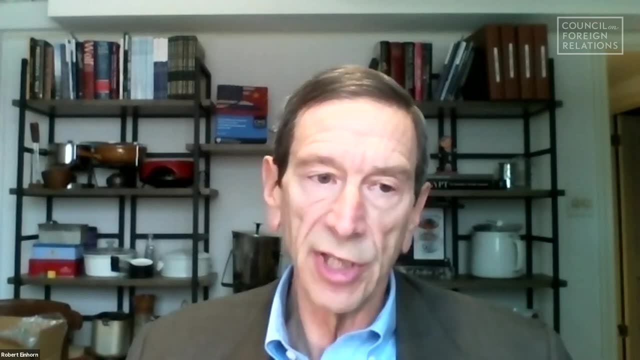 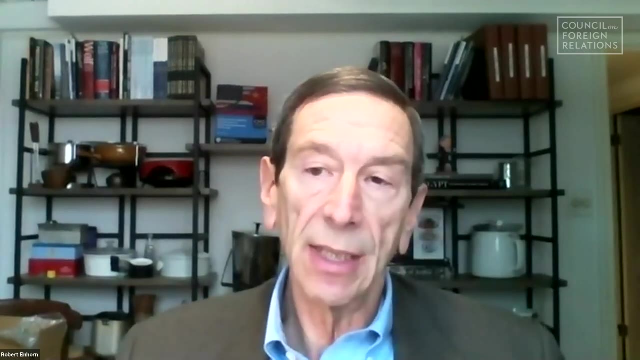 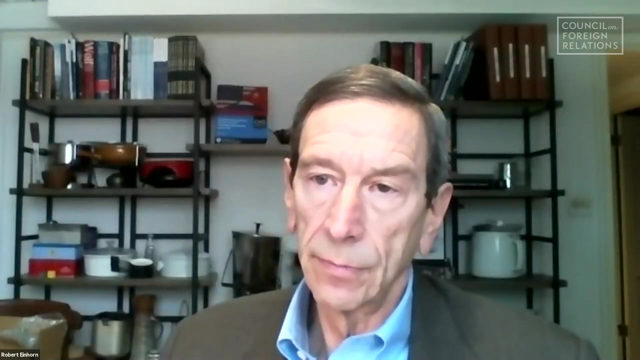 You know there have been setbacks recently: the termination of the INS, the UNF Treaty. Hopefully a new start will be extended for five years once the Biden administration takes over. But there are big challenges ahead and it's going to take concerted action to address them. 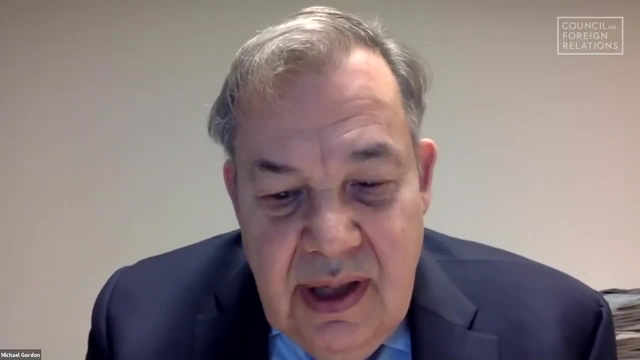 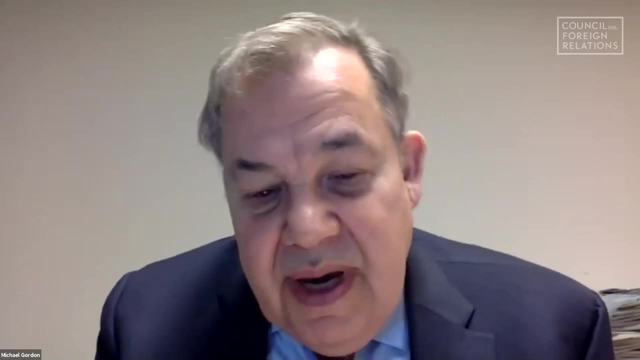 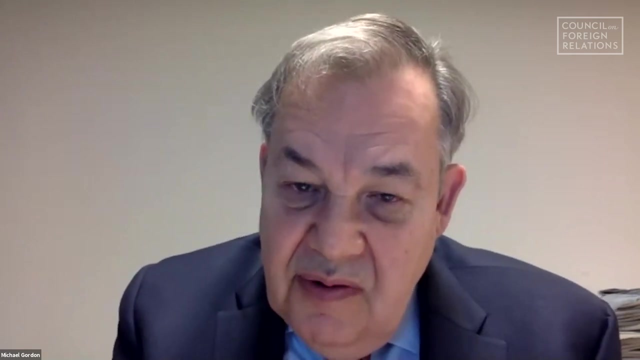 We have just a few minutes before we turn to questions from all the people viewing this now. Does another member of the panel want to weigh in? Anybody else have any other recommendations or suggestions for specific steps to strengthen the NPT over, let's say, the next decade? 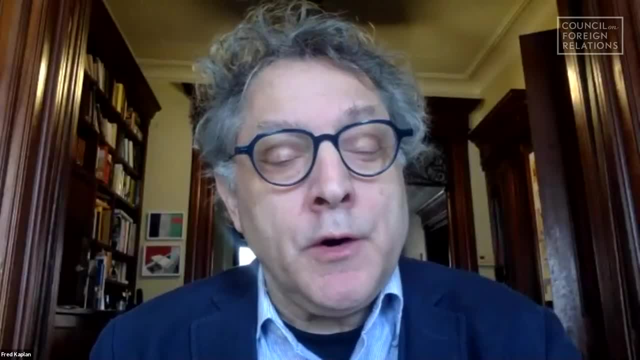 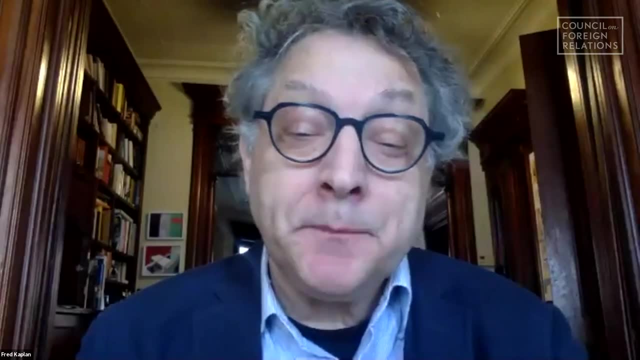 Well, one thing you know: if you look at the literature back in the early 60s there were forecasts that by the year 2000, there would be 20, 25 nuclear states. There were certainly nearly that many with the technical capability. to get there. The NPT was one reason why this was cut off. Another was that the network of alliances that both the United States and the Soviet Union had at the time. Well, in the case of the Soviet Union, it was clamping down on any effort. or even thoughts that the Warsaw Pact allies would have on getting their own nuclear weapons. In our case, it was providing assurances. you know, the nuclear umbrella As this becomes eroded, as it became eroded under Trump, and it's going to take some time. to restore these assurances. that was when, you know, you started having countries like Japan and South Korea thinking: well, I don't know if I can rely on the United States, Maybe I have to go my own way. So networks of either clamping down. 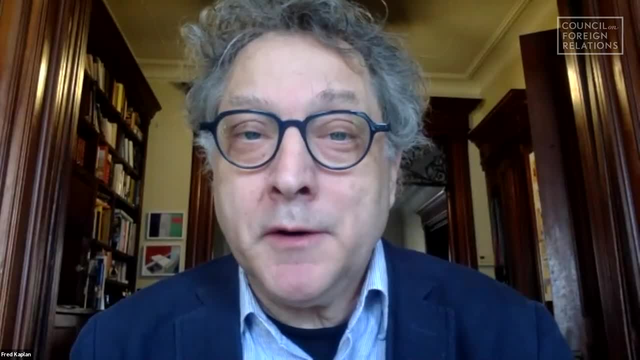 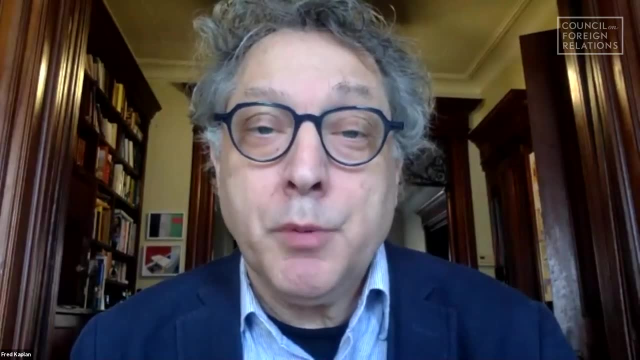 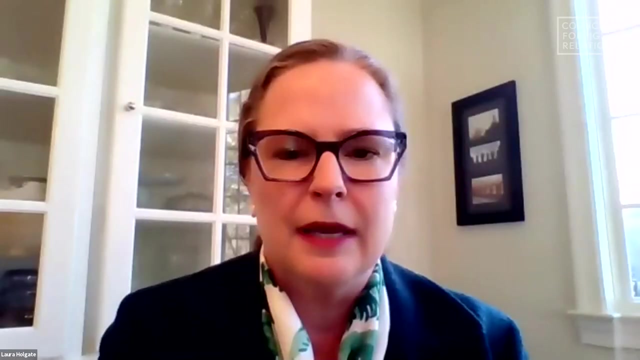 or assuring security, which have nothing to do with technological security, which have nothing to do with the international aspects of the treaty, but just the underlying geostrategic elements are important to emphasize. Okay, I think it's also important to improve the health. 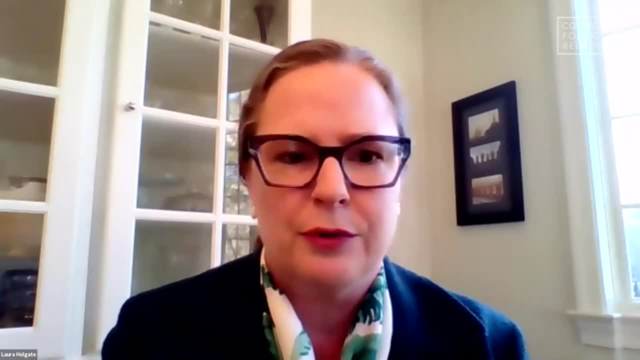 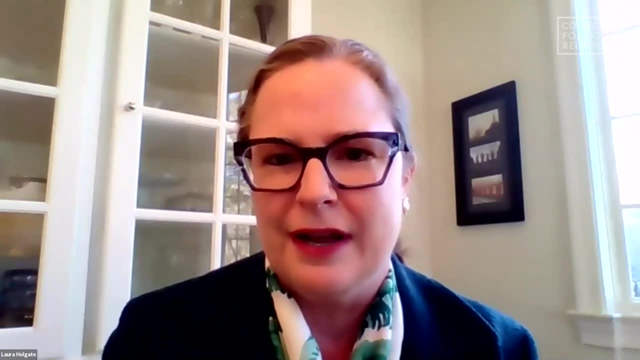 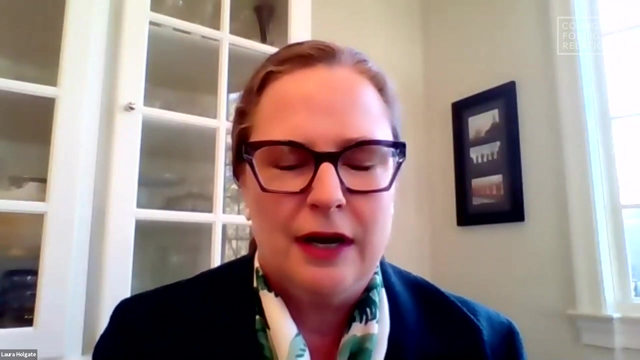 of the International Atomic Energy Agency. It's been on a zero real growth budget for well over a decade, as the expectations of the international community on them has only increased And, as Lisa pointed out, to the degree that we have a growth of nuclear energy. 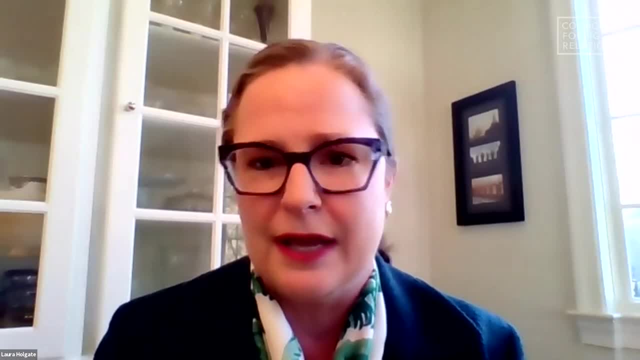 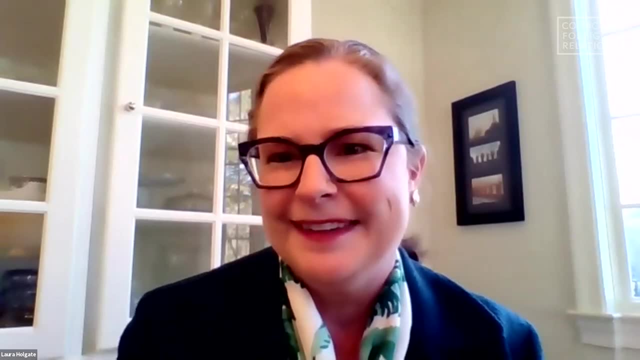 in countries that haven't had it before, of new types of reactors that have the potential to be more secure and more safeguardable by design, but only if we make them that way. they won't automatically be like that. The agency is going to be asked to do more and more. 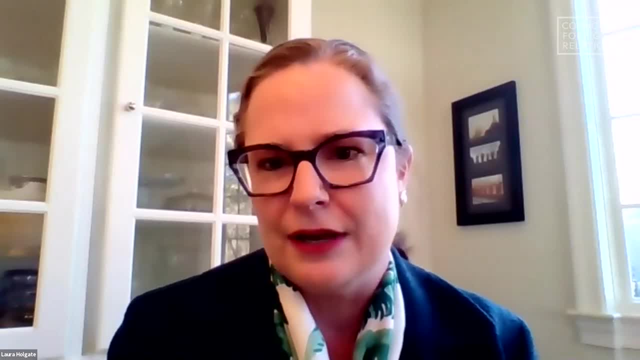 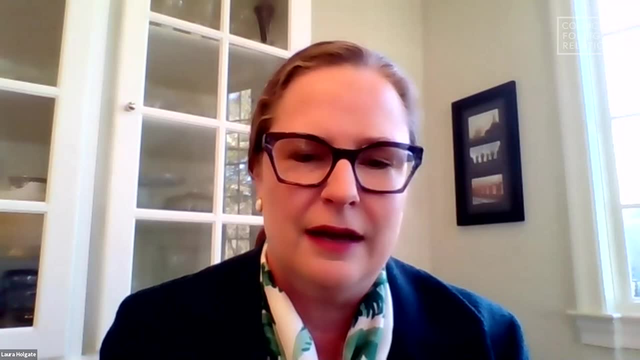 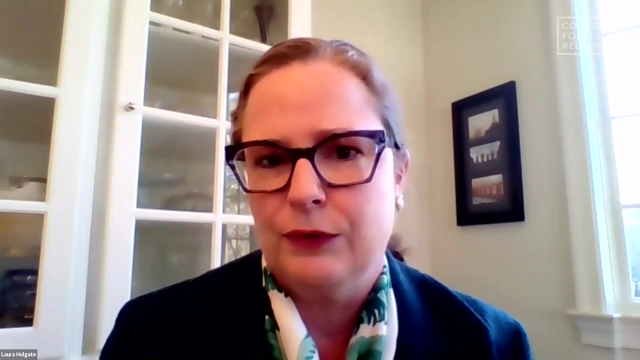 And so getting a recreating the international consensus that allows it to have the people, the technology that is needed to sit underneath its legitimacy, will be critical to the NPT's future success. Michael, can I just add a couple of quick points? One thing that really needs to be done is to do something about the NPT's withdrawal provision. If a country legally withdraws from the NPT, its safeguards, its IEA safeguards, will automatically lapse and it will be legally entitled to use the equipment. 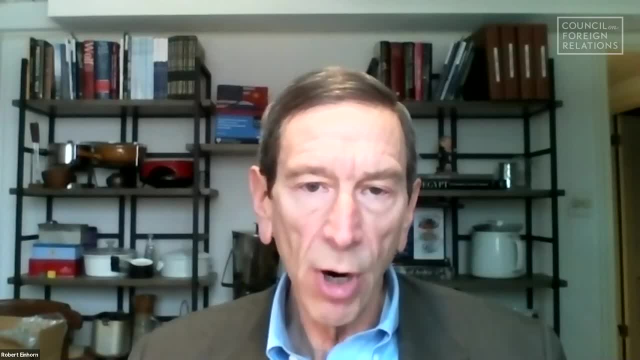 the technology, the facilities acquired while an NPT party to pursue nuclear weapons. This needs to be fixed. There have been proposals over the years to fix it. It hasn't been done. Another thing that needs to be done is that today, nuclear exporting countries they have a strong incentive to make reactor sales And there's a real risk that in the competition to make those sales, including to places like the Middle East, that they will relax the conditions that they require their potential customers to accept, including with respect to adherence. 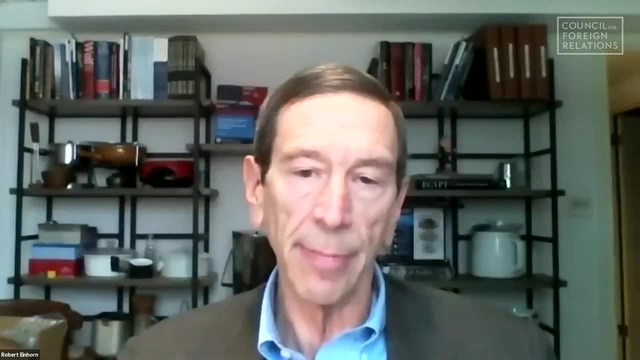 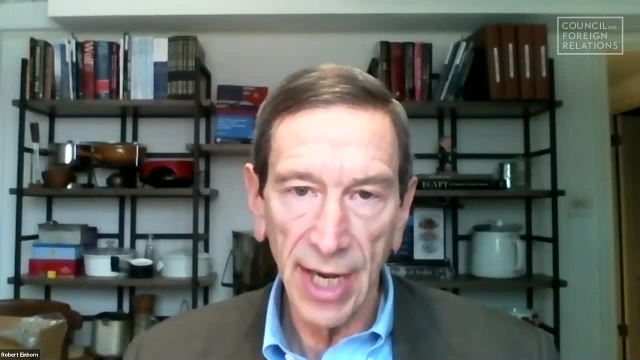 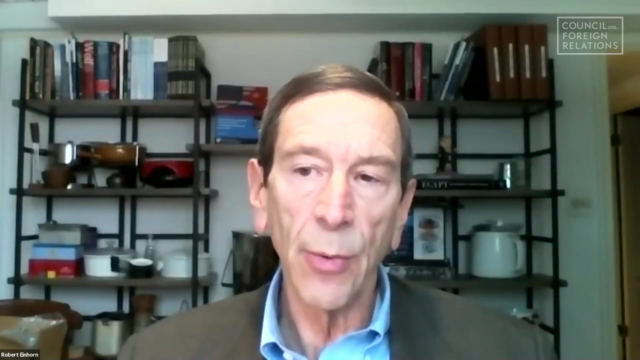 to the additional protocol, including with respect to the pursuit of enrichment or reprocessing capabilities. Groups of nuclear exporting countries should get together, not just in the nuclear suppliers group, which is multilateral, but a small group of them, and to agree to strengthen. 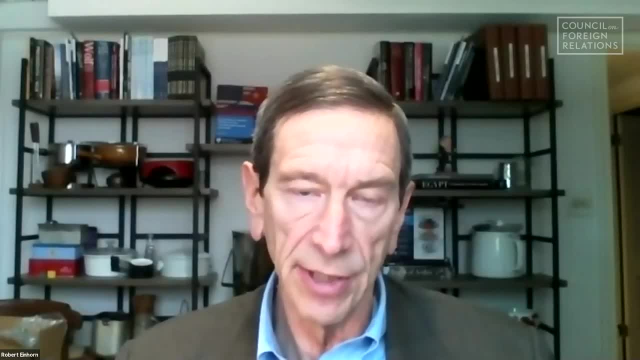 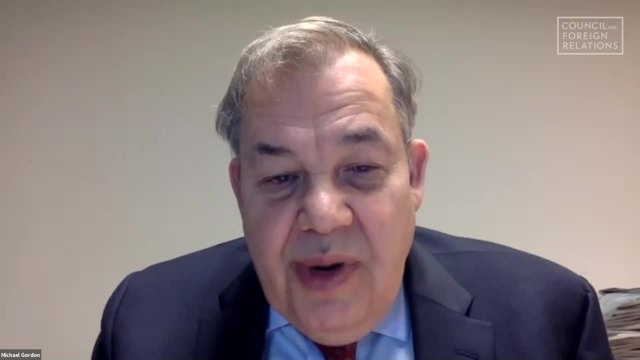 the conditions of nuclear export, especially to the Middle East. Okay, At this point, just to make sure our members get a chance to ask their own questions, we're going to open it up to all members to join the conversation. And a reminder: 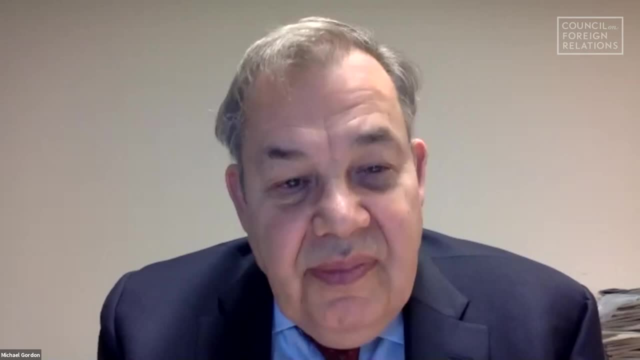 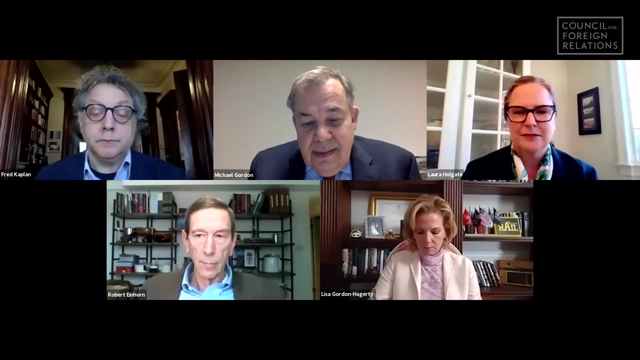 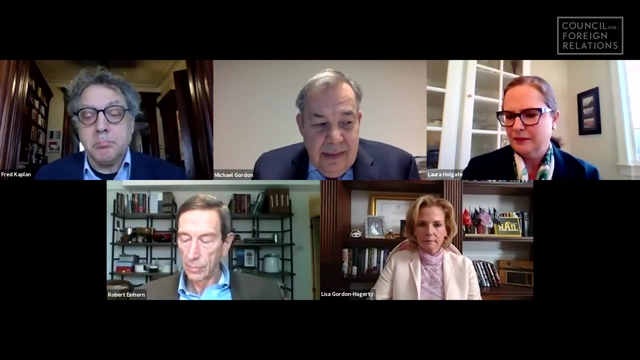 this is all on the record And now our CFR staff's going to remind you how to join the question queue. We'll take the first question from Annalise Riles. Hello, thank you very much for this wonderful discussion. I'm Annalise Riles. 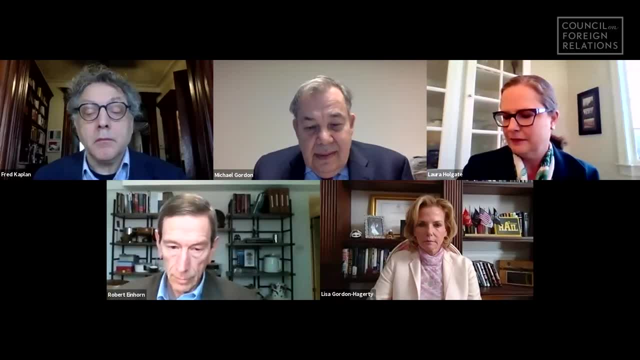 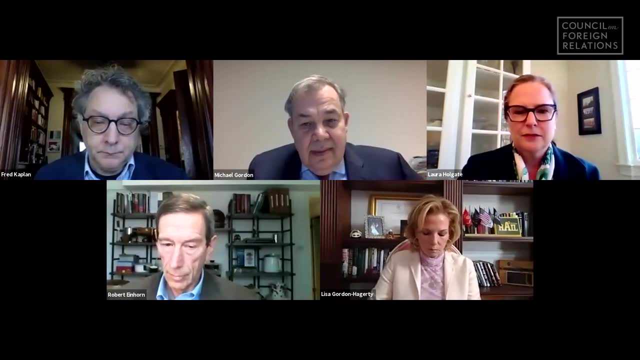 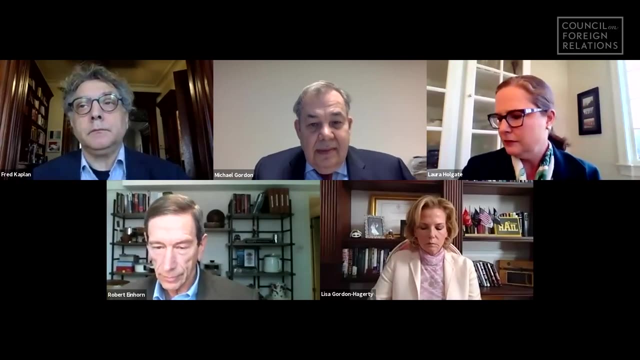 Director of the Buffett Institute at Northwestern University. On January 21st, a new nuclear ban treaty will come into force. as you know, It takes a different approach and it's been brought into being by a different cast of characters. What are the implications? as you see it, 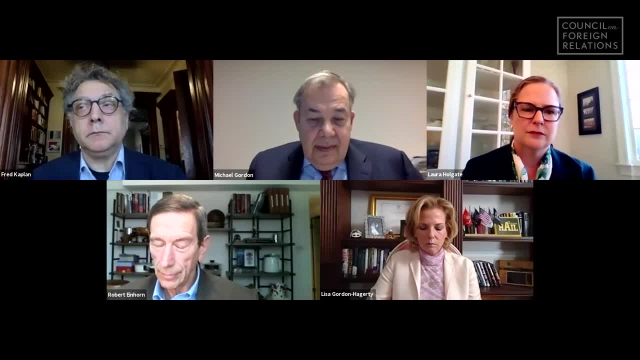 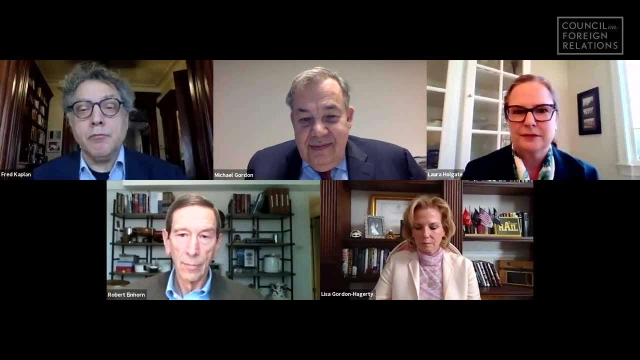 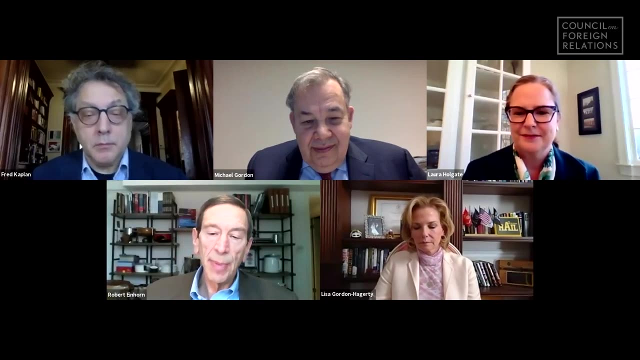 of this treaty for the nonproliferation regime and what should be the approach to it for the Biden administration. Thank you, Who wants to take that? Go ahead, Annalise the TPNW, the treaty you referred to. 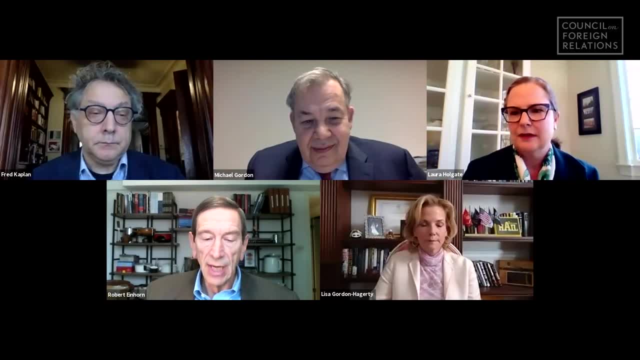 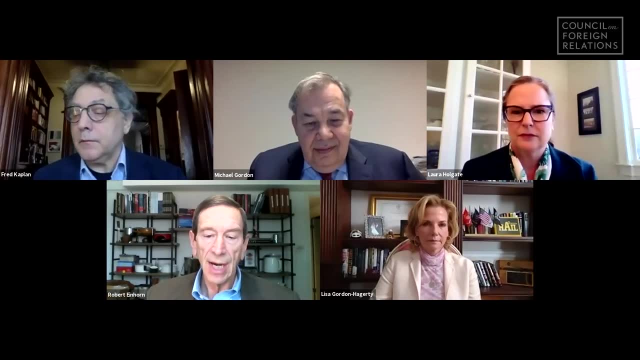 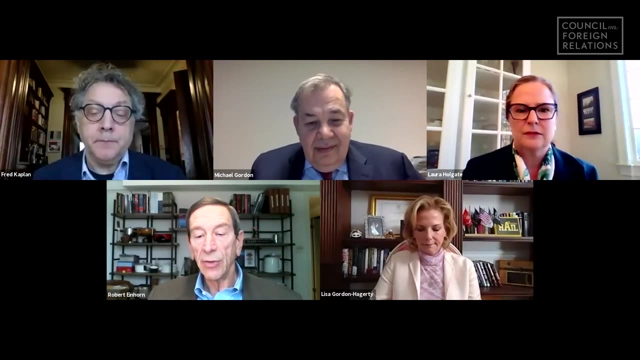 is going to enter into force very, very shortly. I don't think the proponents believe that it's going to encourage further steps toward nuclear disarmament. I doubt that it's going to have that practical implication. It will enter into force for over 50 states. 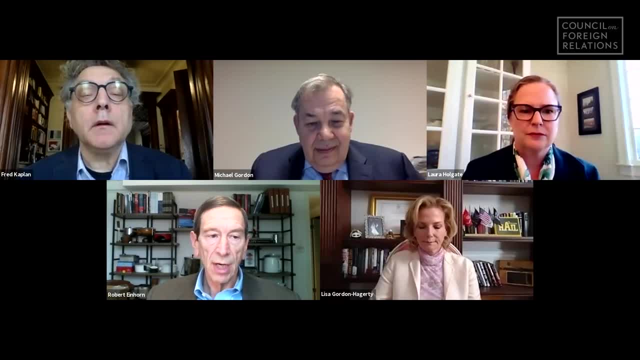 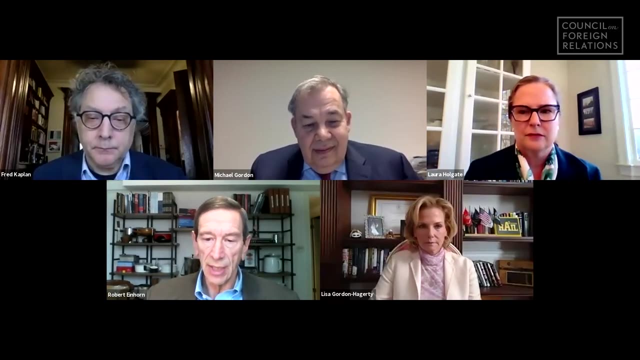 but none of those states have nuclear weapons. None of those states have security guarantees from the United States that depend on nuclear weapons. My own view and the view of the nuclear weapons states who oppose the treaty is that the best way to pursue nuclear disarmament 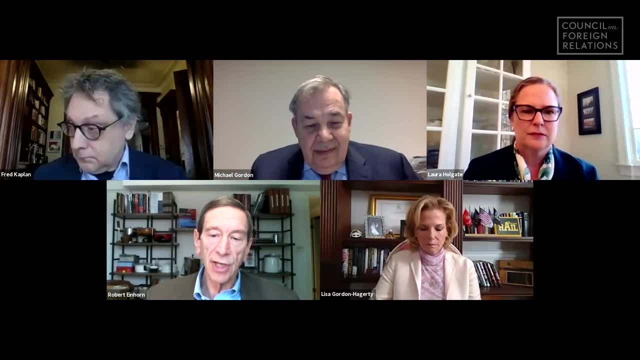 is through a step-by-step approach based on what's permitted by international security conditions And unfortunately today those conditions are very good. But sooner or later they're improved and we can get back on the track to further nuclear disarmament. But I don't think this effort. 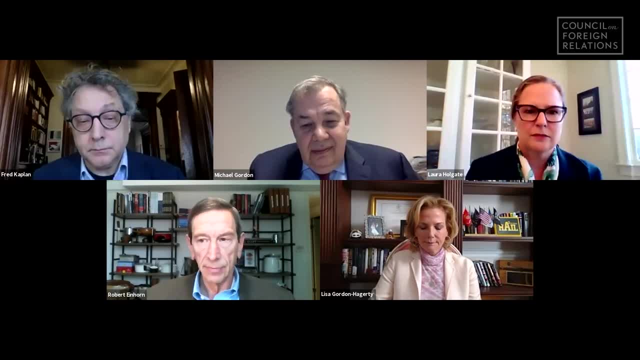 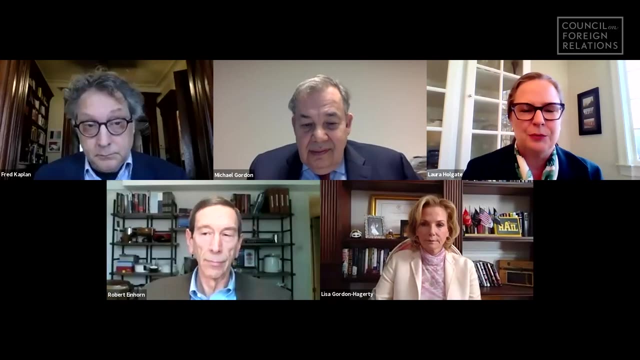 is going to have much effect on nuclear disarmament. I think the Treaty on Prohibition of Nuclear Weapons is really kind of a cri de coeur from the rest of the non-weapon states in protest to the lack of progress on nuclear disarmament. 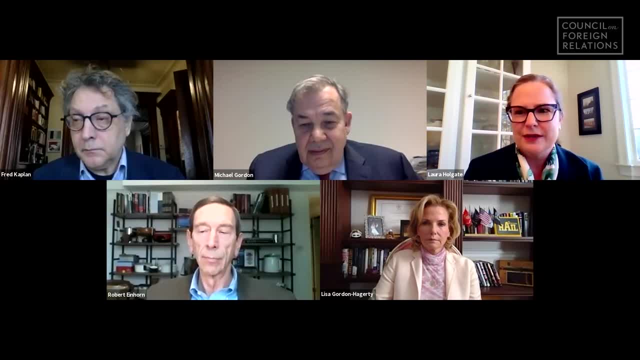 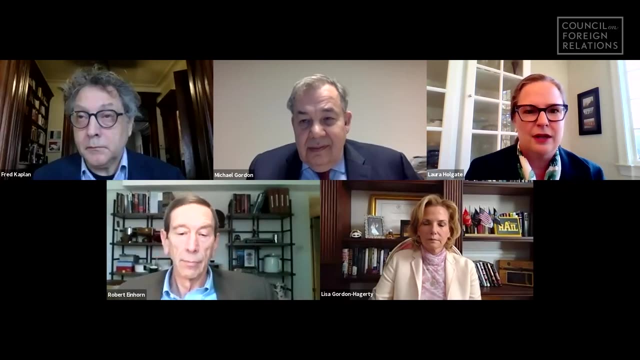 And so I think it's important that it be taken seriously, but not necessarily literally as a kick in the pants to get US and Russia back to the negotiating table and unlock the lack of progress on Article 6. Reforms that Bob very rightfully pointed out. 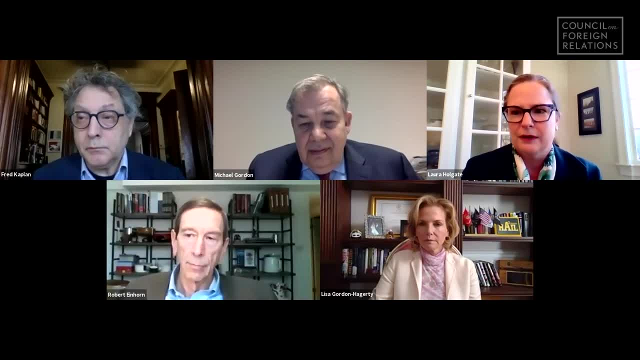 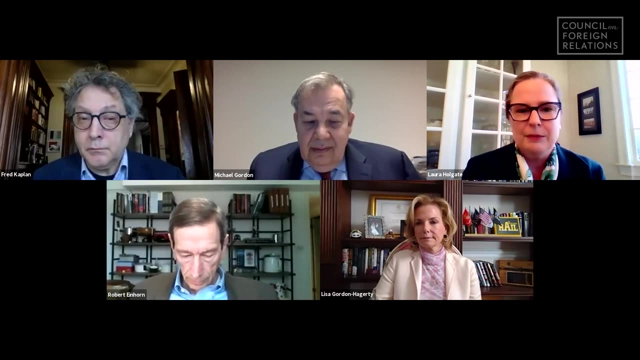 to the NPT are not going to be possible if the countries that have weapons are not seen as carrying out their work under Article 6.. So I don't think it'll change the legal or behavioral landscape very much for those who are members of it. 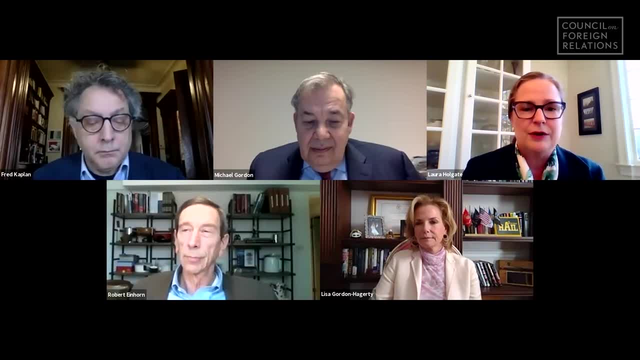 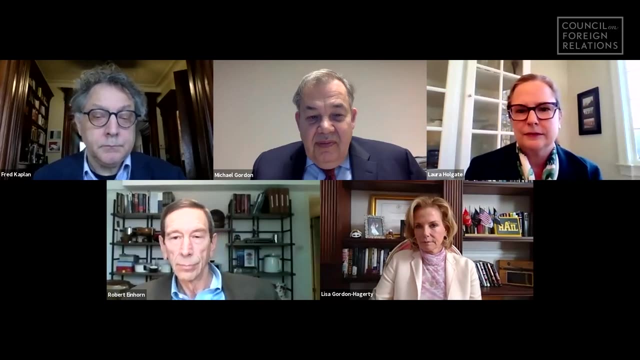 But I do think that the weapon states ought to take the disgruntlement that it reflects quite seriously and return to first bilateral and then, you know, at least five-part arms control negotiations. Let's move on to the next question, so we can get some. 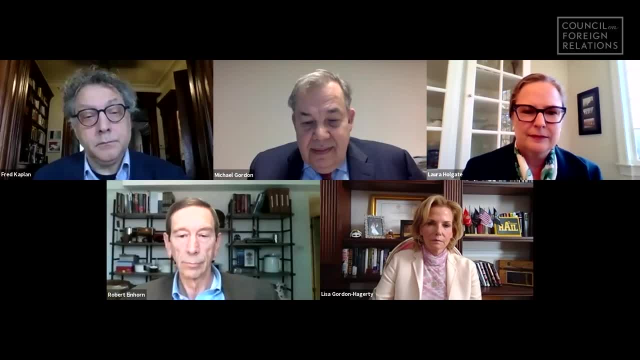 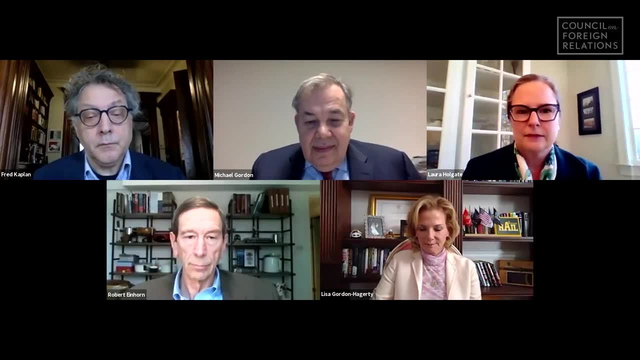 I think there'll probably be a bunch out there. We'll take the next question from Christopher Ford. Hi, Hopefully you can hear me. Excellent, Very good, My name is Chris Ford and I actually have no affiliation whatsoever at this point and lots of time on my hands. 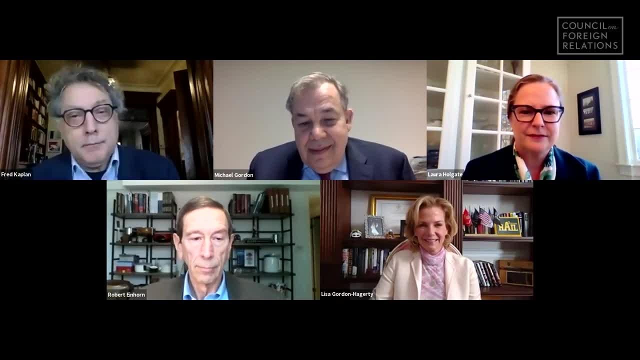 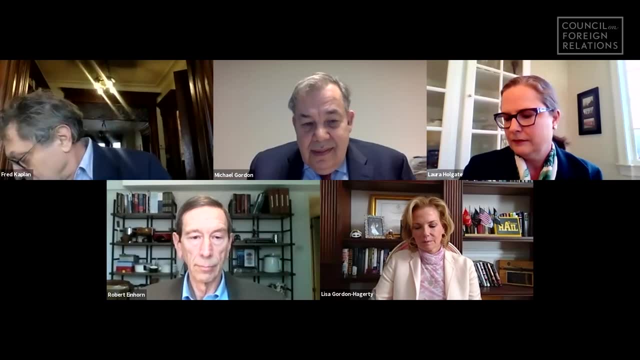 Thank you guys, all of you, for this great discussion. A quick, very quick comment and then a quick question, if I might. The comment is actually to add a bit of gloss onto what Fred said about the origins of the NPT. 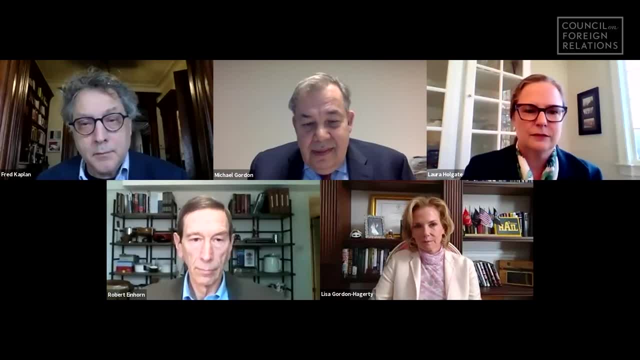 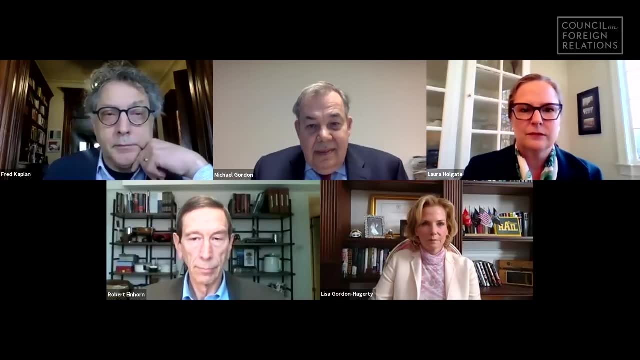 And I guess I would point out that there are some origins that go back even further, at least as far as 1961, at the UN General Assembly, with something called the Irish Resolution, which established what in effect became the two core principles of the current treaty. 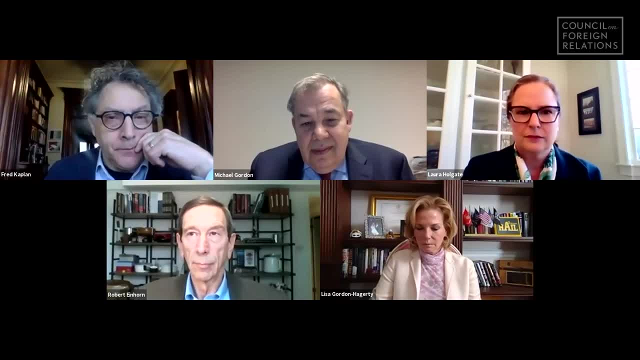 and still are all these years later. First of all, the idea that those who have weapons shouldn't spread them And, secondly, the idea that those who do not have weapons shouldn't try to get them. And we see both of those today. 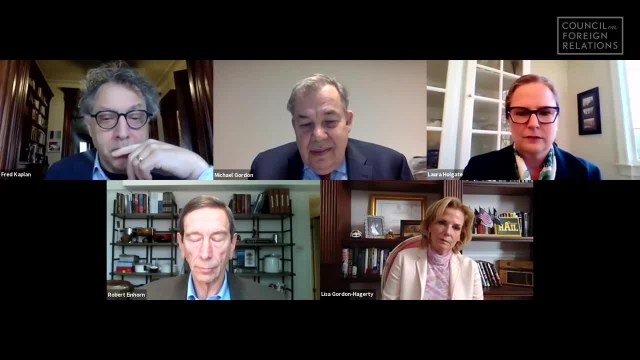 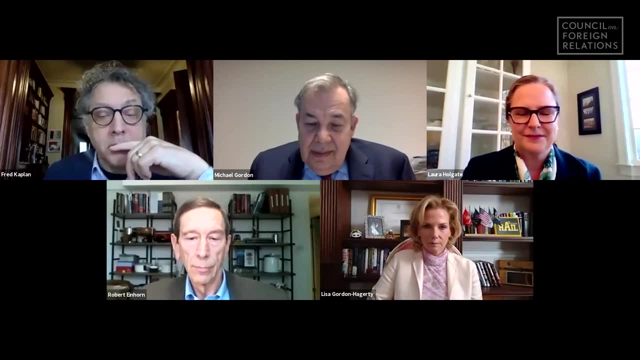 in their modern incarnation in Articles 1 and 2 of the NPT. So there's a fantastically long genealogy, even earlier than the point that we were discussing earlier. My question has to do with the rescheduled NPT review conference. 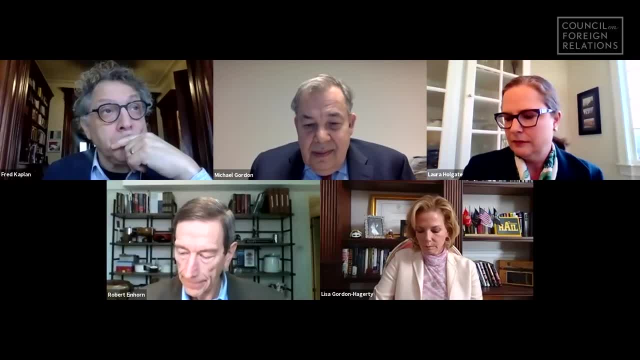 which is, I guess, now on for August, and what it might be possible for the parties to agree to at that event. The last time there was an agreed final document at a review conference was in 2010,, when Joe Biden was vice president. 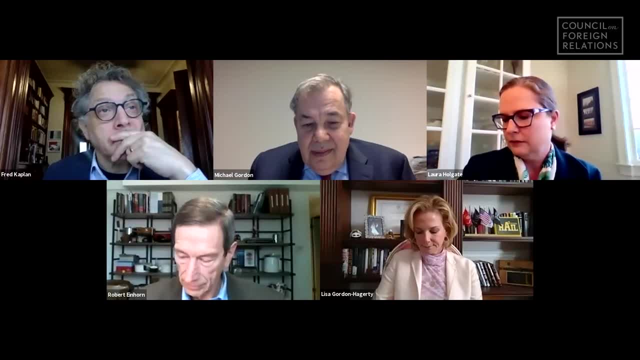 and everyone, including the US delegation there, agreed, among many other things, to implement something called the 13 practical steps that had been agreed as early as 2000 at the review conference, which means that the US delegation and all the other parties at the NPT 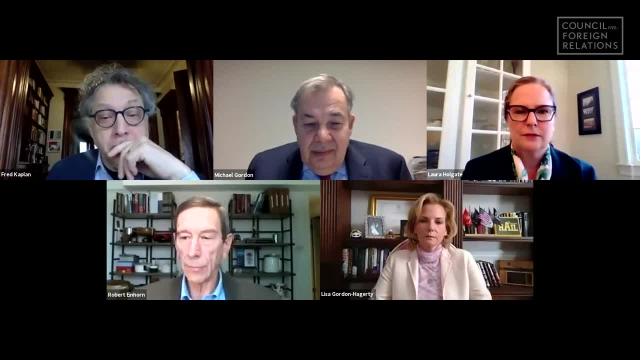 in 2010, agreed to implement start two, to negotiate start three, to implement the trilateral initiative and to strengthen the ABM treaty, none of which actually existed at the time. they all agreed to do these things. I guess my question for the panelists is: 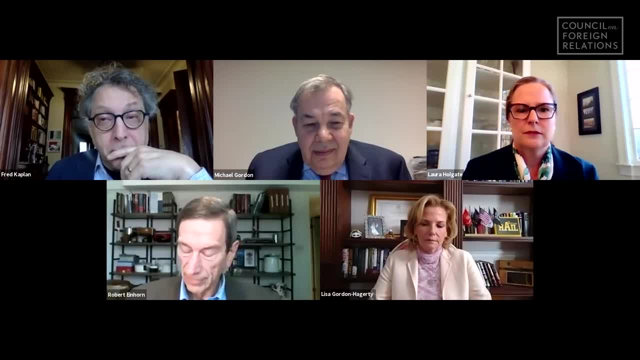 do you all think that the parties might be able to agree upon something in August of 2021 that actually reflects the 21st century rather than the agenda of the 1990s? And, if so, what would that agreement look like? Thanks very much. 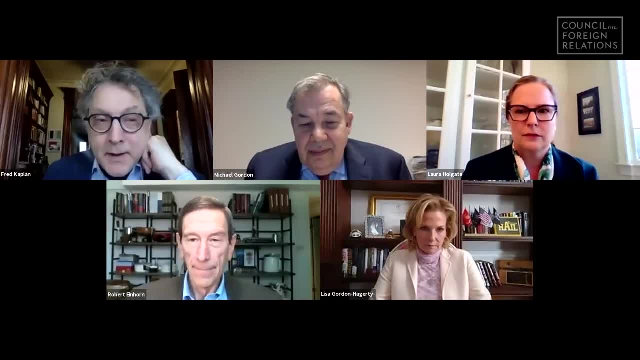 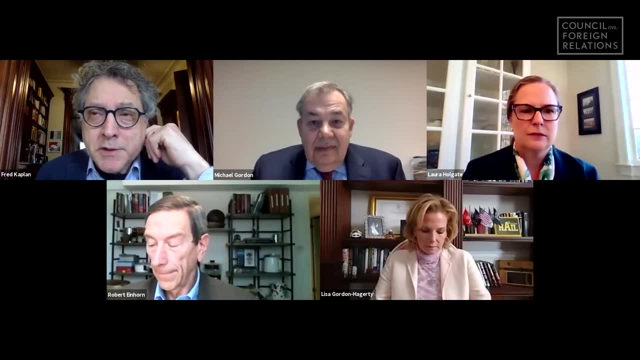 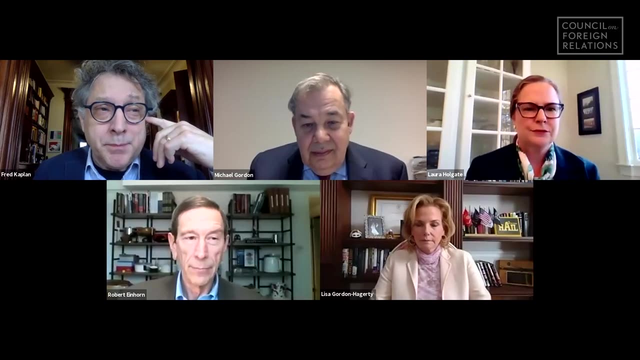 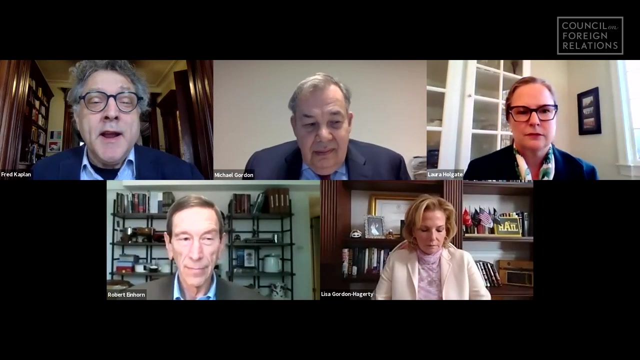 Well, I would say the idea of a start three. the idea of start three, when people first started talking about it, was to address- And I think, certainly post annexation of Crimea and incursions into Ukraine, I think even people in the Obama administration. 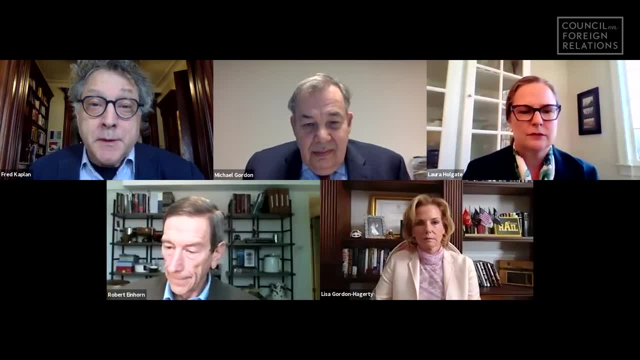 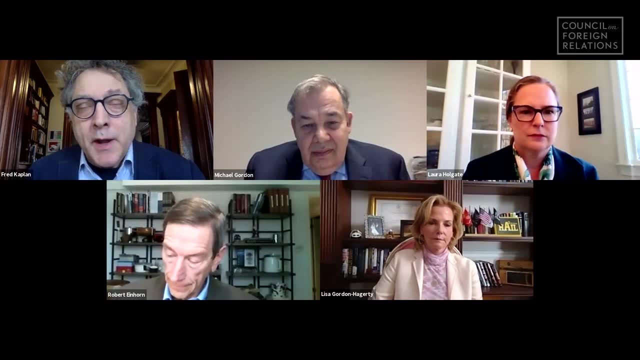 were conceding that this just wasn't going to happen. This wasn't going to happen. I think that Russia was not going to reduce its theater nuclear weapons in any significant way, any more than in the 1960s the United States would have reduced. 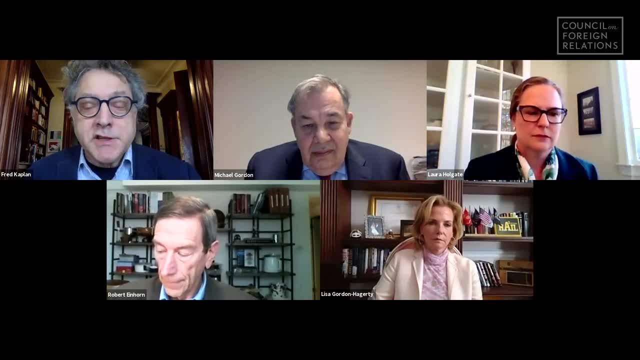 its some 7,000 theater nuclear weapons in Europe, which it saw as a hedge against what was seen as Russian conventional superiority in Europe. So I think that's probably not a Anything that's going to happen. I think maybe one thing to focus on. 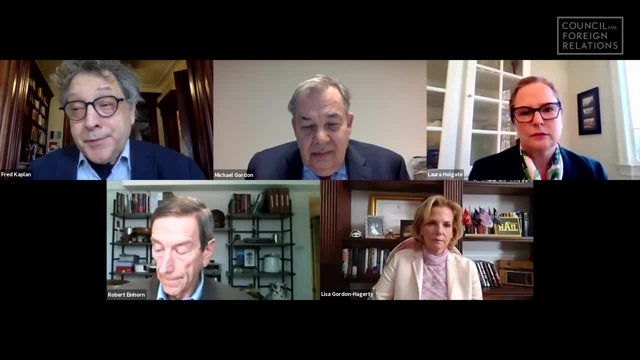 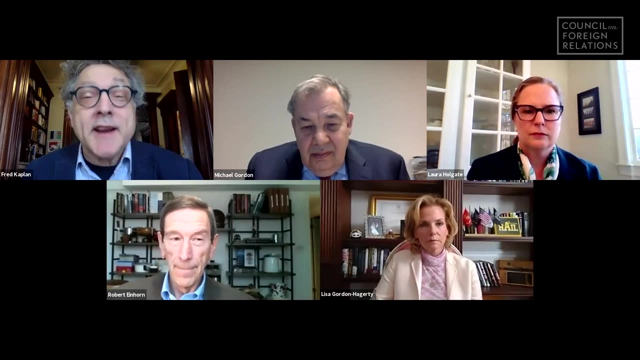 while it's very difficult to focus on anything else, are things related to just broad confidence building measures, having to do with And just restoring arms control talks in general. I would say that for the first decade of nuclear arms control negotiations, far more important than anything. 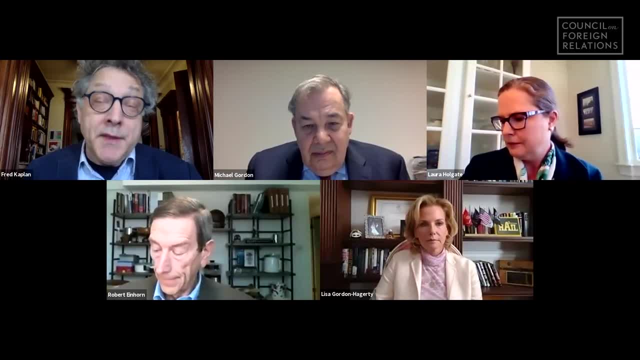 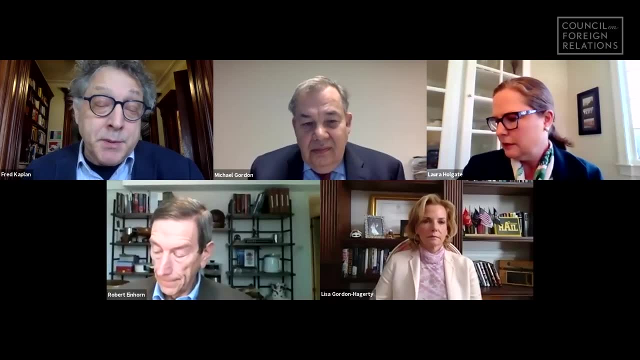 that was actually accomplished in the treaties, except maybe the ABM treaty, which was quite significant. The more important thing was just having Russian and American officials and diplomats sitting around the table talking about something. Arms control was kind of a Something that they could talk about. 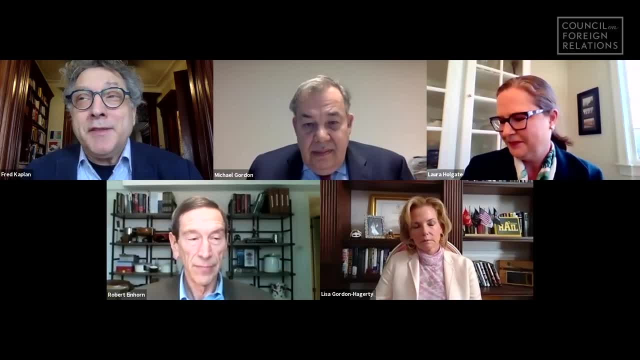 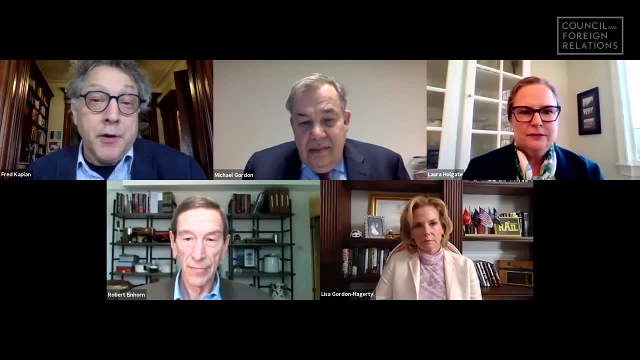 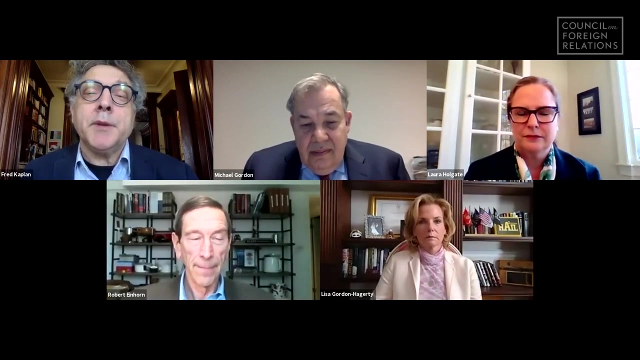 when it was politically impossible to talk about anything else. So I think it might be a valuable thing just to have diplomats sit down and figure out a next steps agenda, Which in itself could have more tangible effects immediately, Kind of a confidence building implications right away. 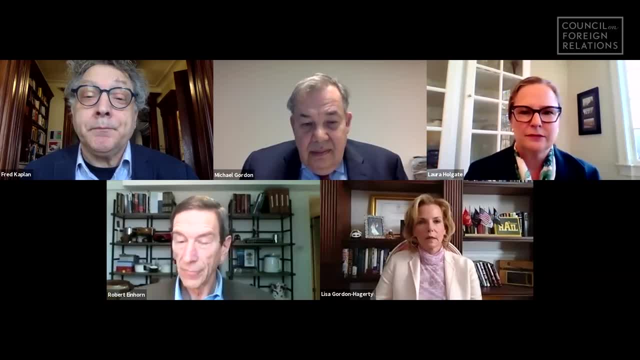 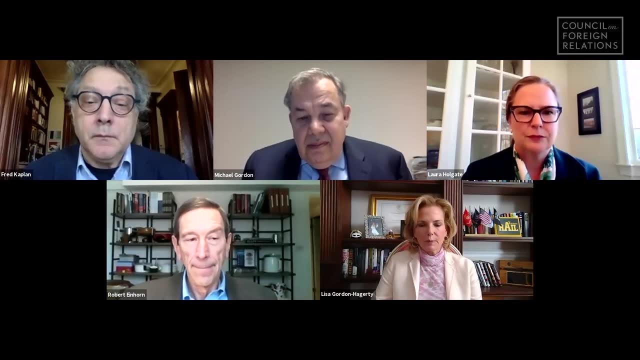 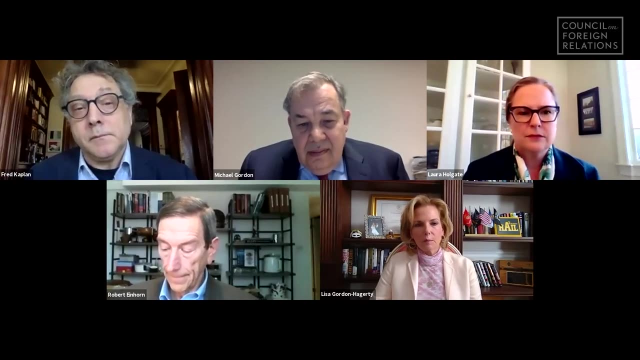 and more tangible ones down the road. And if I may add to that, Fred, those are great points Not to stray away from the NPT but in the New START negotiations that have been ongoing. I will tell you one of the things. 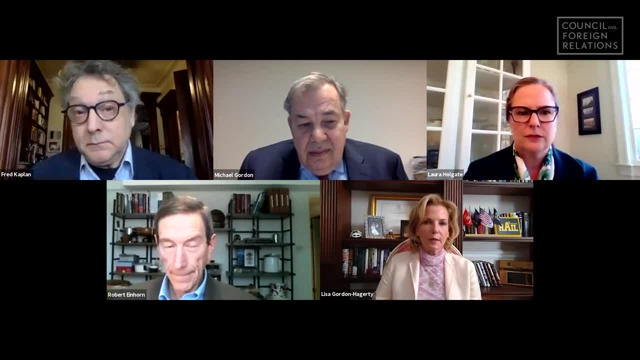 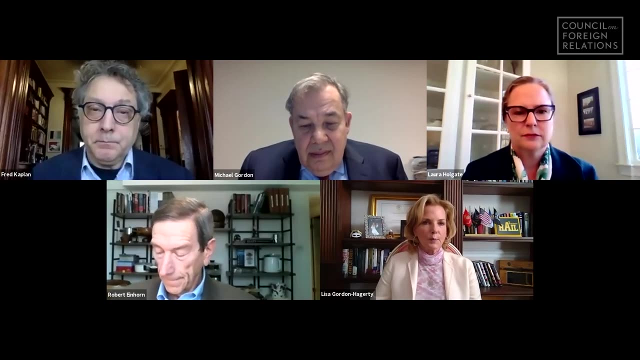 that I think was one of the biggest opportunities that we put on the table was confidence building measures with the Russians, And we have not seen that moving as quickly as we could. I think there are some opportunities, because we did have quite a robust New START opportunity ahead of us. 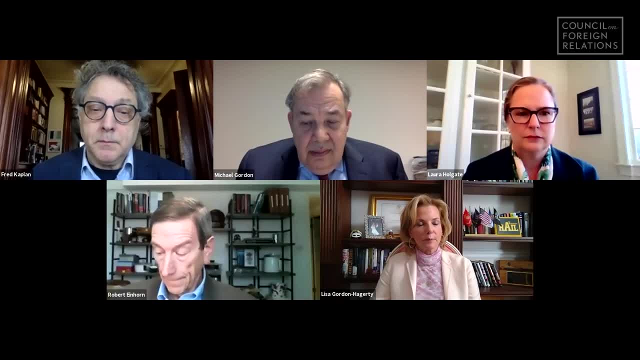 that was at least proposed by the United States as far as I'm concerned, And we were part and parcel of that from a technical standpoint, So in my previous capacity. But I would say that there are some obvious opportunities there at the RevCon where we can apply those. 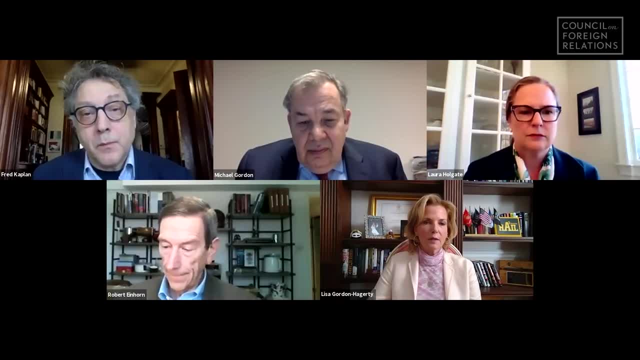 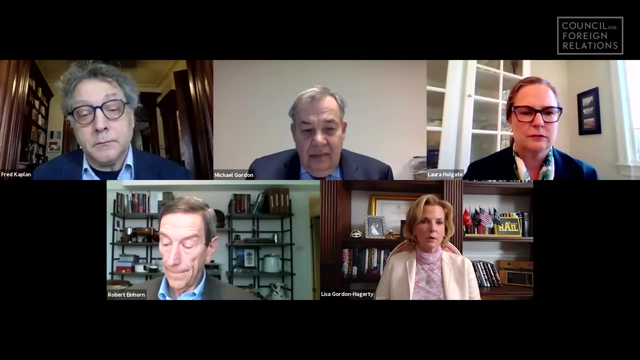 whether it's bilateral or multilateral. So I think there are some things. But just again, just to make clear, even with the New START negotiations, with the discussions with the Russians, the conversations, in my opinion, were more one-sided than they were coming back to the table. 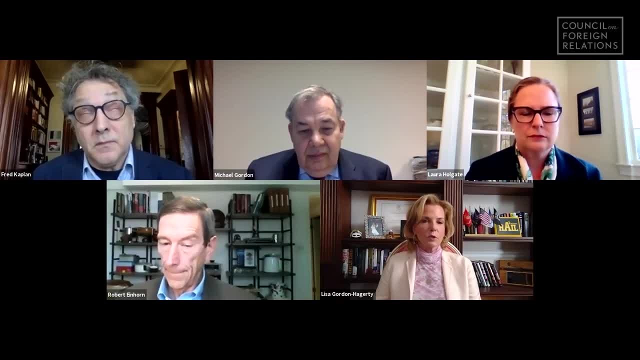 In fact, it was even as far as who the Russians brought for their negotiators. So I would like to see that too, And I think there are some opportunities there as we embark on the 21st century. in the next 50 years, or how many years? 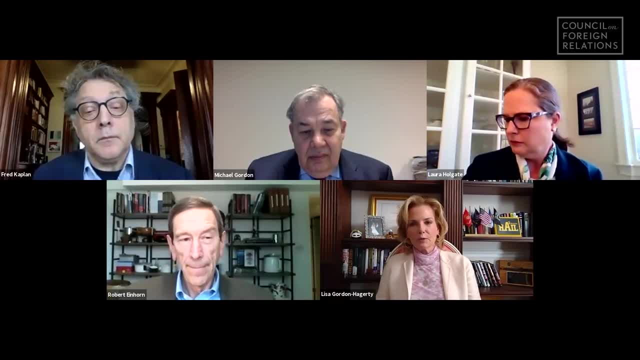 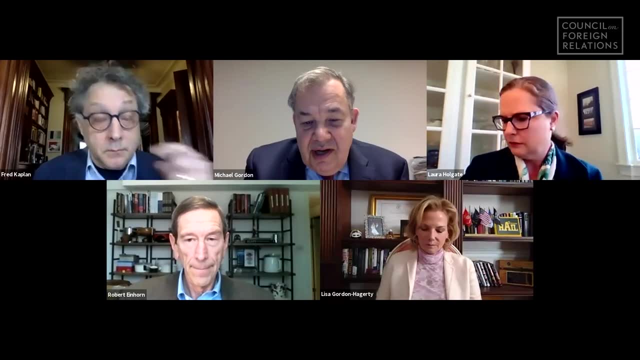 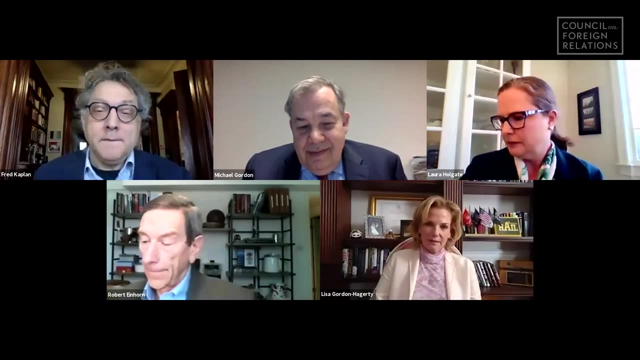 we will have an NPT. Chris, great to hear your voice. Okay, I guess. moving on to the next question, since everyone's so shy, We'll take the next question from Joe Nye. Hi, Great to be here. Great panel, great people. 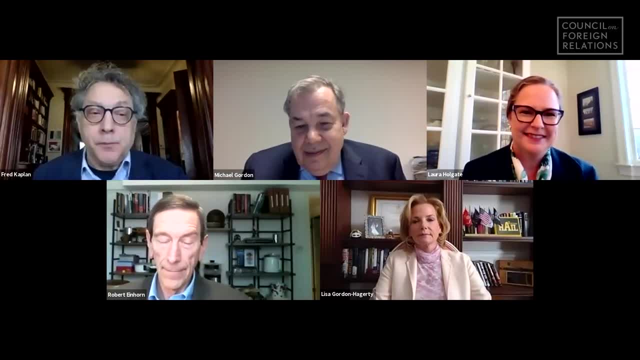 And I agree with everything said, But I'd like to hear a little bit more about North Korea and how that's going to affect South Korea and Japan. I've been involved in a number of track- two meetings with both those countries in the last few months. 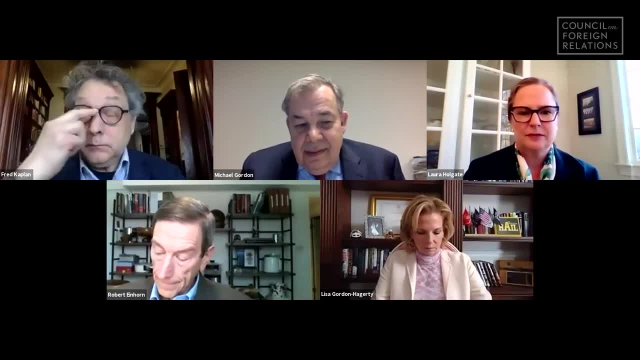 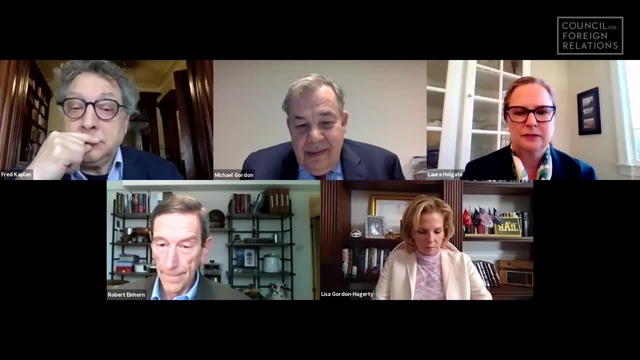 And they're very worried about legitimizing North Korea's status as a nuclear weapons state. Rich Armitage and I just issued another report on US-Japan alliance And we tried to duck that by saying: our long-term goal remains the ultimate denuclearization of the peninsula. 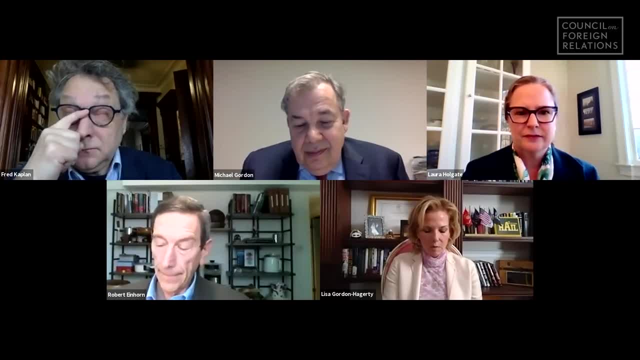 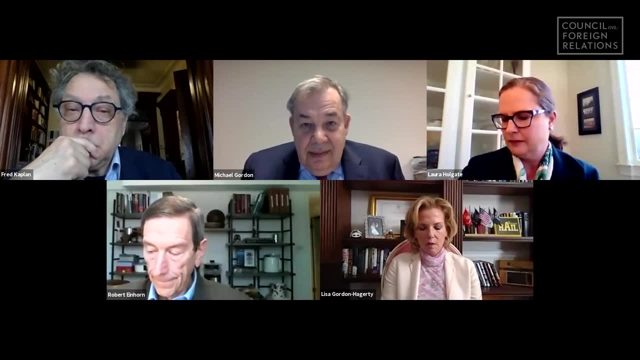 But in the meantime, Biden's going to have to do a number of things in terms of trying to bargain with, or limit or contain North Korea. How do you square that circle? How do you? what would you recommend, Bob? why don't I put this to you? 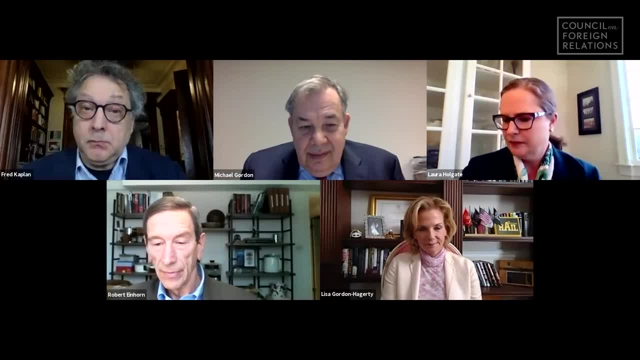 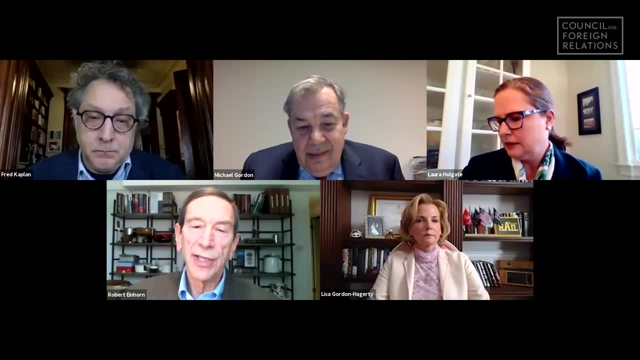 When I used to work on this together. How should Biden handle or approach the North Korean problem? Yes, Joe, It's look. the goal must continue to be the eventual complete denuclearization of North Korea. We cannot accept North Korea. as a nuclear weapons state. If we did, I think both Japan and South Korea would be terribly concerned And they may reconsider their own option to acquire nuclear weapons. So the goal has to be complete denuclearization, But it should be clear by now. 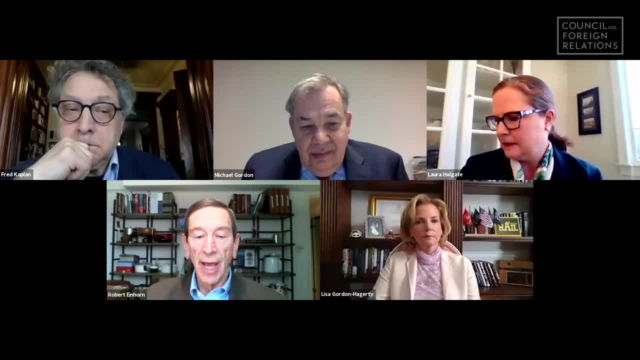 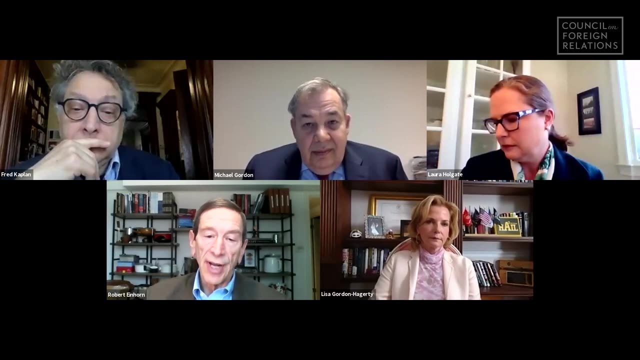 that this is not going to happen in a single step and at an early date, or even in the foreseeable future. This is a long-term goal And I think the Biden administration must adopt, you know, denuclearization as a long-term goal that has to be pursued. 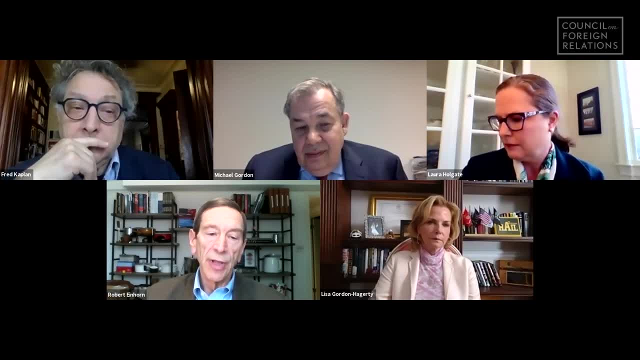 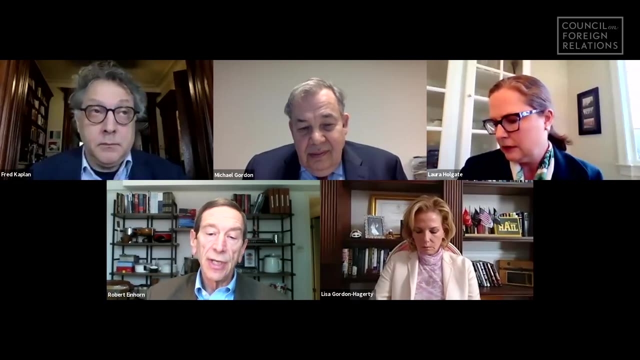 on a step-by-step basis, With reciprocal benefits to the parties at each step of the way, which includes removing or suspending some of the sanctions and economic pressure against North Korea, And so it should focus now on an interim agreement, a first step on the road. 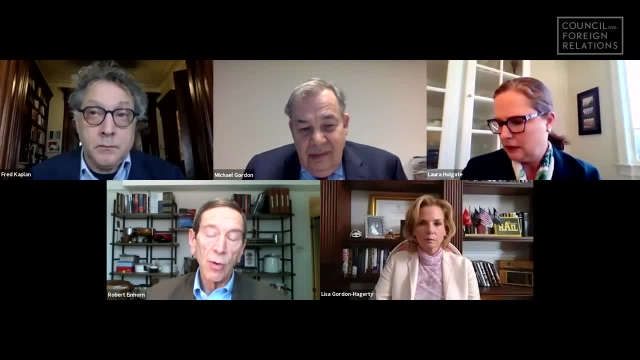 toward complete denuclearization And, in my view, such an interim step could include the formalization of the current moratoria on nuclear weapons testing by the North and the flight testing of long-range missiles. In addition, there should be a prohibition on the prohibition. 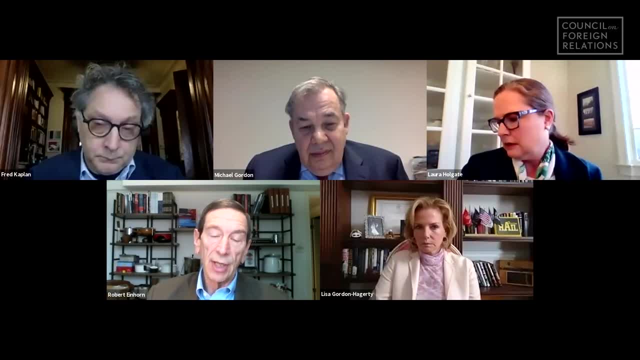 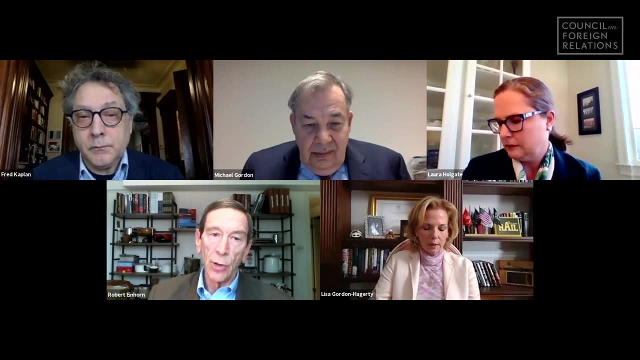 a prohibition on the production of fissile material, separated plutonium or enriched uranium anywhere in North Korea. This will be hard because verification of a nationwide ban on fissile material production will require intrusive measures and the North Koreans will resist intrusive verification. But I think it's a goal. 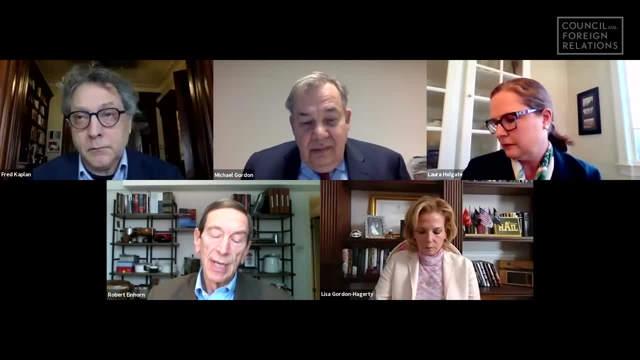 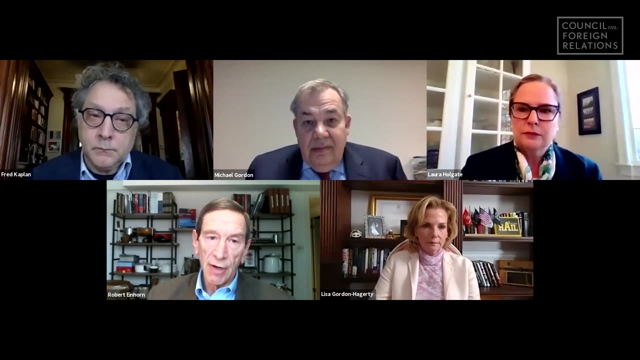 that would be very important. It would cap the material that North Korea could use in building nuclear weapons And I think would alleviate concerns by Japan and South Korea about the buildup of the North Korean nuclear threat. So it's a half measure, but it's the most practical measure. 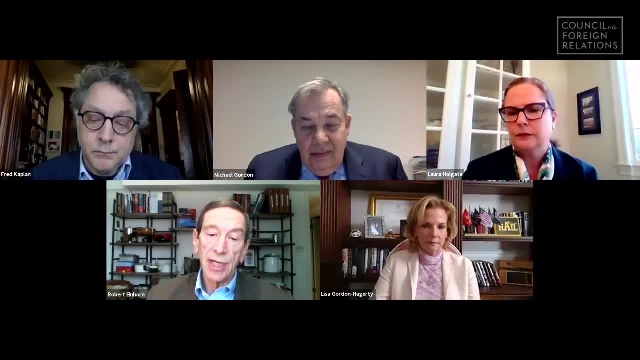 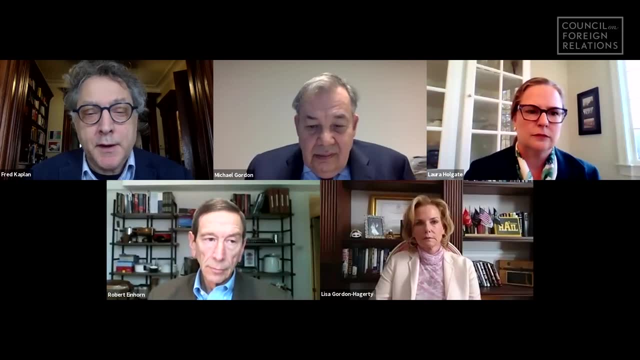 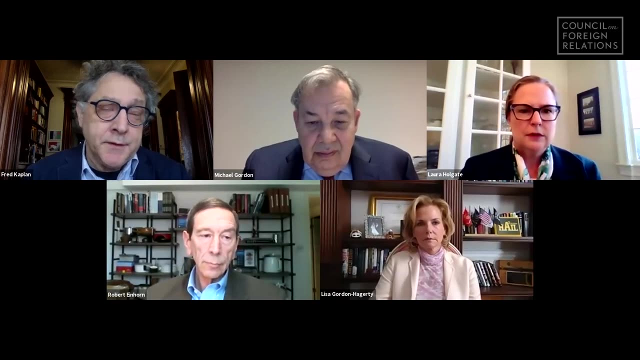 at the present time And it's best for non-proliferation in Northeast Asia. Well, I would just say there was a time- and Bob Einhorn was very much involved in this- before North Korea had nuclear weapons, that there was an opportunity. 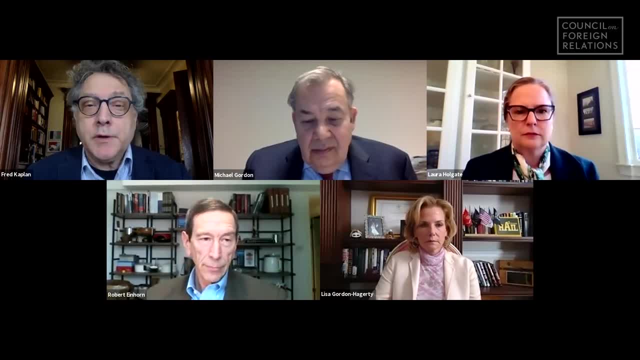 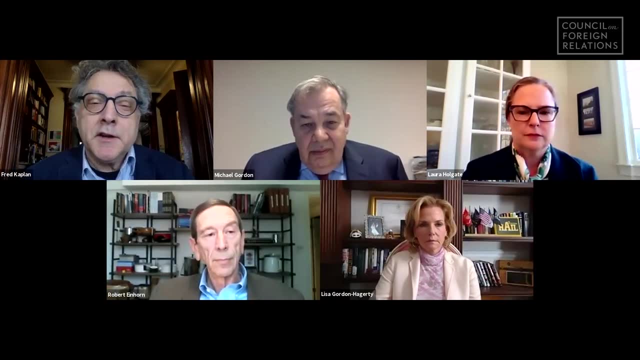 to contain them And in fact, the agreed framework, which is much derided, was actually a very successful agreement as far as it went. It didn't go all the way, but what it banned, it really did affect things And we were supposed to reciprocate. 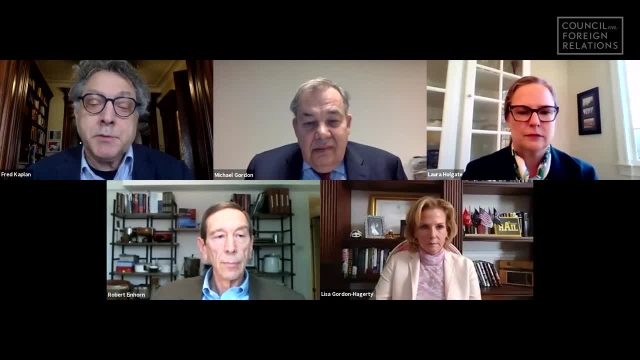 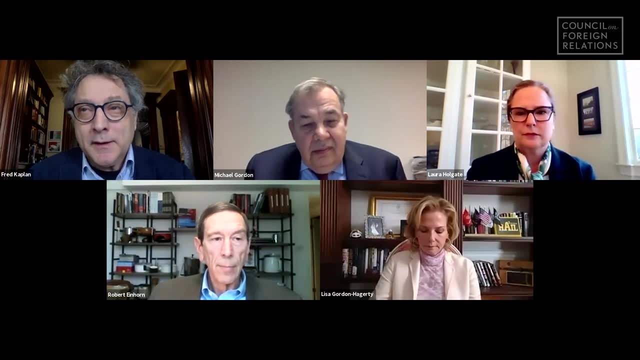 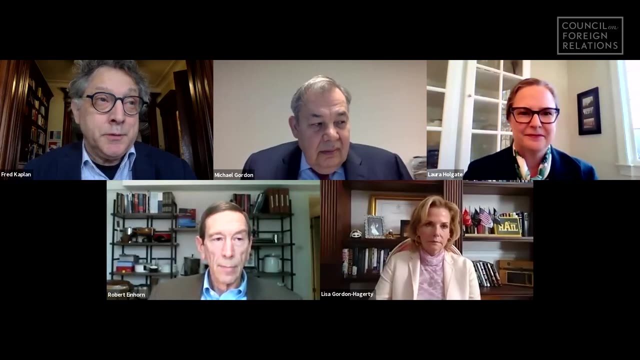 with the providing of light water reactors, which we never did, And there was supposed to be diplomatic relations, which there never was. Now, however, I think, now that North Korea has a pocket full of nukes and a leader who is perhaps 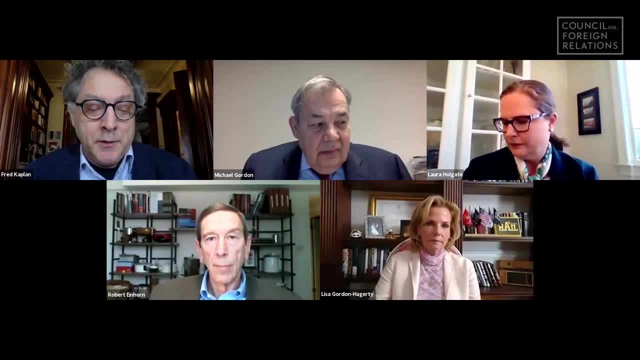 a little more wild-eyed or unpredictable than his father, his father and grandfather. it's going to be hard to do any of these steps. I mean step number one to anything should be North Korea making a statement of what they have. I mean, you can't have any statement like 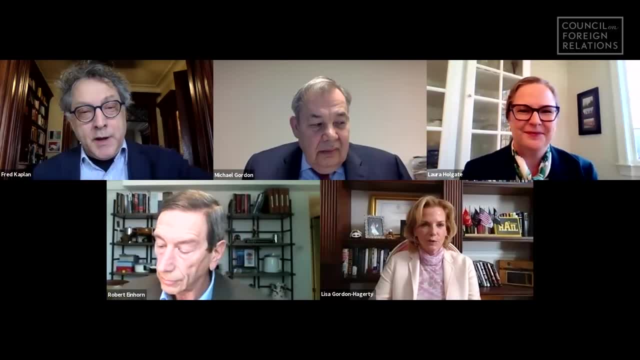 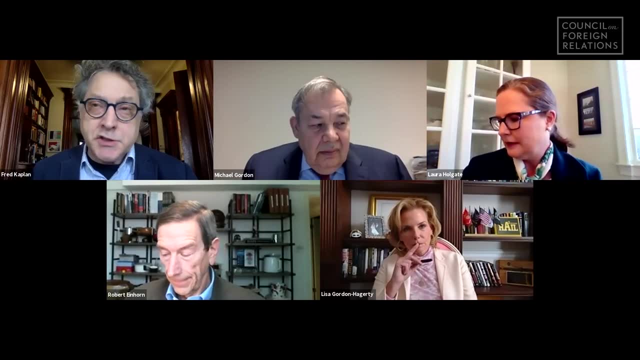 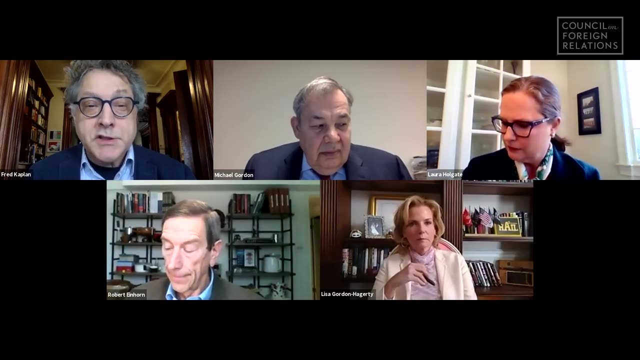 okay, I'm reducing 20% of my nuclear weapons, while you get rid of 20% of your sanctions without knowing what the baseline is. And North Korea, in the negotiations with the Trump administration, just resolutely refused to provide any data whatsoever. 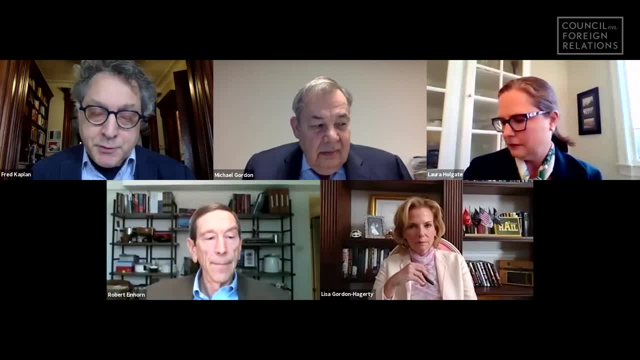 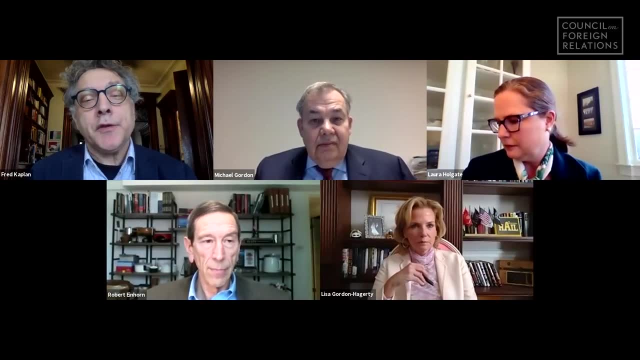 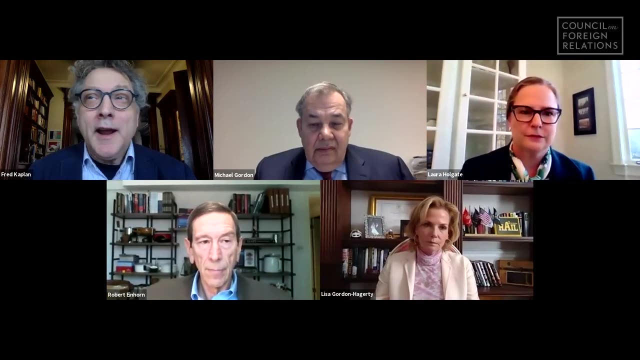 I don't know how you get around that. as long as politics remain the same, they are, I think while it is unwise to officially acknowledge that North Korea is a nuclear weapons state, I think we do have to accept as a practical matter that they kind of are. 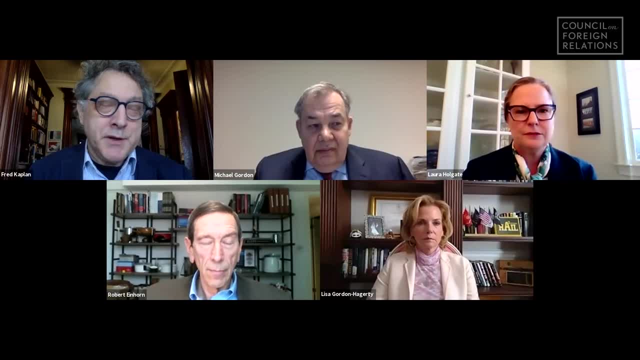 and that containment and continued pressure can go a long way to prevent them from doing anything haywire. I mean Kim Jong-un, you know. I remember HR McMaster once saying something like that: he's not because he kills his own people. 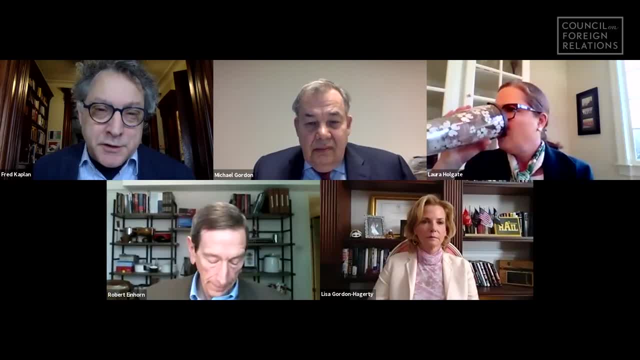 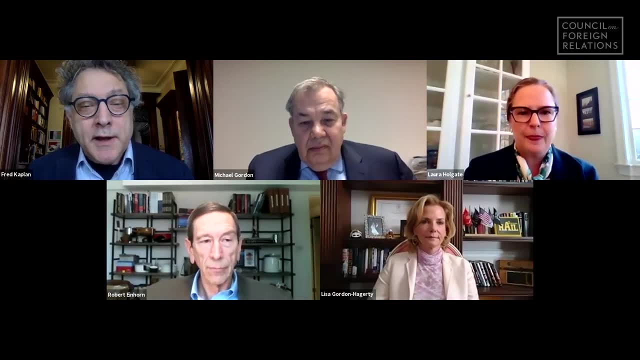 he's not susceptible to classical deterrence theory. Well, it seems to me that since he killed these people in order to perpetuate his own rule, he's actually quite susceptible to classical deterrence theory. He doesn't want to endanger himself or his regime. 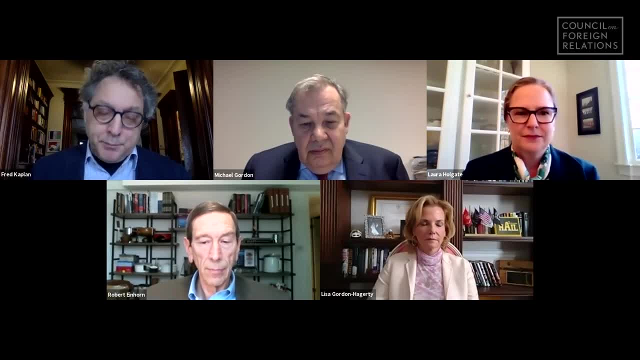 And I think yes, push for all these possible openings for negotiation, but in the meantime it has to be a continued containment and pressure and stiffening the alliances and any openings of cooperation with the countries around North Korea. Let's take the next question. 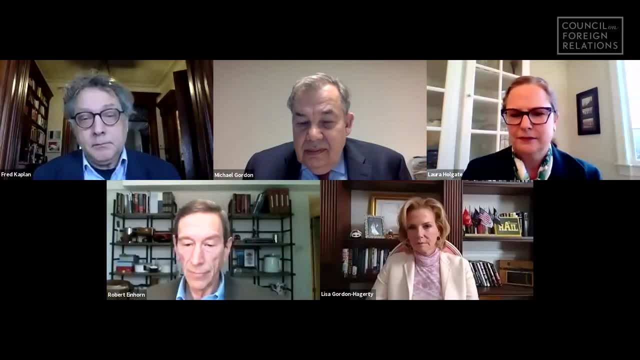 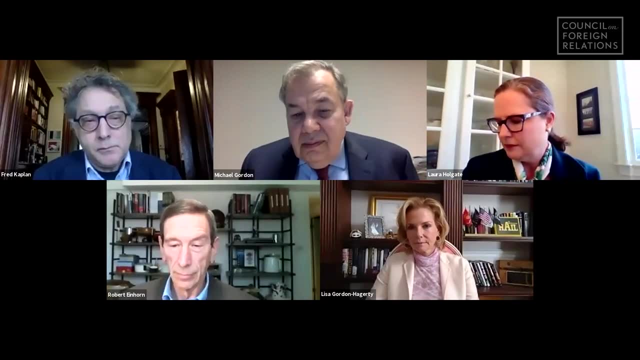 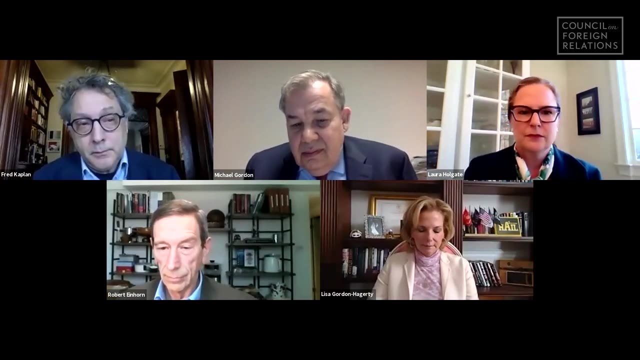 We'll take the next question from Cynthia Roberts. Thank you all for doing this tremendous call. My question actually follows from the one on Korea. It's related to the problem of, and the challenge of, US extended deterrence. We know that the Biden administration 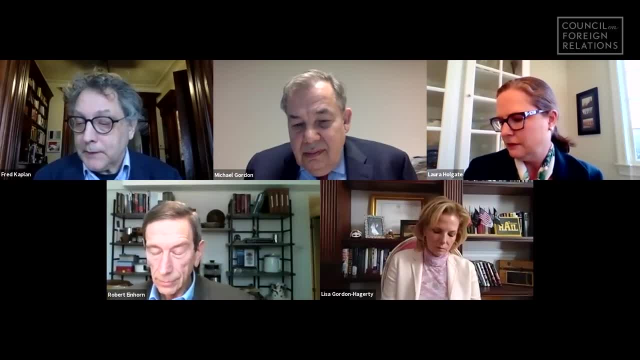 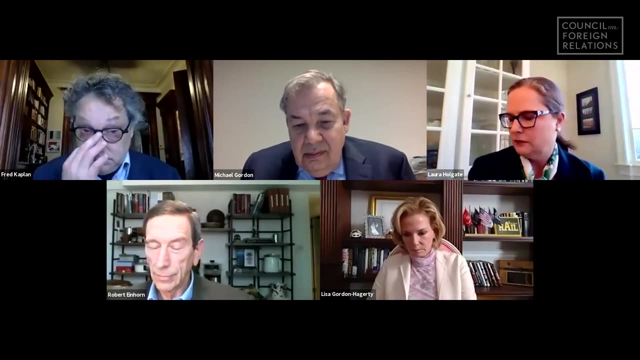 wants to deepen and correct and improve our relations with our allies, but it's unclear how much they're going to support the recapitalization of the nuclear deterrent, which was just passed in a bill through Congress. But more is needed there. And then there is the additional question. 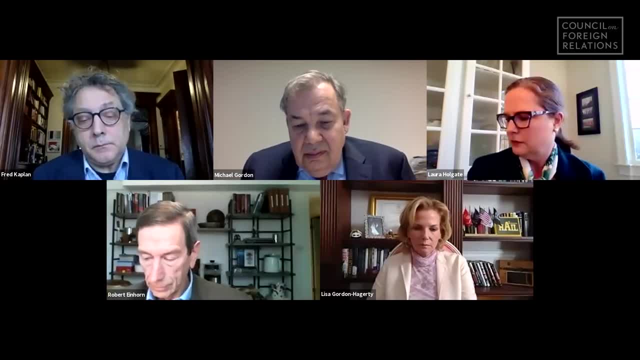 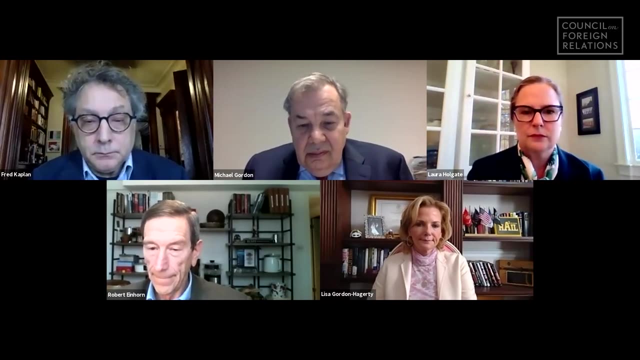 of how flexible the NPT can be interpreted, going forward on this question of extended deterrence, For example, we still get challenges from the Russians on nuclear sharing in NATO. What if it's needed in Asia to do something of the same sort Or similarly? 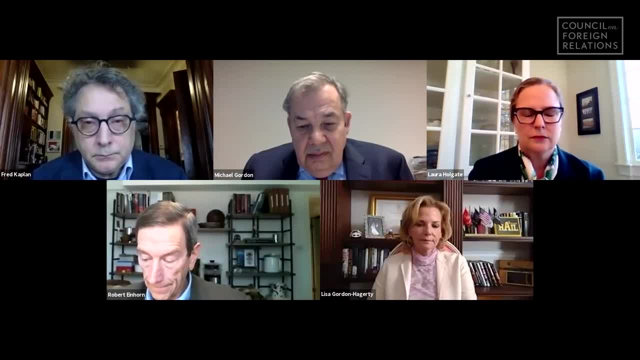 what if the Europeans actually surprisingly, deepen their strategic relationships and their defense relations and decide to pursue a European nuclear option? Is the NPT flexible enough to allow for this, And are the Americans prepared? Is the Biden administration prepared to go forward with enhanced nuclear sharing? 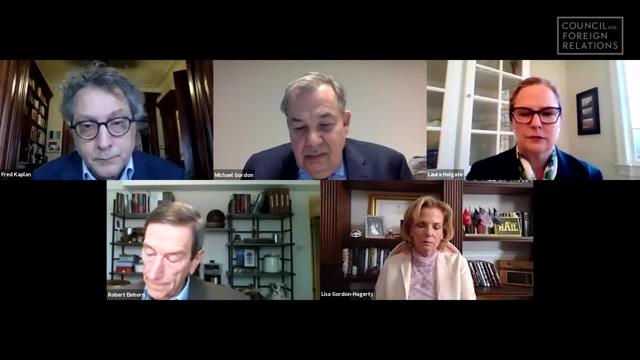 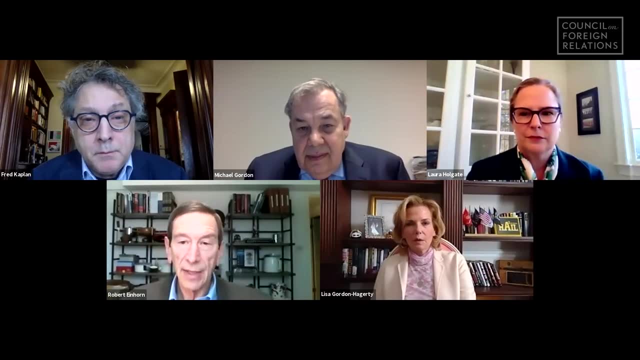 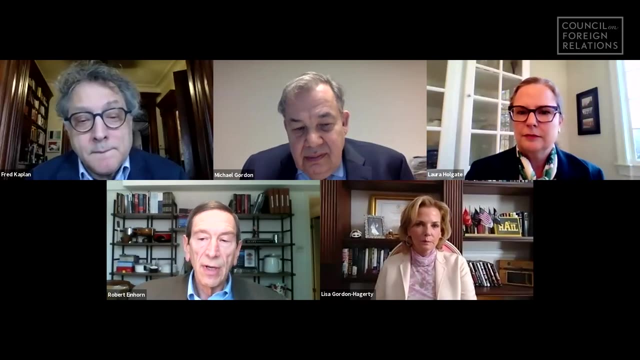 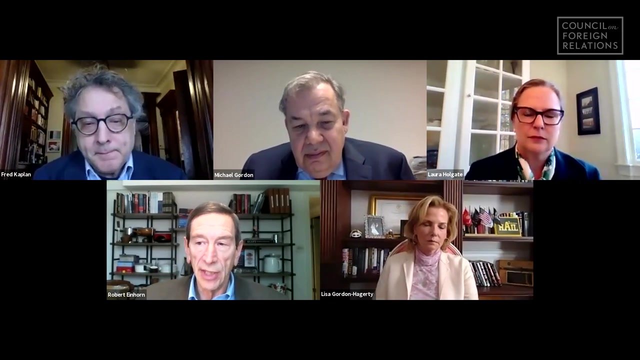 to reassure our Asian allies, not just our European allies. Thank you very much, Bob. why don't you go first and then Fred? Yeah, You know, I think effective diplomacy with North Korea would not be possible without a strong alliance system. 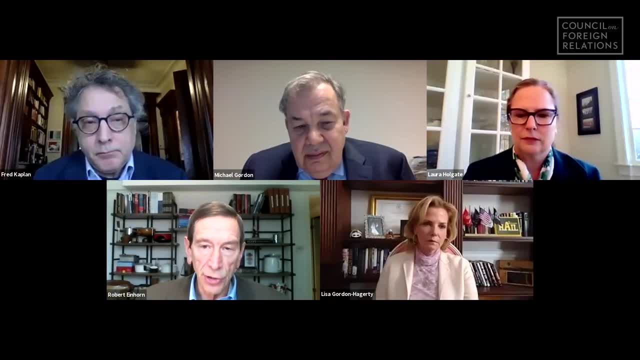 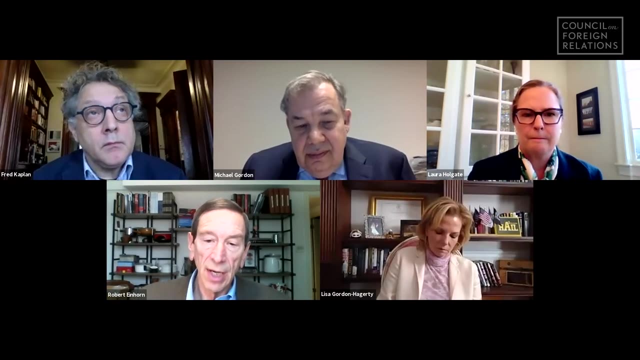 I think the first step of the Biden administration will be to shore up the credibility of US assurances and to strengthen alliance deterrence and defense capabilities. That's the foundation to pursue diplomacy with North Korea. In terms of extended deterrence, I think Cynthia is right. 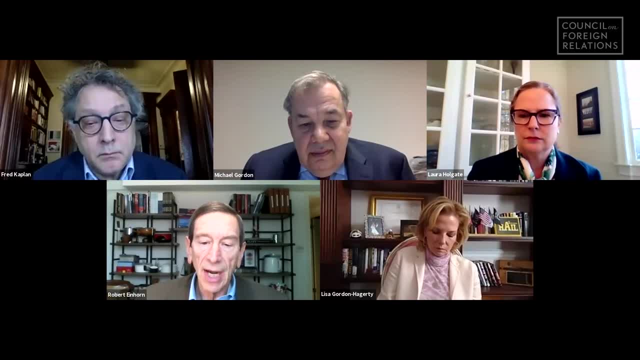 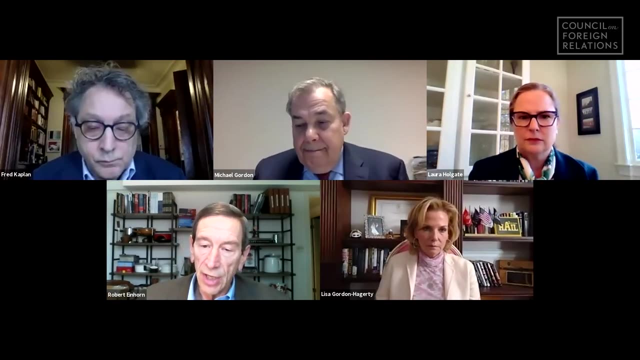 I think we have to take steps to reinforce the extended deterrent. I think that can be done short of, for example, having US nuclear weapons stationed in South Korea, as US weapons continue to be stationed in certain NATO countries. I think the NPT is flexible enough. 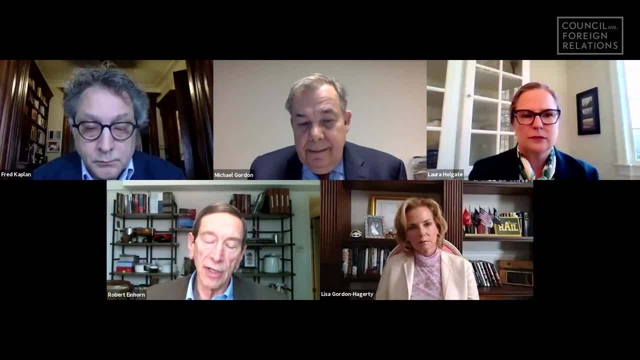 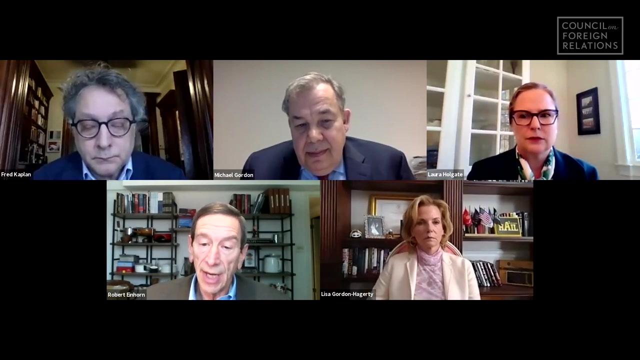 to permit the stationing of US nuclear weapons abroad, provided they're kept under US control. I don't think that will be necessary in Northeast Asia In terms of adopting some of the the burden-sharing in South Korea as it's pursued in Europe. 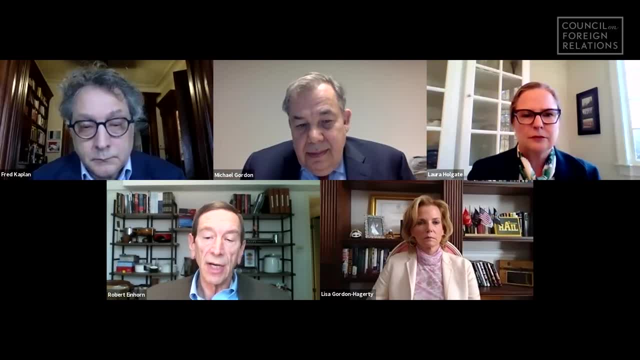 I think the US can do more to give South Korean allies more of a say about how the US extended deterrent is planned and operationalized in Northeast Asia. But I don't think the type of deterrence or the type of nuclear-sharing arrangements. 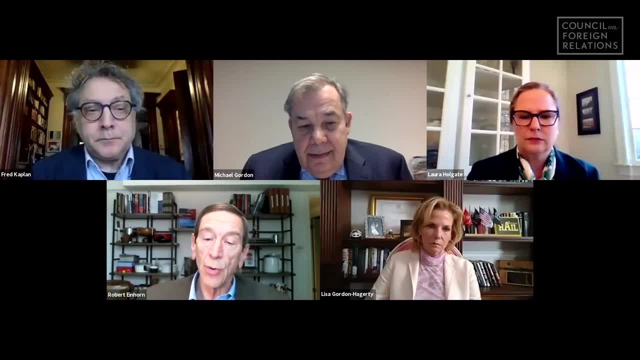 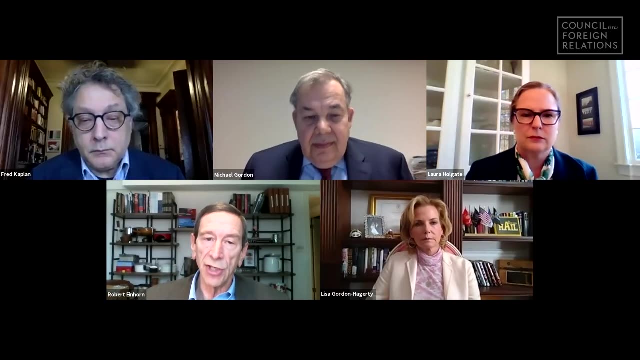 adopted in NATO, for example, training allied pilots to deliver US nuclear weapons. I don't think that's necessary in Northeast Asia And I think there'll be political inhibitions in Northeast Asia to establishing those kind of nuclear-sharing arrangements. Yeah, I would just say. 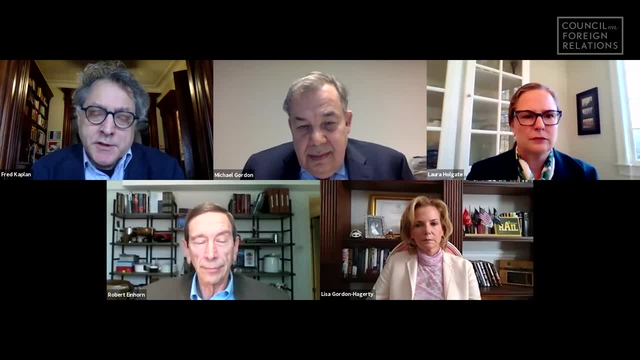 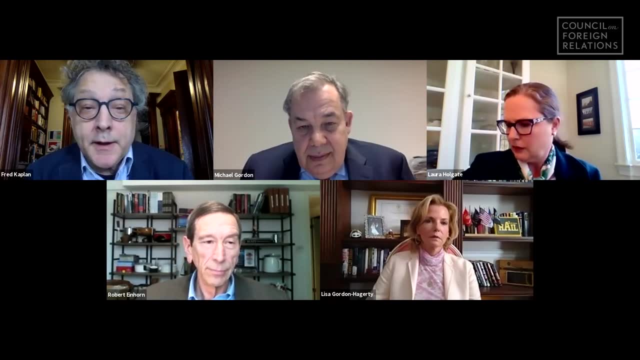 a few things very quickly. One: I don't think that extended deterrence requires the modernization of all three legs of the nuclear triad, And I think we will see, under the Biden administration, a serious reassessment of whether we need to go ahead with 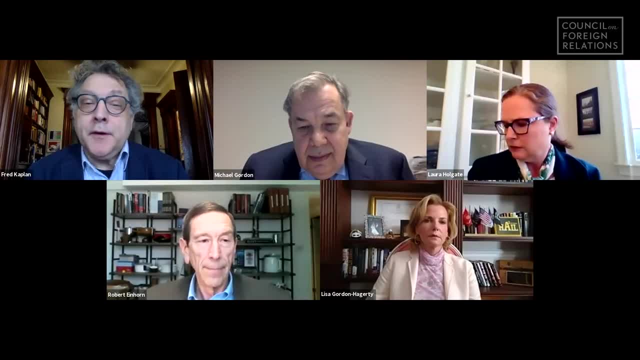 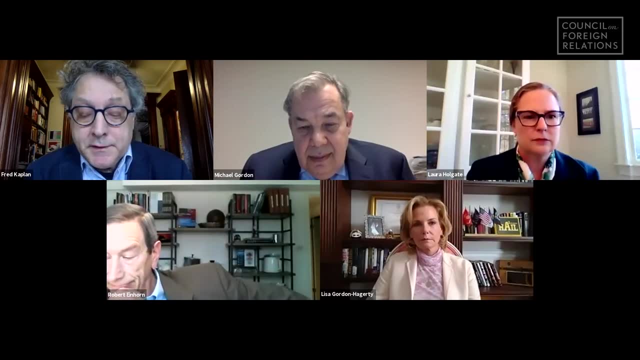 400 new ICBMs, new air-launched cruise missiles in particular, and maybe even a new strategic bomber. The surface-life agreement for extension programs could have taken us a long way and could take us further In terms of a European Union nuclear force. 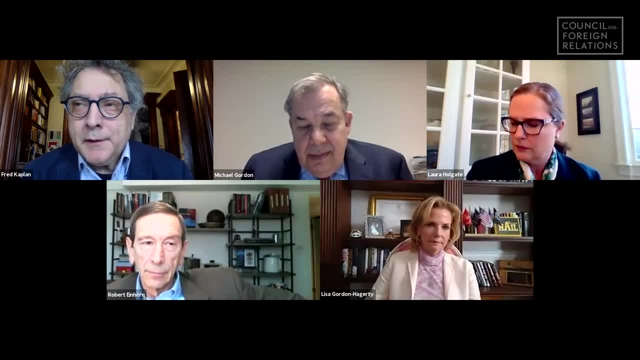 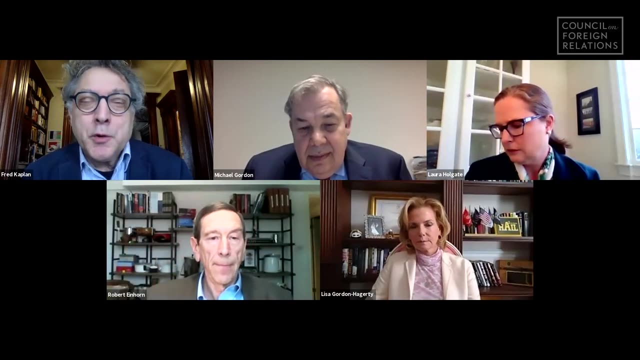 I find this pretty implausible. You know, right now, of course, Britain and France have their own nuclear forces, which were explicitly omitted from the count of the INF Treaty, which means who gets, who would be really, in effect, the nuclear power. 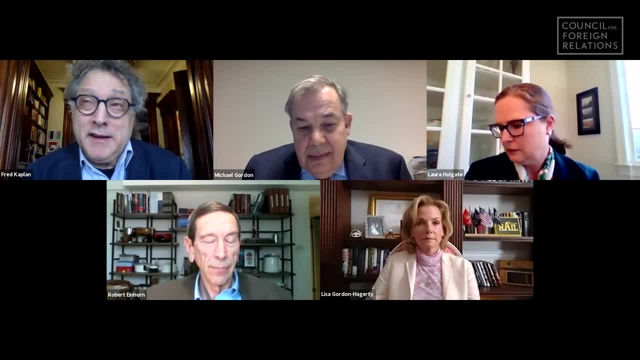 in an EU nuclear arsenal, It would be Germany, And I think you know, even though Germany has proved itself no longer to be so infected by the 1940s as it used to be, I think there'd be a lot of resistance. 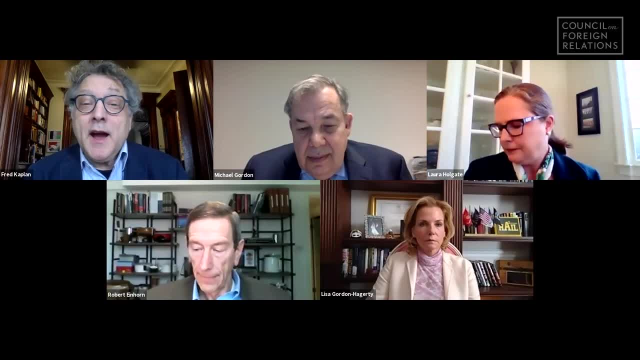 to that, including inside Germany. One interesting thing about Biden and extended deterrence: he is on record as supporting a no first use declaration. If you had no first use, that's kind of the end of extended deterrence. However, he has also said: 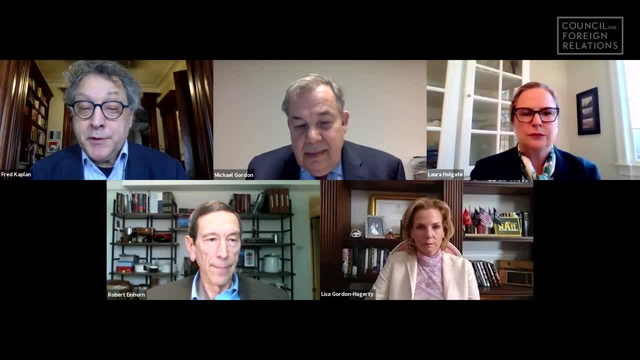 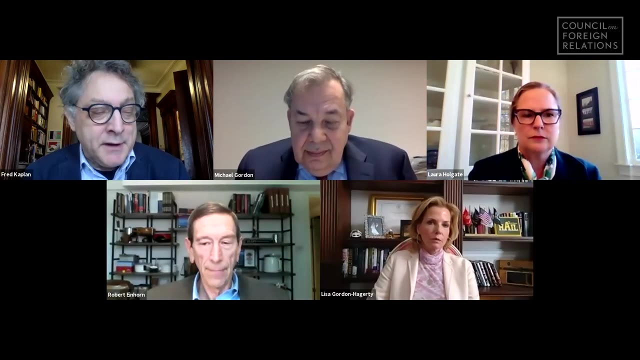 we would adopt that as policy only in consultation with our allies, which is kind of a you know kind of a concession that it's really not going to happen. In the Obama administration, where Biden was, of course, vice president Biden, I mean Obama- said: 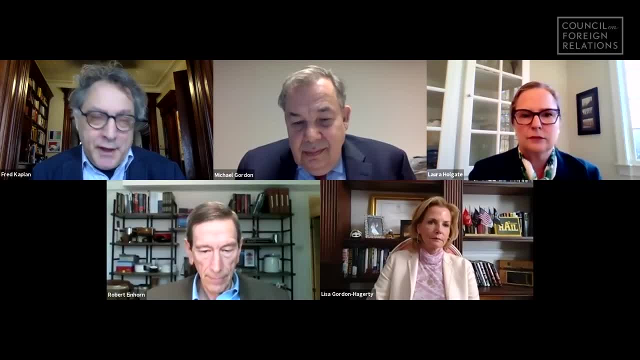 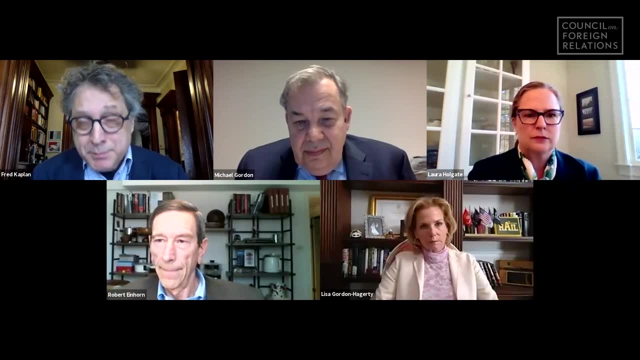 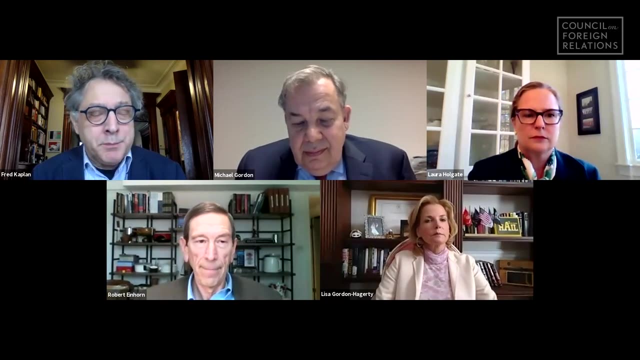 in private meetings several times that he really didn't think that any American president would use nuclear weapons first. However, he accepted the arguments that if we declared that as policy, the allies would go nuts, And he also accepted an argument put forth by Secretary of Defense Bob Gates. 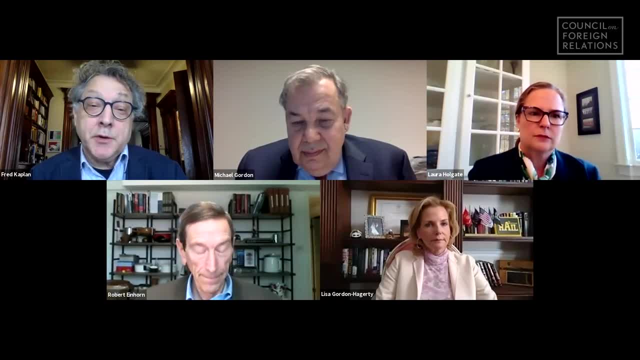 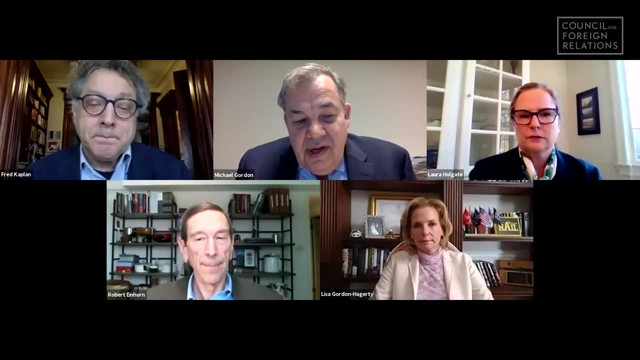 that. well, some countries have biological weapons that can do tremendous damage, And we gave up biological weapons, And so nukes can be a deterrent to that, And why tell anybody that we're abandoning that as a possible deterrent? Actually, Fred, during the campaign. 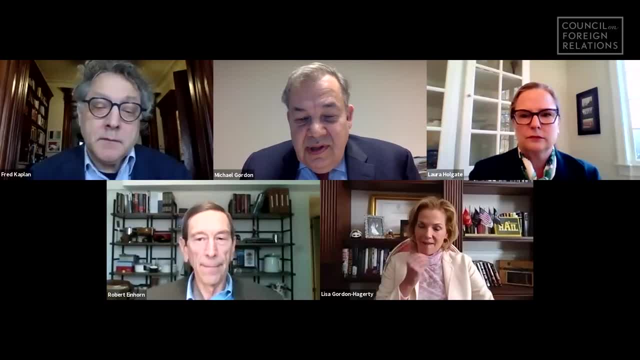 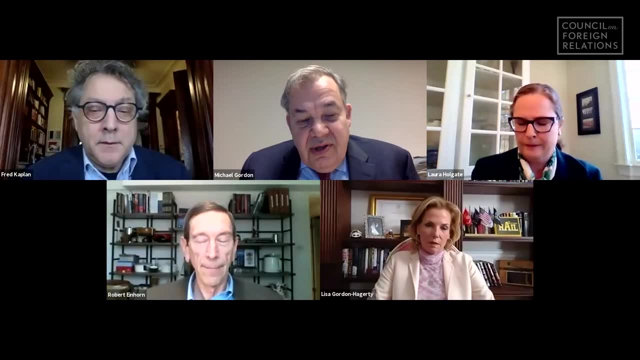 Biden didn't endorse no first use. What he endorsed was sole purpose, which was the proposition that nuclear weapons can only be used to deter other nuclear attacks or preempt a nuclear attack, but would not be used in response to a conventional attack or cyber or things like that. 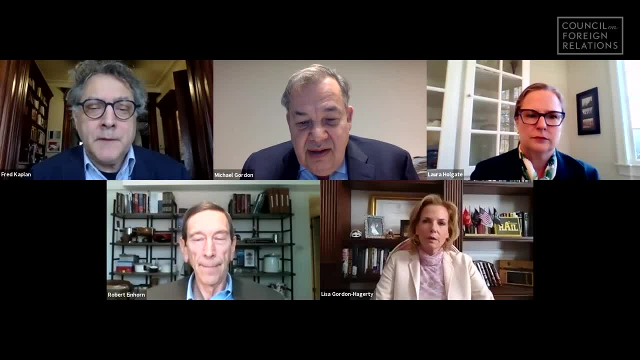 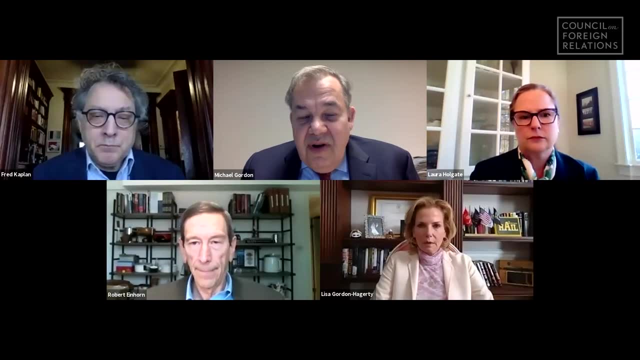 It's a little different than no first use, but he had, as you pointed out, the important caveat That this would only be done in consultation with allies and with the military. Let's go, We're down to sort of our last five minutes. 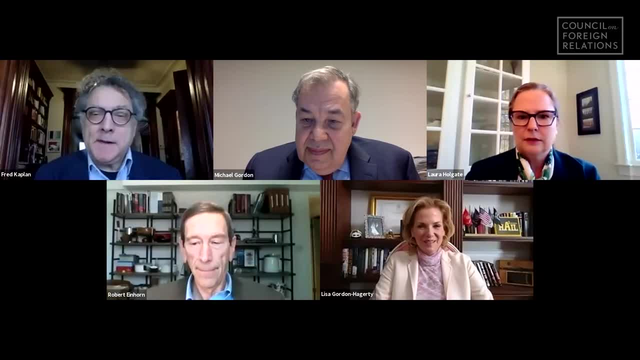 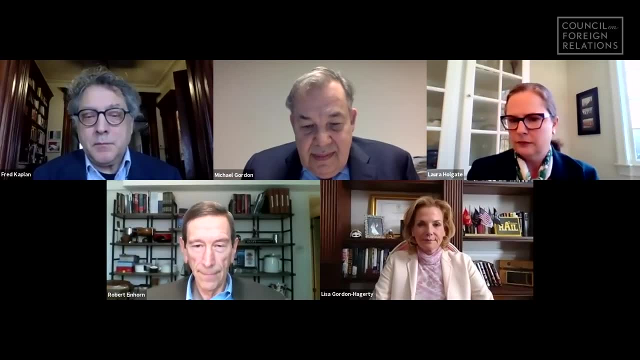 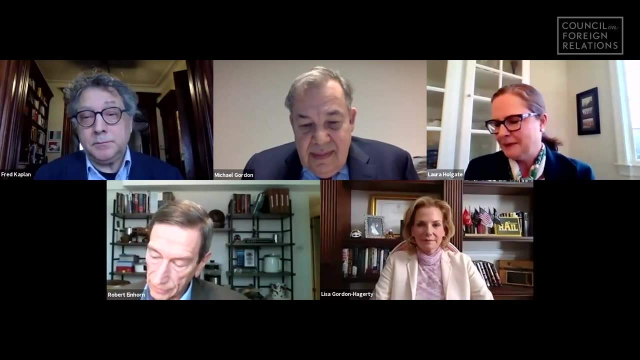 Let's just try to squeeze in a few more questions. We'll take the next question from James Gilmore. Good, Thank you very much. I'm Jim Gilmore, the ambassador to the OSCE. I'm in Vienna right now. I've been sitting here. 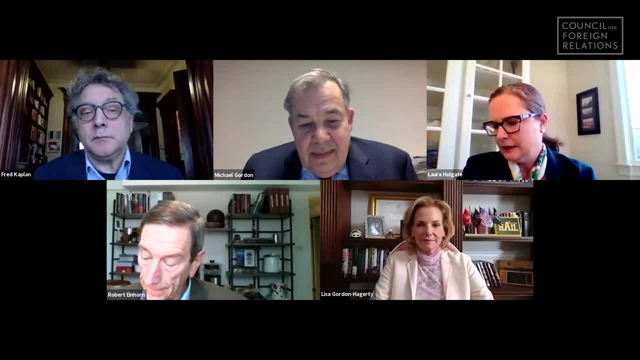 trying to formulate this in a very, very short time. I'm not sure if I'm doing it in a responsible way, but I guess my question to the panel is: disarmament is not really a goal, is it Because, in a world that's still using force, 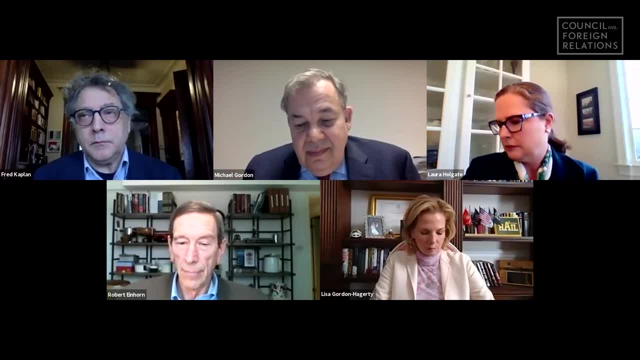 nuclear weapons are the assurance of the survival of a regime, And I think that's driving a lot of the nuclear policies. So really, what we're talking about is the reduction of certain types of weapons, aren't we? Or the types of weapons that might be used? 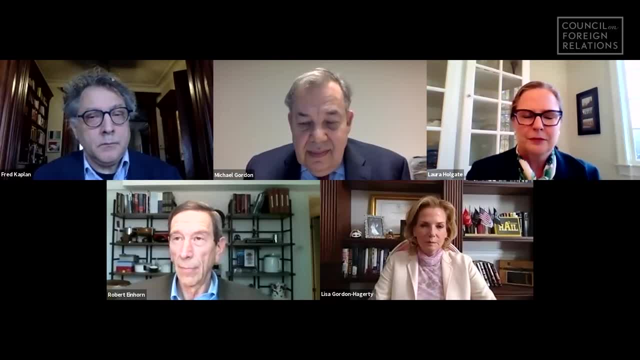 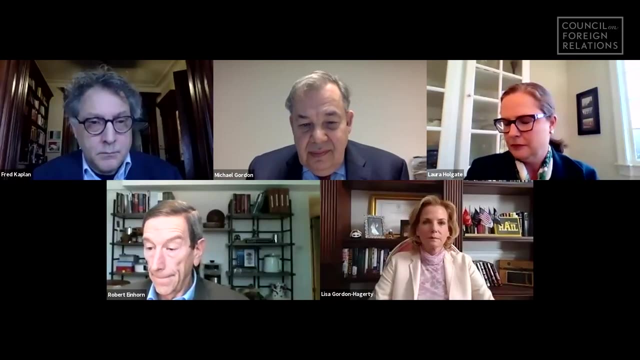 like the battlefield weapons? And secondly, if we see countries beginning to acquire nuclear weapons, what's the right policy for preventing that? We waited too long with North Korea And now we're stuck with them because they've got nuclear weapons and now they have assurance. 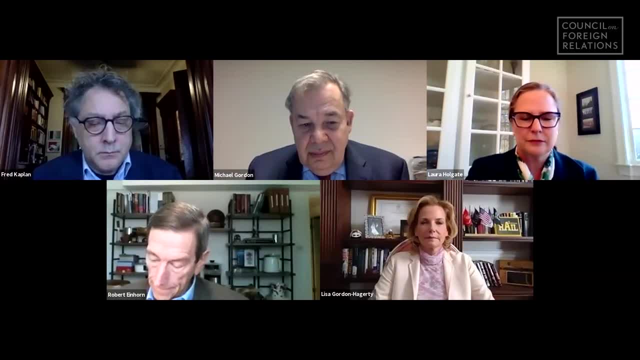 of regime certainty. What do you do when a country is basically moving towards that? now that we've learned, What do you do? Do you move in militarily and just take it out Which we're capable of doing before the crucial event? So thank you very much. 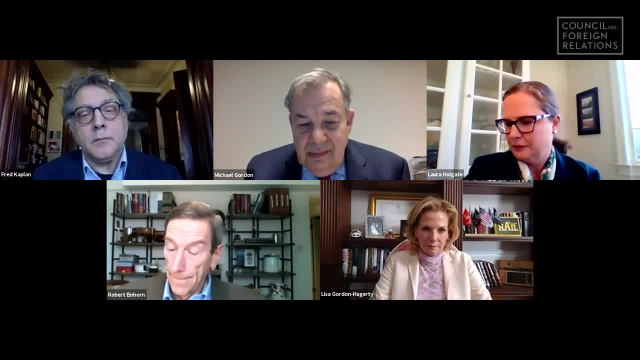 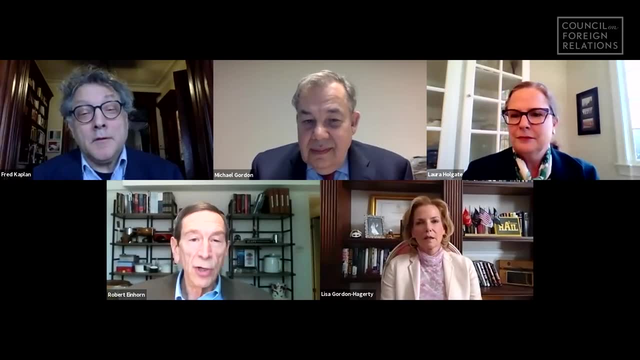 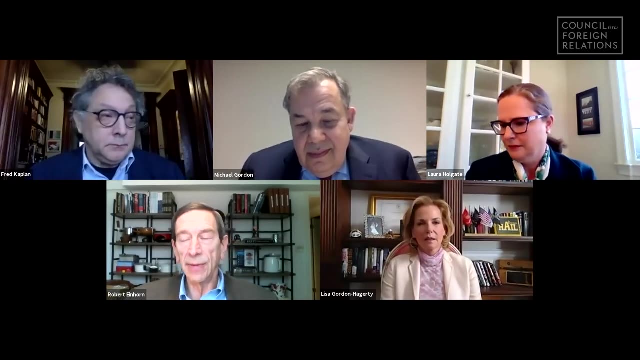 I'm really grateful for this opportunity to listen to you, this distinguished panel. What do you do when you see a country moving to nuclear weapons? We saw Iran moving in that direction, And so the United States under President Trump, President Bush. President Obama put intense pressure on Iran, Not enough pressure to get them to give up their enrichment program altogether, but a willingness to on Iran's part to accept strict limits on their program, effectively in the JCPOA, effectively blocking their paths. 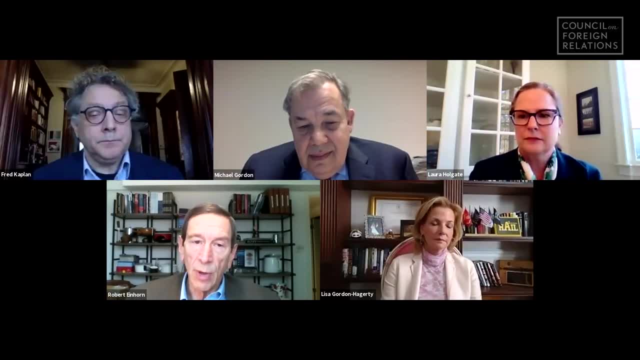 to nuclear weapons? I think we were. you were right, we're a bit late on North Korea. They'd already separated enough plutonium for one and a half nuclear weapons by the time the agreed framework was put in place. But I think it's a question. 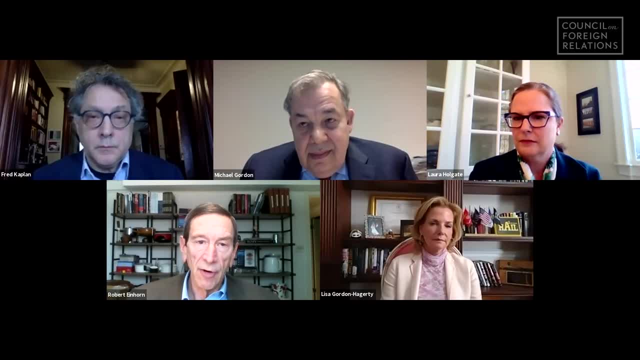 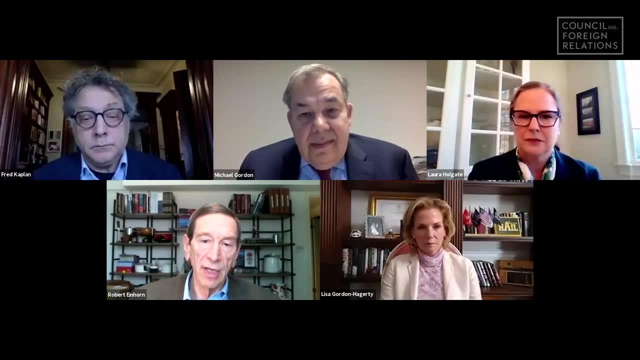 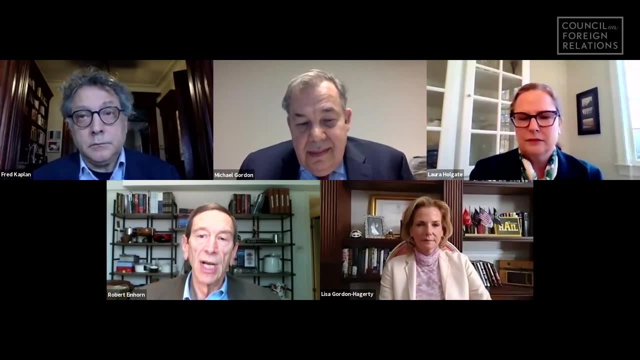 of building broad international support for preventing these developments, putting intense pressure on these countries to stop their pursuit of nuclear weapons Use of military force. the United States has, you know, considered the use of force against North Korea's program. You know Israel was asked. 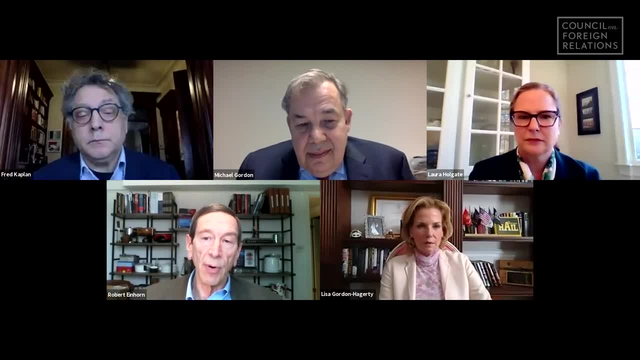 in the United States to join them in using military force to stop Iran's program. I think in both cases those administrations wisely decided that military force would not be effective in a durable, for a durable period that is more likely to you know. 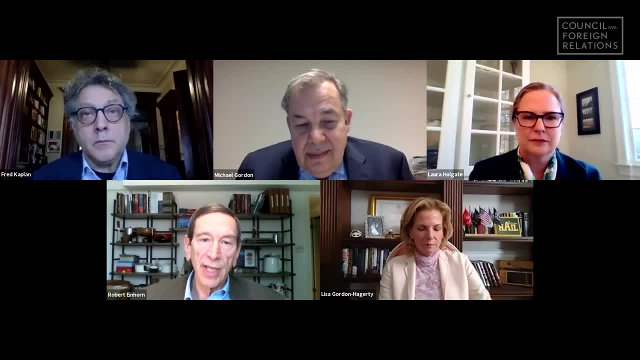 to rile up these countries and to make them even more determined to acquire nuclear weapons in a more covert way in the future. Next question: just, Fred, I just want to give a. we only have a few minutes, so let's try to. 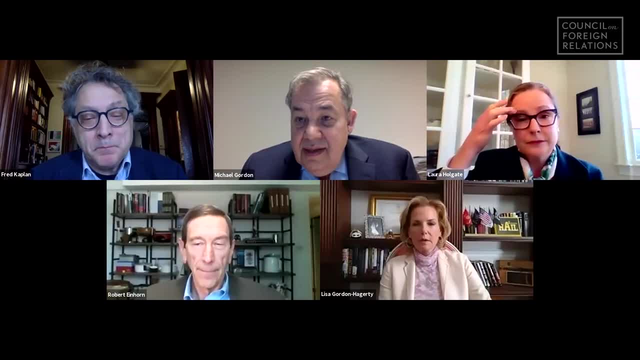 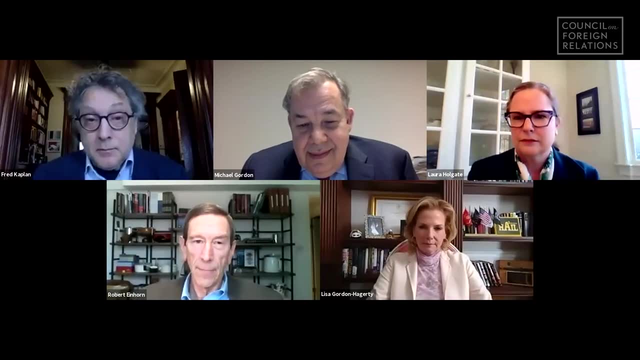 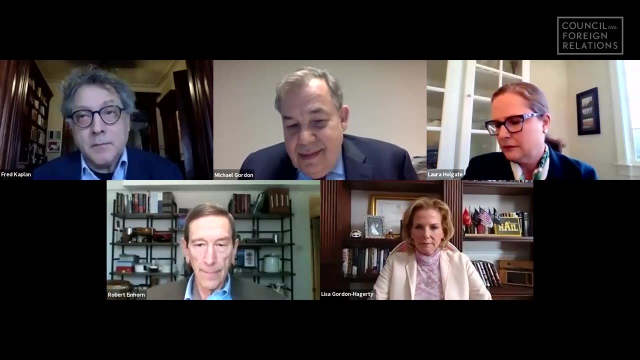 you know, see what other people have to say. Okay, We'll take our next question from Henry Sokolsky. Thank you very much. I'm with the Nonproliferation Policy Education Center, And first I'd just like to note: 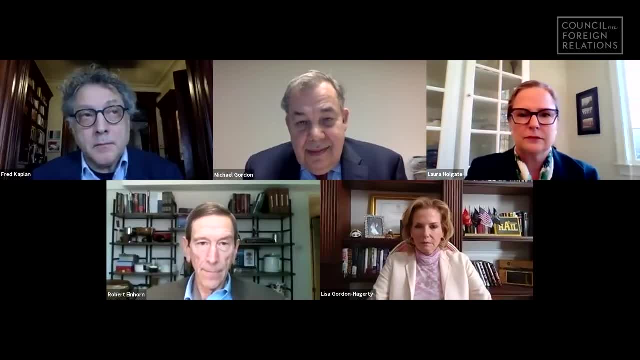 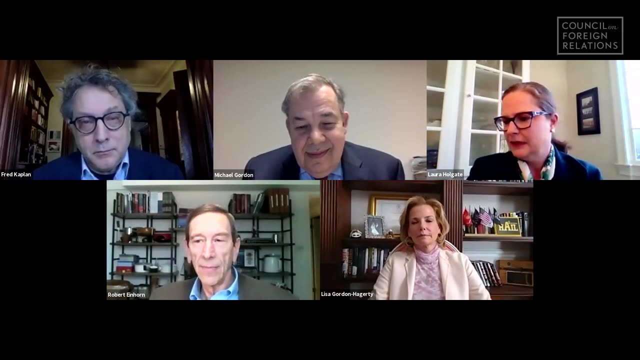 that the NPT Irish resolution. actually, if you talk to the Irish they think that's what happened in 1958, not 1961 or 64. So we've run that ground. Question I have is: given the emphasis that Egypt and other NPT members. 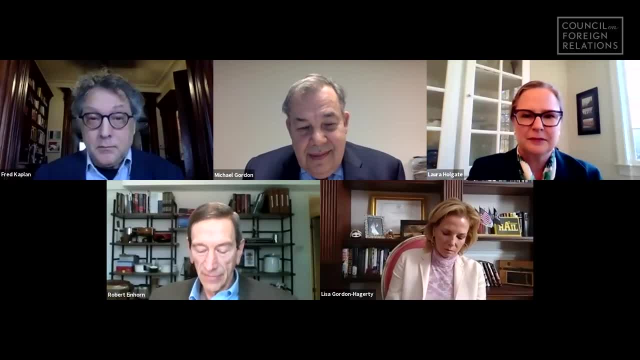 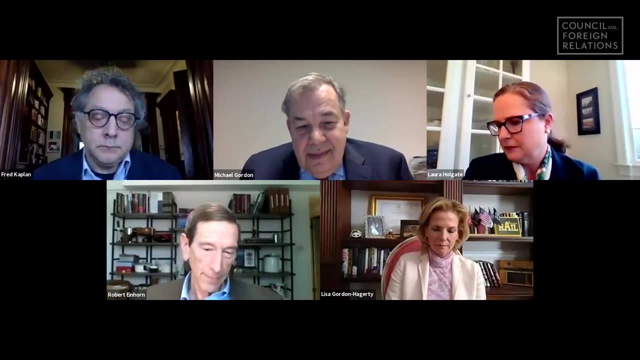 have placed on conducting serious Middle Eastern nuclear weapons-free zone talks? why is it in America's interest to continue to deny Israel has nuclear weapons? Would you advise the Biden administration to agree, as Trump did not, to admit that Israel has nuclear weapons or in any way diplomatically? 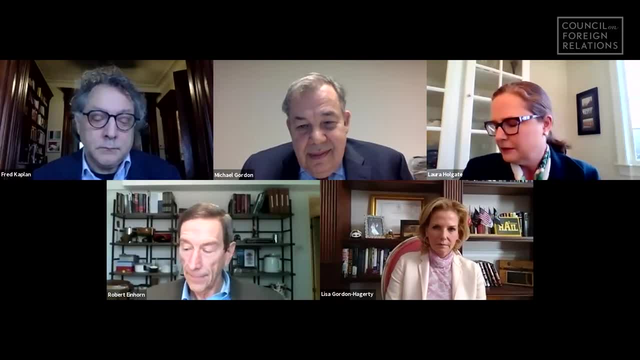 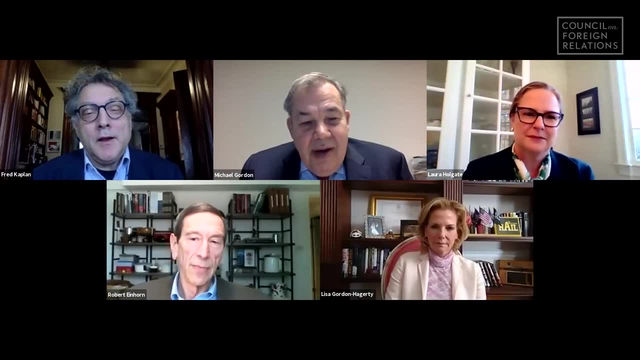 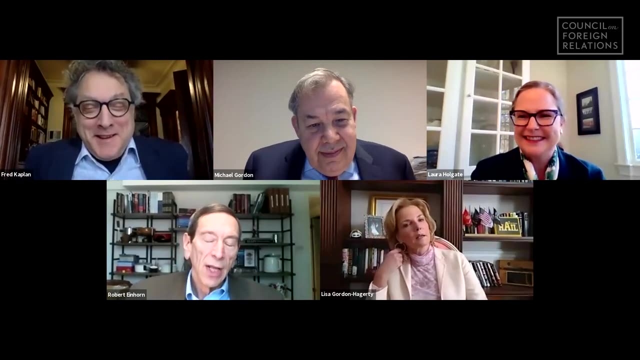 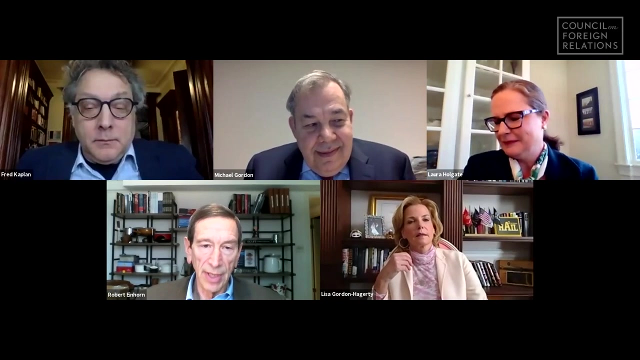 to raise the matter of Israel's nuclear weapons program in public. Okay, Bob, you start and then we'll take that on. You're sort of the proxy for the deep state. Look, the United States has appreciated for decades Iran's capabilities. But it's cooperated in Israel's policy of not admitting that it has nuclear weapons. I think there's some value in not explicitly recognizing Israel's nuclear capability. For one thing, if we did acknowledge it, some of Israel's rivals maybe not now. 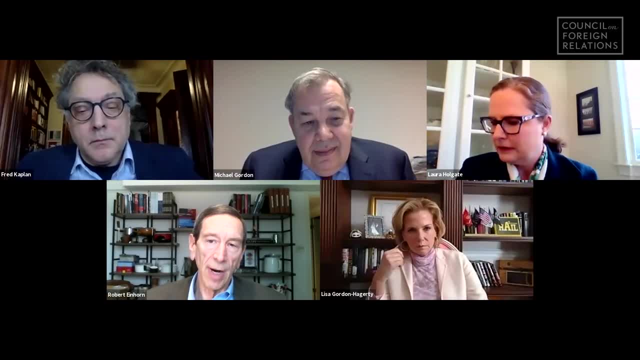 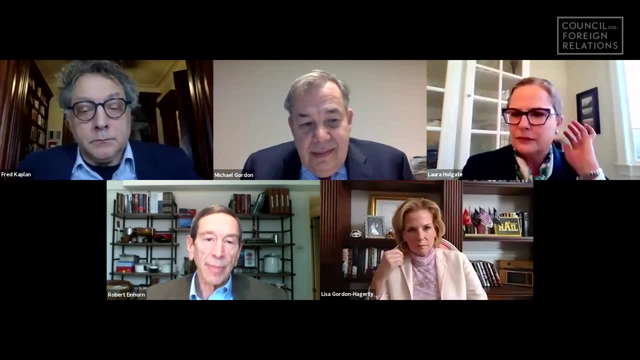 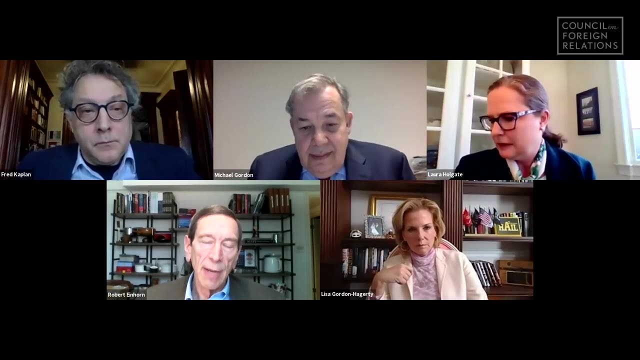 with the normalization going forward with some Arab countries. but for a long time the ability for Arabs to say we don't know for sure that Israel has nuclear weapons has been advantageous, because this way pressure would not be put on these Arab governments by their populations. 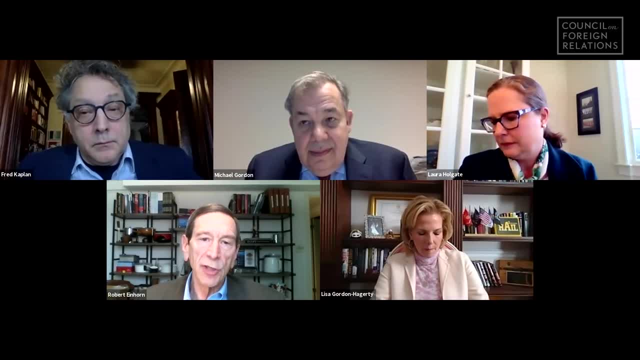 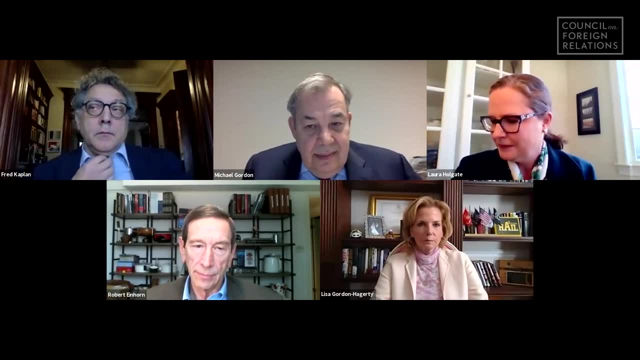 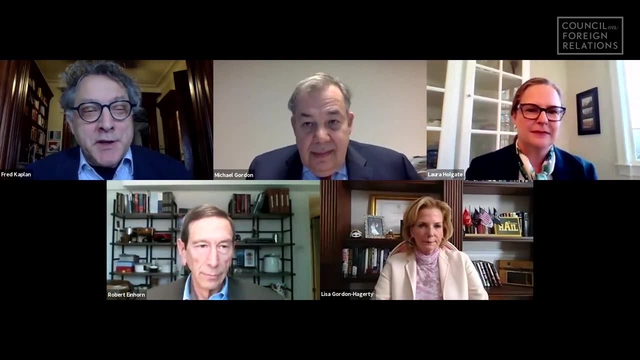 to follow suit. So it's been a useful fiction And I don't see any real reason to change that now. I think the whole enterprise of nuclear weapons and nuclear strategy is built in part on many useful fictions, For example. it's a legitimate question. 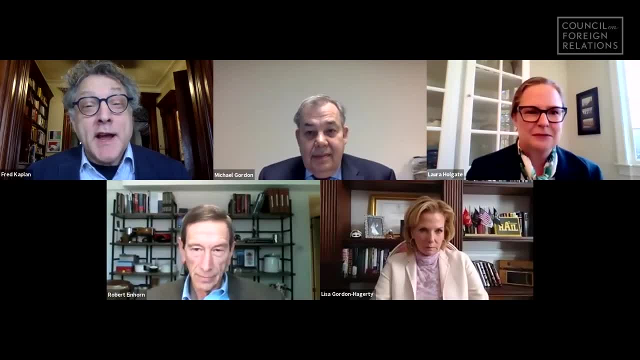 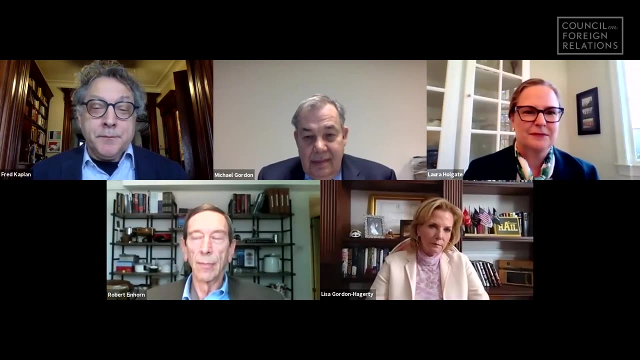 If somebody attacked us with nuclear weapons, should we attack back? But this is something that you don't even want to talk about, especially in any official capacity, because that might reduce the potency of the deterrence, the threat, Extended deterrence. 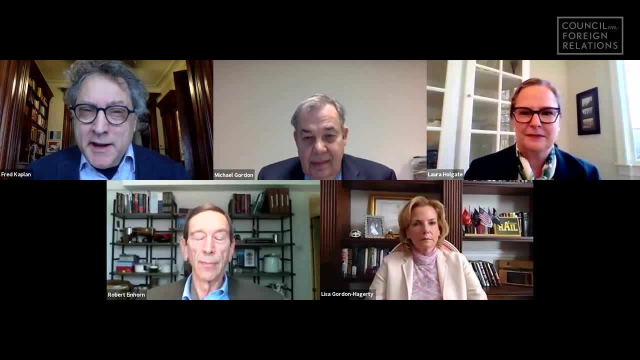 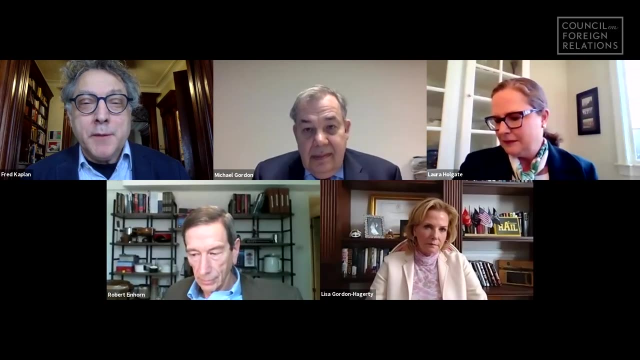 Are we really going to use nuclear weapons if, say, Taiwan is invaded by China Again? it's something that you don't even want to discuss seriously, at least in public, because it would, you know, reduce the deterrent value of these nuclear weapons. 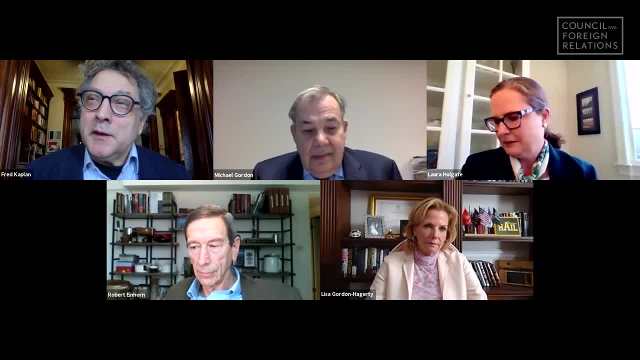 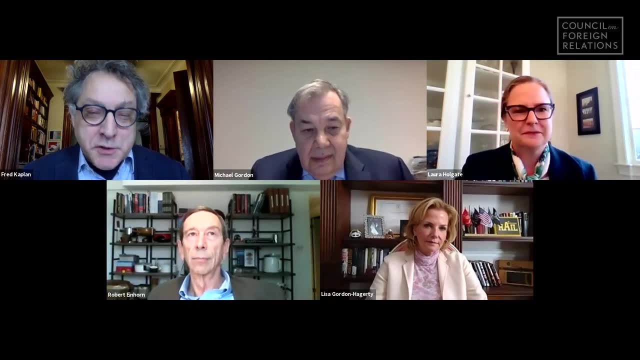 So in some ways we are all. anytime anything about nuclear policy is brought up, we are all sort of running in the street blindfolded with scissors. in a way, We're hoping on a prayer and a dime that this won't get out of hand. 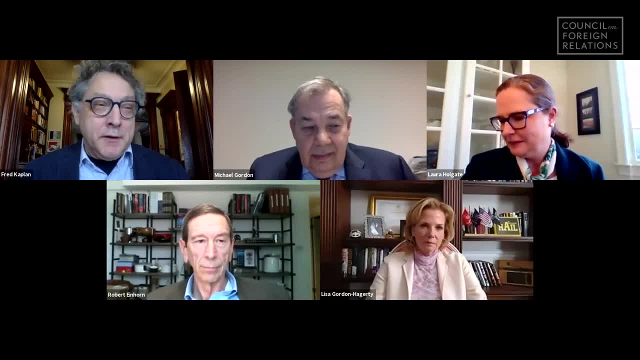 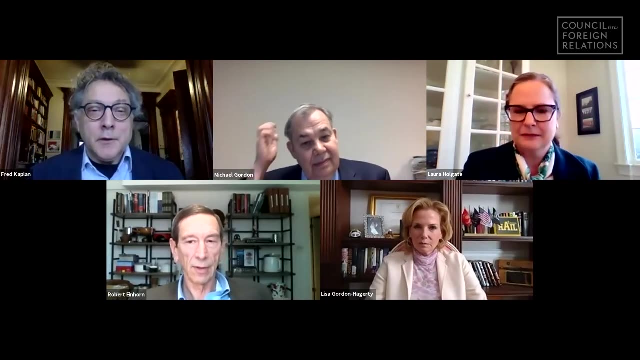 But yeah, again, if you do face these matters bluntly and frankly, you could get into even more trouble. So that's part of the paradox of the whole enterprise. Does anyone want to answer the second question? Which one was that The one no one answered? 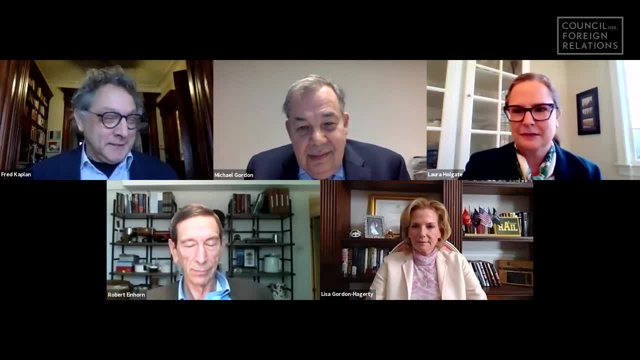 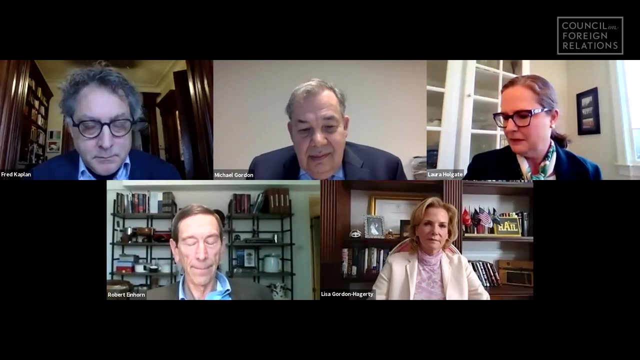 And that is: would you advise the Biden administration to do what the Trump administration did, which was sign an agreement that we will continue to make it actually illegal for any official to say that they have nuclear weapons and not to raise the question of their force publicly at any time? 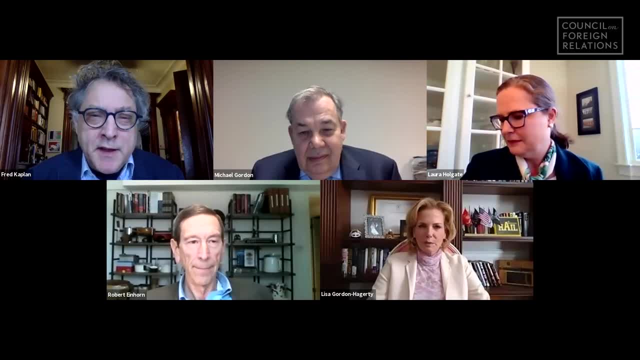 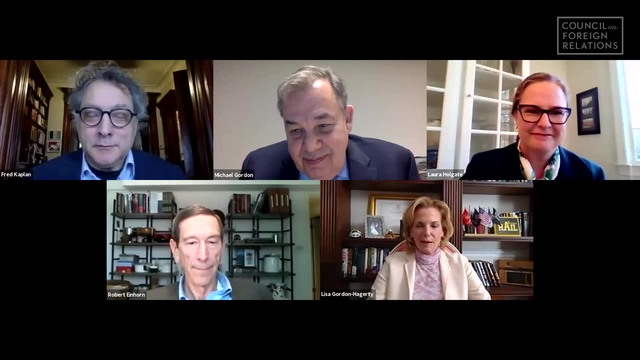 Simple question: Is it illegal for a US official to say that By regulation, it is. yes, Laura and Lisa, do you have any thoughts on this? before we wind up, I guess I would say that I agree with Bob and Fred's analysis. 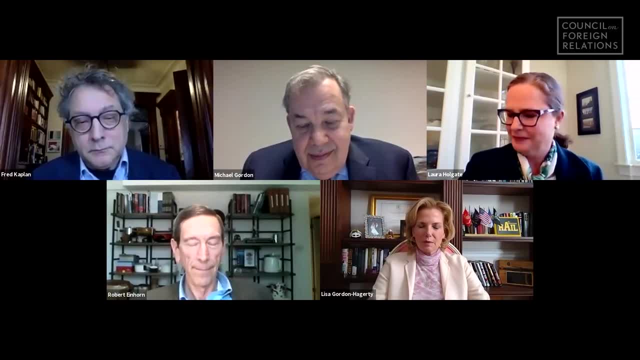 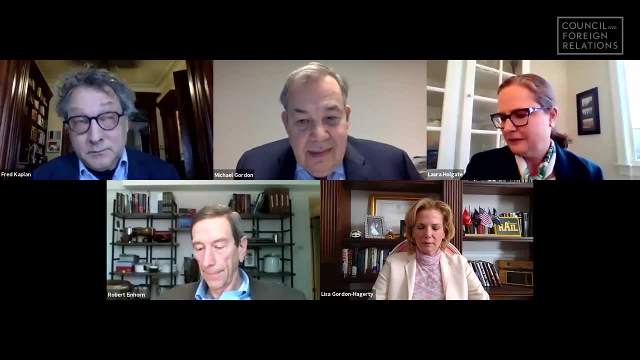 that there are some things that are. perhaps there's a political aspect of it and I don't think that there's any use in moving forward in acknowledging Israel's whether or not their alleged nuclear weapons, whether their nuclear weapons are in the United States. 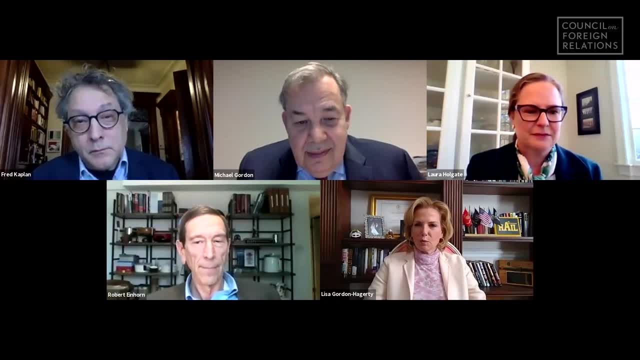 So I'm with Fred and Bob on this point. So I'm not sure what that would do and whether or not we're going to require officials to sign such a policy or adhere to such a policy. So I'm not quite sure, Sometimes leaving well enough alone. 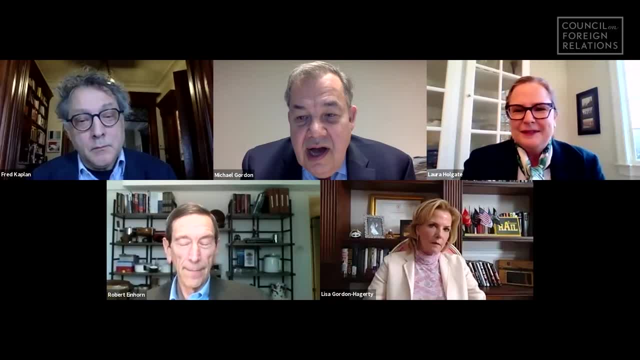 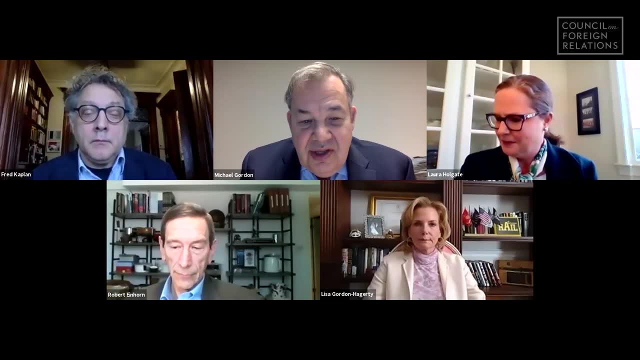 is probably good enough in this sphere. So it's 12 o'clock and we've sort of come to the end of this wide ranging and provocative discussion, And so you know, I'd like to thank everyone who participated in this, and Bob Einhorn and Lisa Gordon-Haggerty. 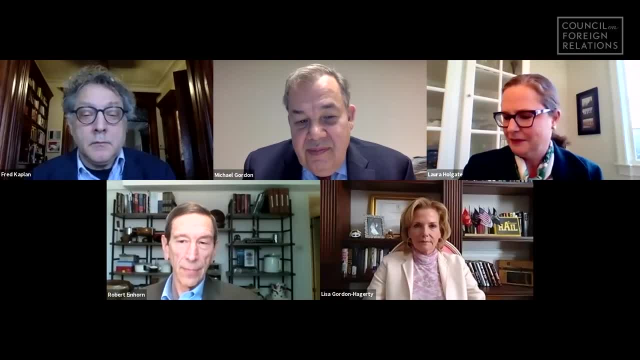 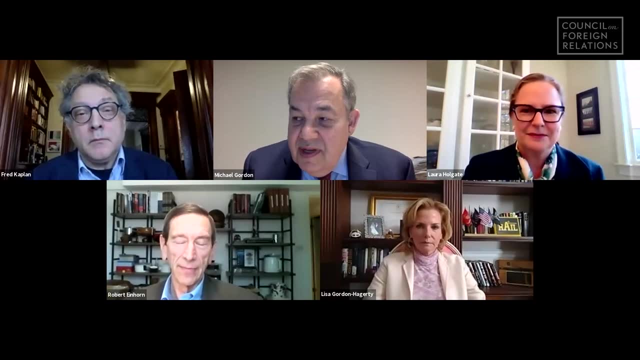 Laura Holgate and Fred Kaplan, And his book again is called The Bomb, And this video and transcript of this meeting is going to be posted on the CFR website so you'll be able to go back to it. So thank you for participating in the event.